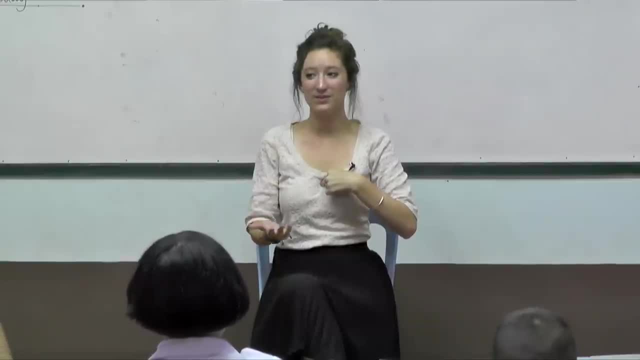 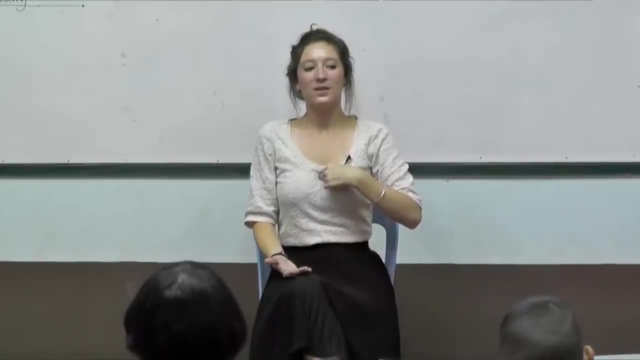 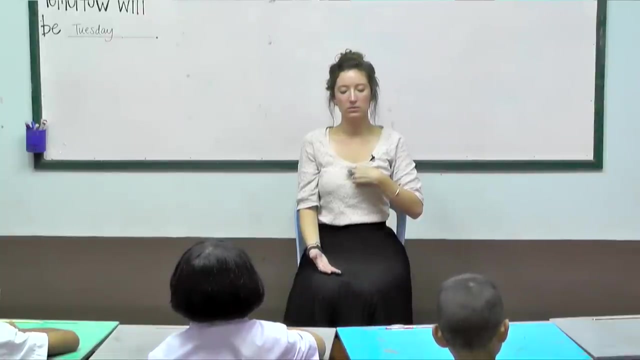 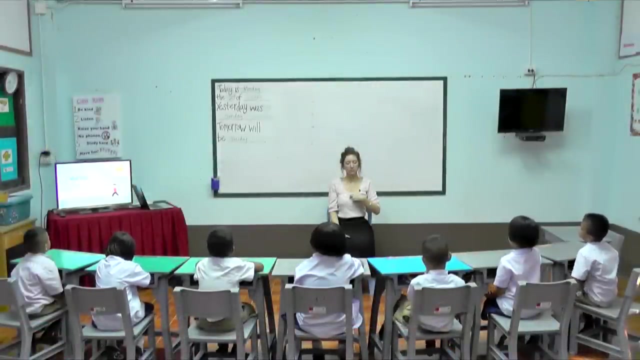 Or your pulse. We'll take our other hand open, Lay it in our laps, Take a deep breath, Close your eyes And let's meditate together for a minute. There we go. 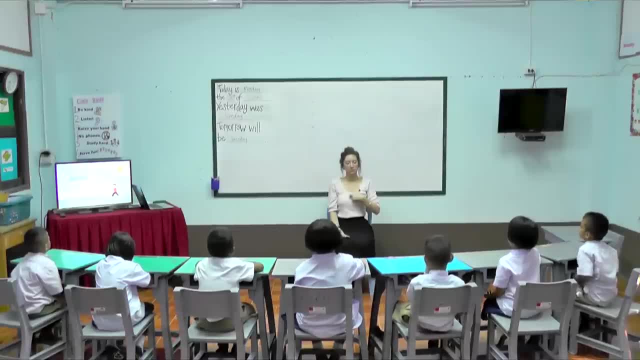 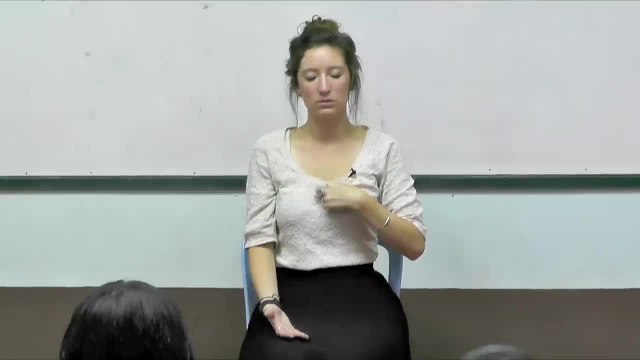 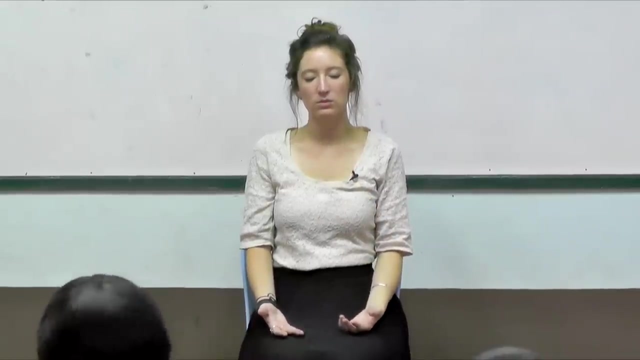 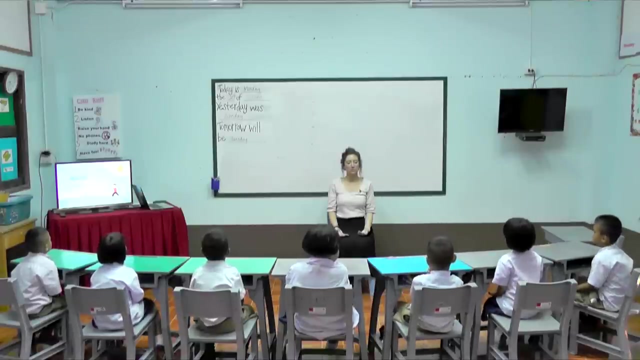 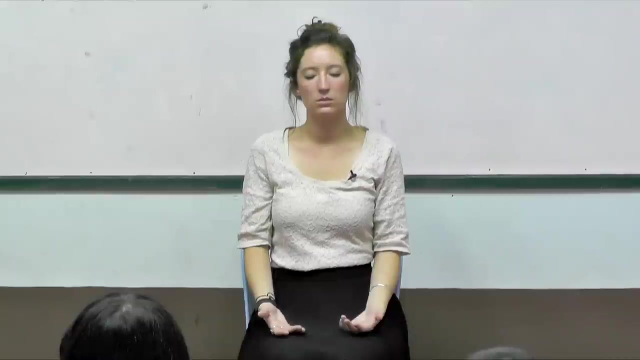 Remember, once we're able to feel with our fingers, we can go ahead and lay both hands down, palms open, Continue to focus, stay around your heart center, Feel the energy here. Thank you. 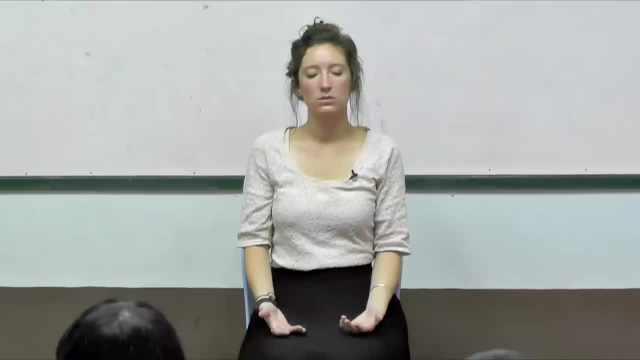 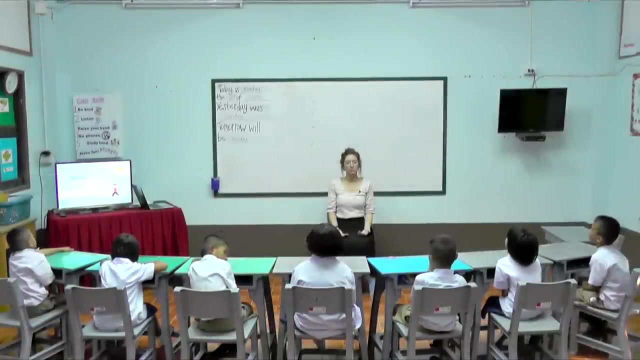 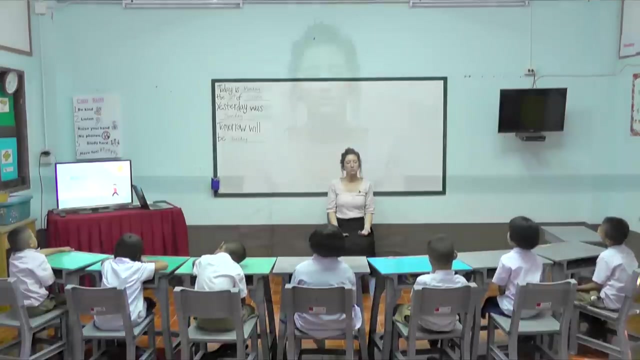 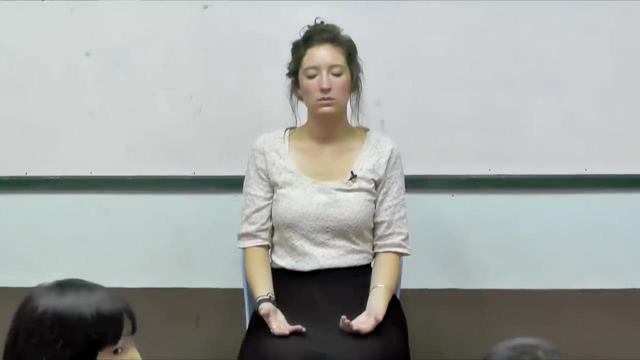 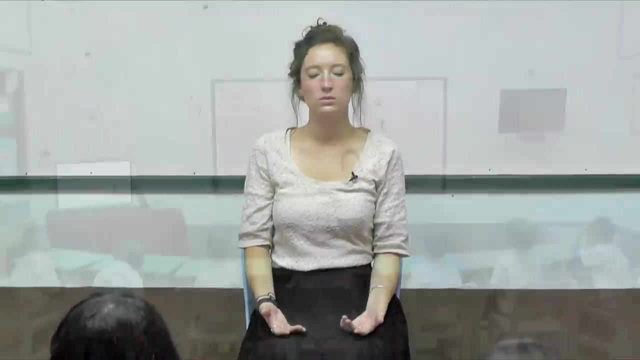 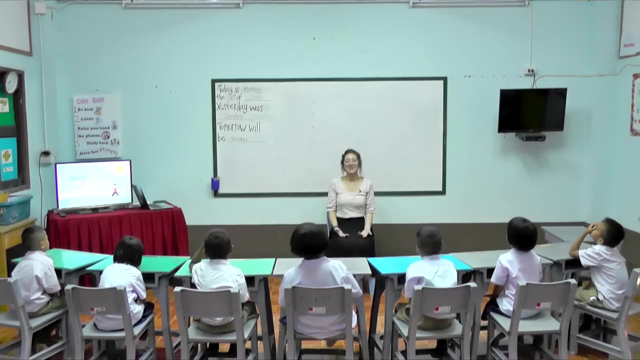 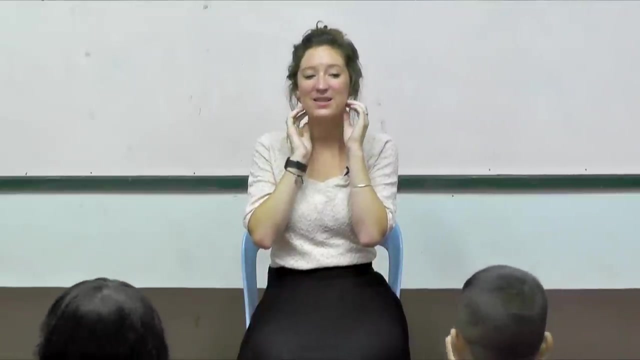 Thank you. Feel the energy in your heart center. Stay focused, Stay focused. Okay, Great job, Great job. Great job everybody. We'll come out of meditation together. We'll slowly open our eyes and take three deep breaths. 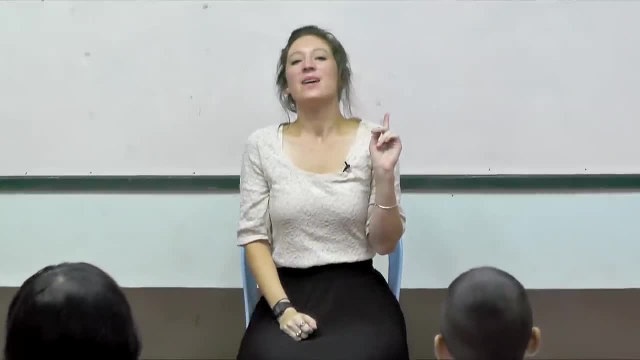 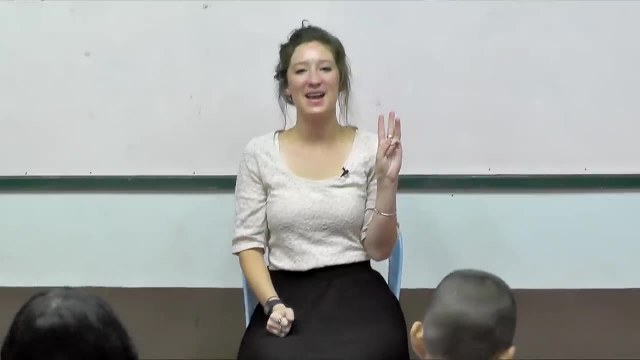 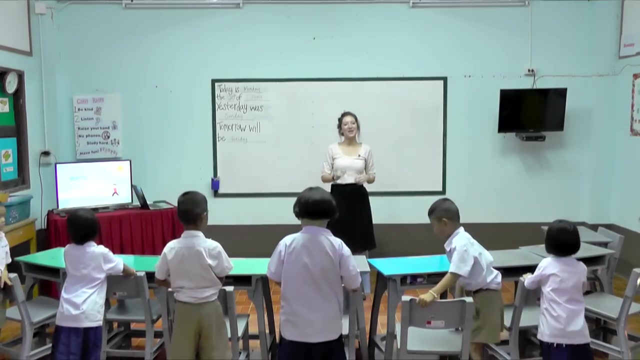 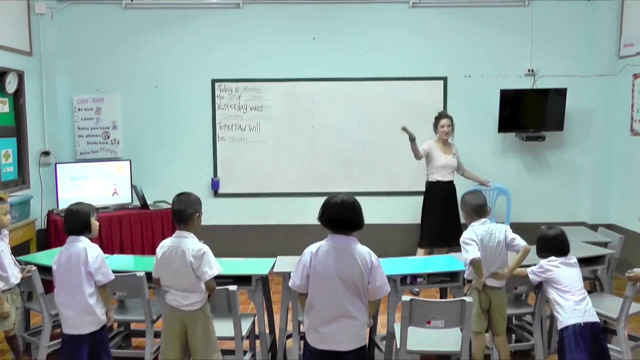 Ready. One, Two Breathe with me And three. Great job, We'll take a stand, please. I like to begin our classes with a little bit of physical warm-up after meditation. So everyone stand up and together first. 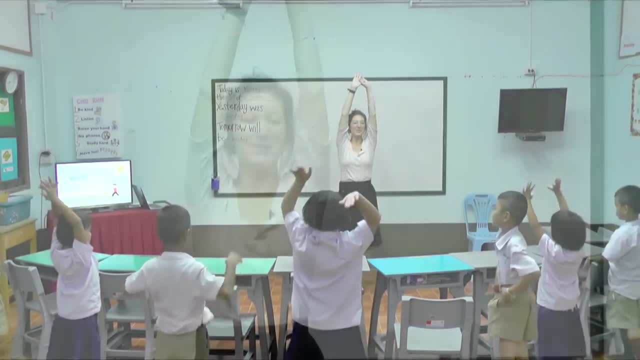 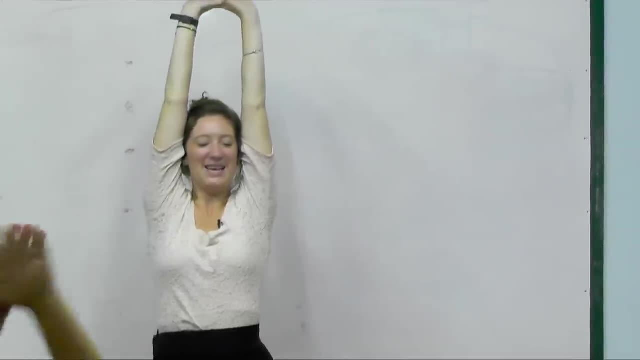 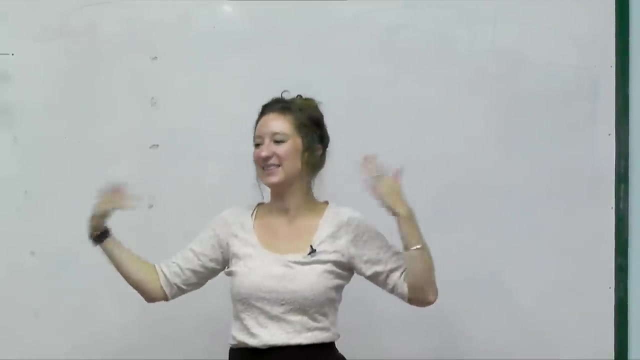 we will stretch up, oh, stretch up to the sky, Stretch with me. Oh, it feels so good. And then we shake it out, Shake it out, Loosen up our bodies and shake it out, Yeah. And then we stretch it down to our toes. 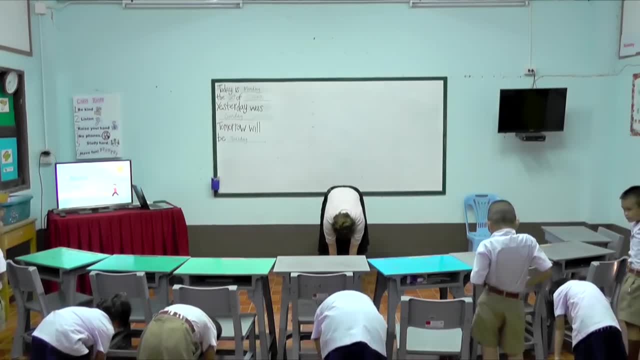 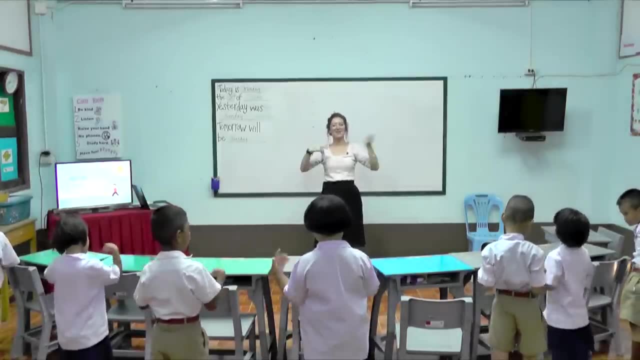 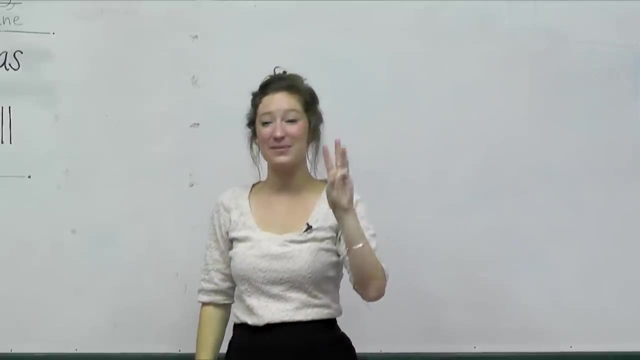 Come on, Stretch with me, Stretch And we Shake it out. Shake it out, Good job, Shake it out. Now we're going to spin around. How many times? Three? We like to spin three times. Do it with us. 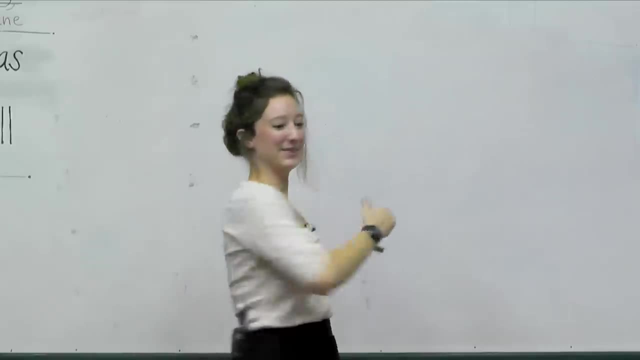 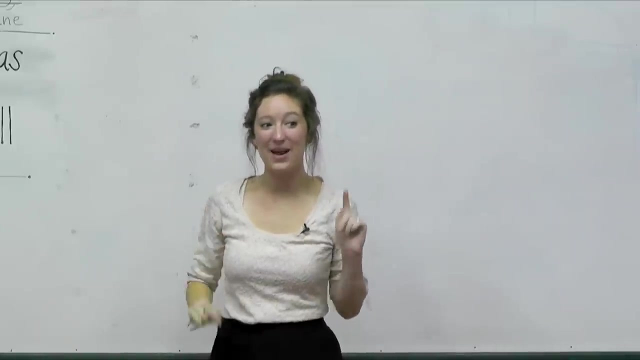 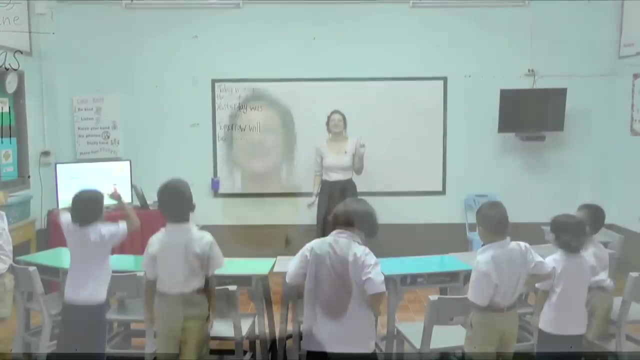 One, Two, Two, Three. And then we like to jump up and down. How many times? One, Two, Three. And then we like to jump up and down times. Three times One, two, three. Great job, everybody. You can have a seat now. 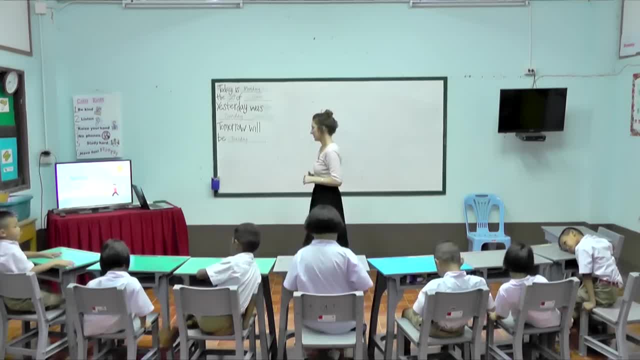 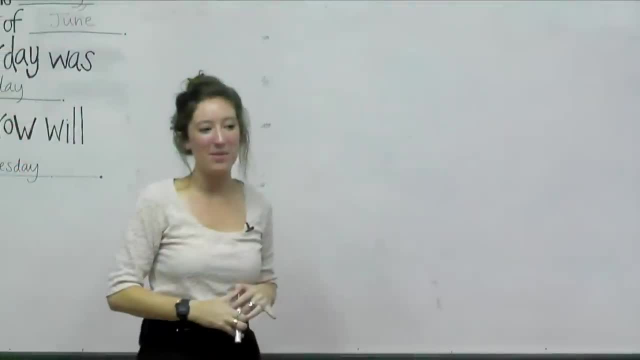 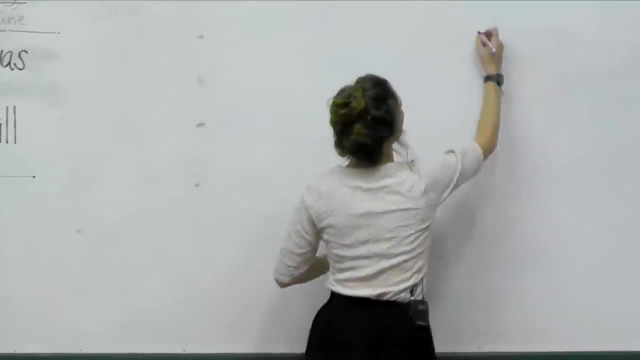 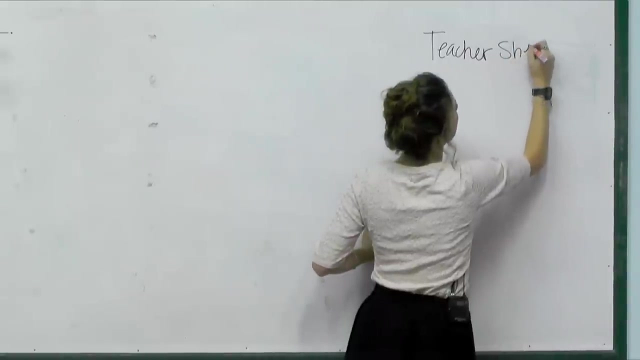 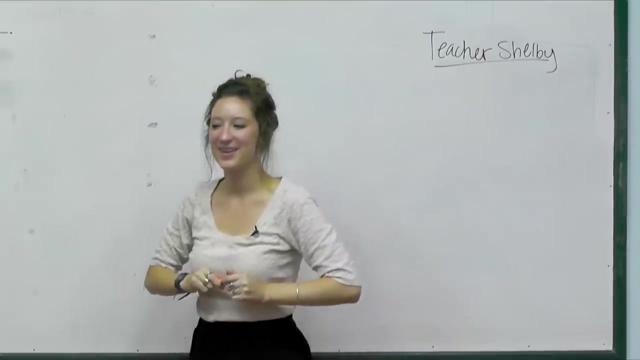 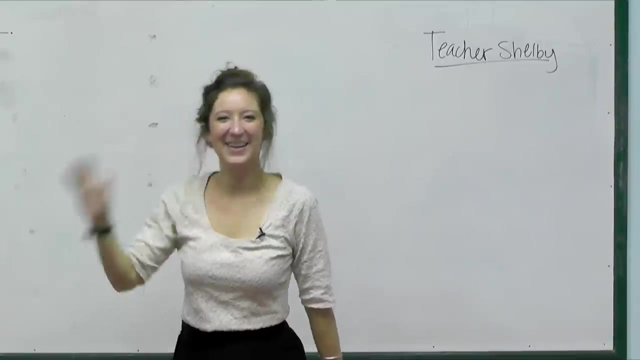 Sit down in our chairs, Awesome. So today, for our first math lesson, we are going to talk about numbers, Numbers, Yeah, So I'll go ahead. since it's our first lesson, I'll write my name: Teacher Shelby, Teacher Shelby, Teacher Shelby. Very good, Nice to meet you all. 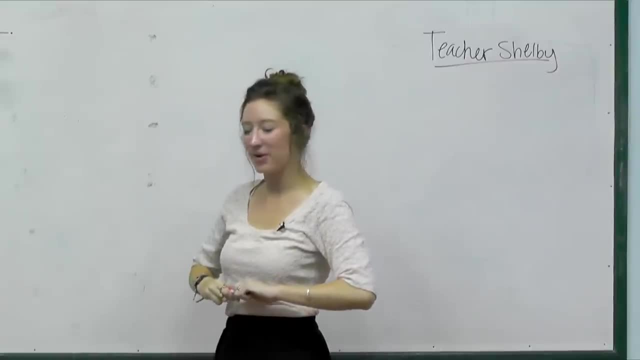 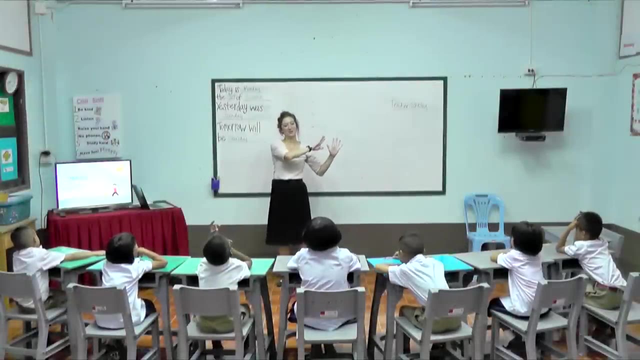 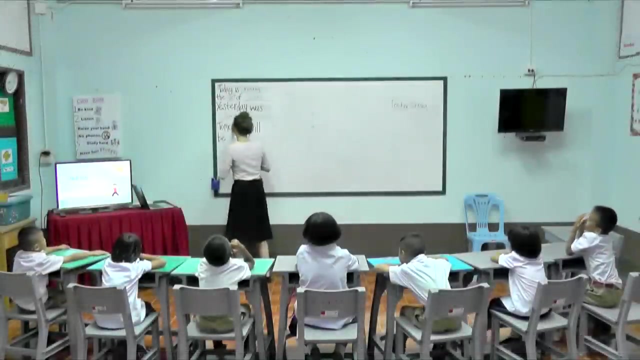 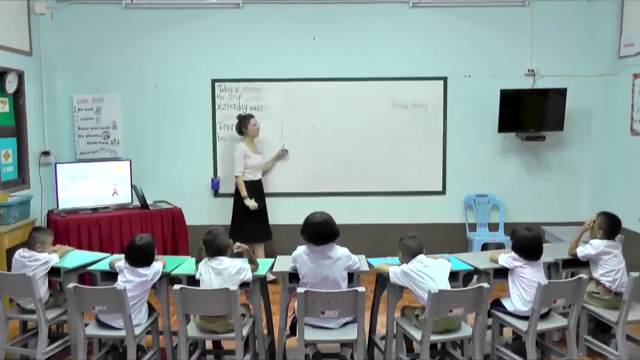 I'm teacher Shelby, So let's get back to our numbers. We're gonna talk about the numbers one all the way to ten, right, And then we're going to count things, Yeah, So first let's talk about how we write them. Yeah, What number is this One? It's the number one, So let's talk. 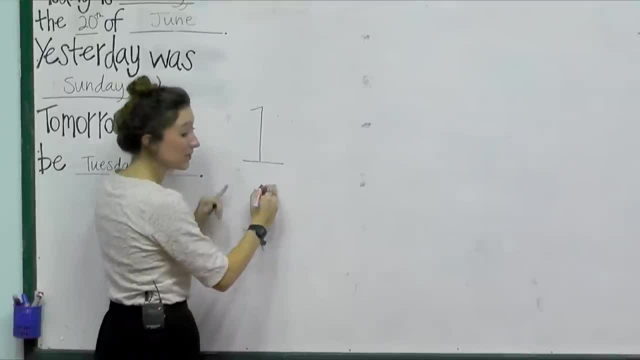 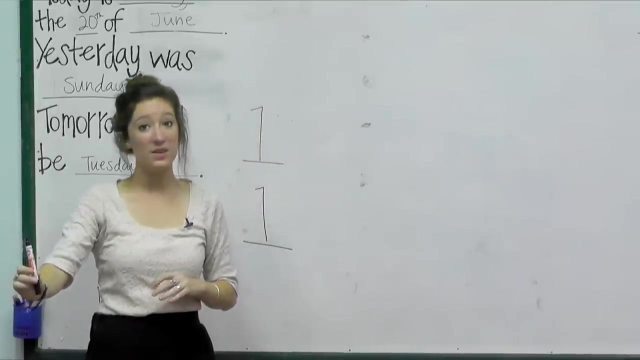 about how we write the number one. Let's look at one. first We go up, right Down And then across. That's how we write one. Yeah, That's how we write one. Does someone want to come show me how they write one? Yeah, Come show me. We want to make sure that we're writing our numbers correctly. 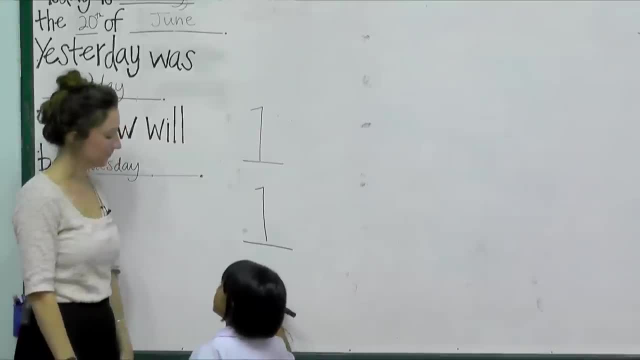 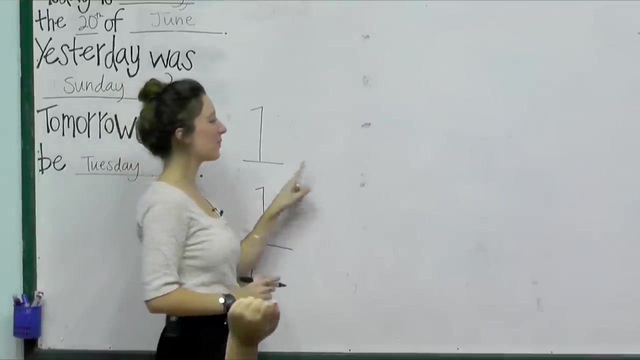 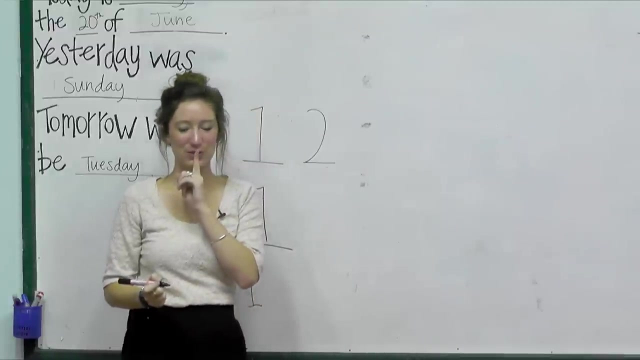 Write one for me. One, One, One, One. That's perfect, Thank you, Good job. And so who knows what comes after one? Two, That's right. Two comes next Two. How about? we'll just go in order, We'll. 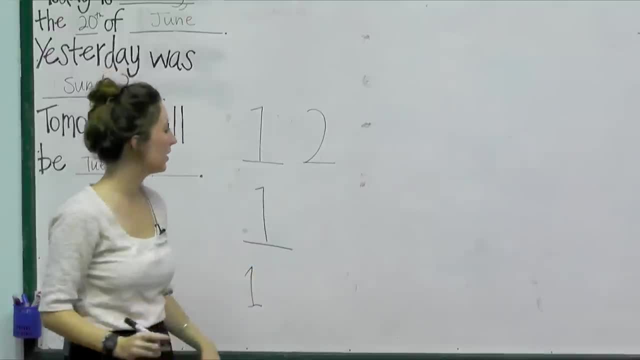 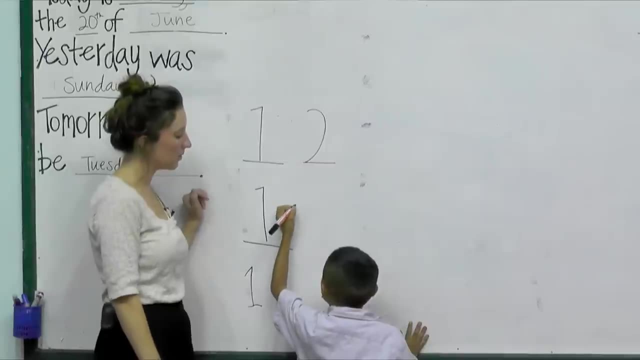 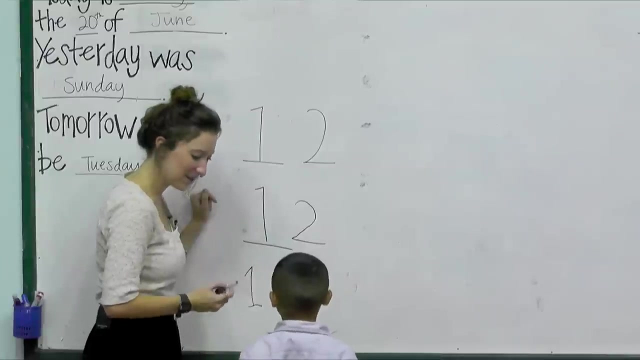 start with two, and then we'll go in order this way: Okay, Two, Two, right. So we want to make sure that we're writing two correctly. That's perfect, That's very good, Thank you. And so you may notice, some people write two like this: 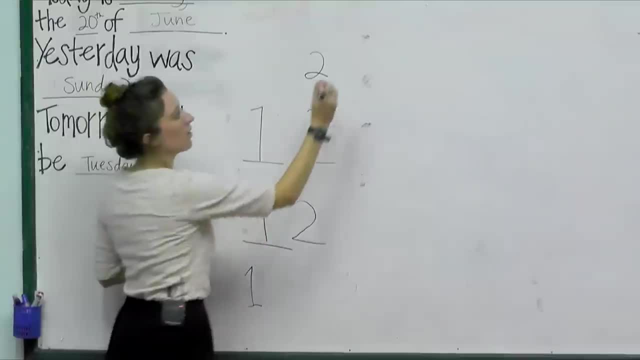 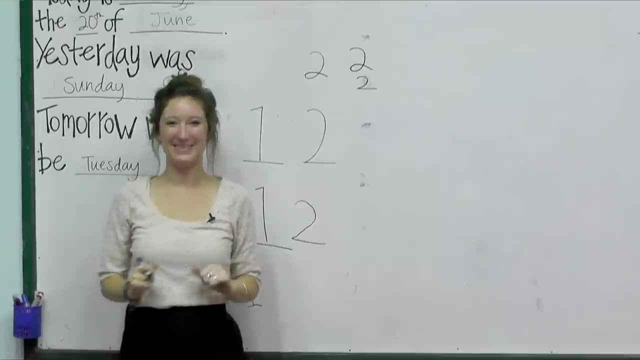 That's okay too. We can do that. We can make a loop like this, or we can make a stop. We can make a loop like this. We can make a loop like this, We can make a stop. We can make a straight like this. Yes, Okay, Either way. Either way is fine, Whatever is easiest for your hand. 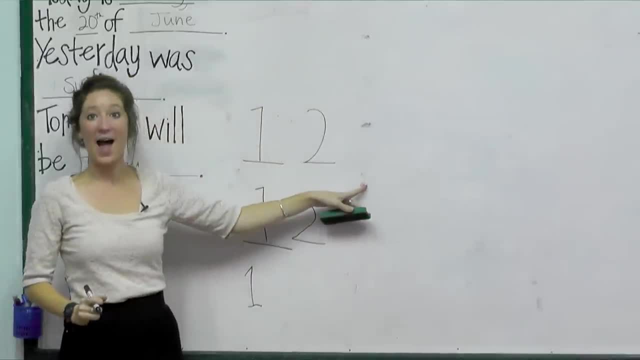 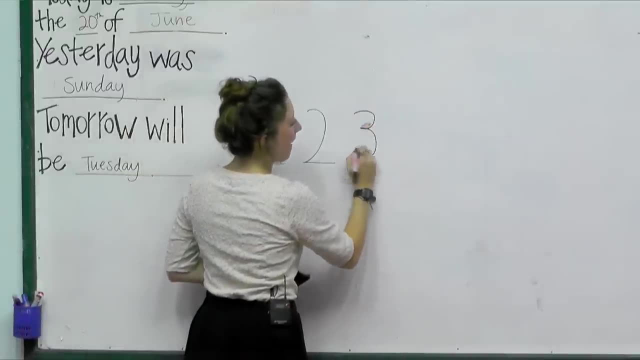 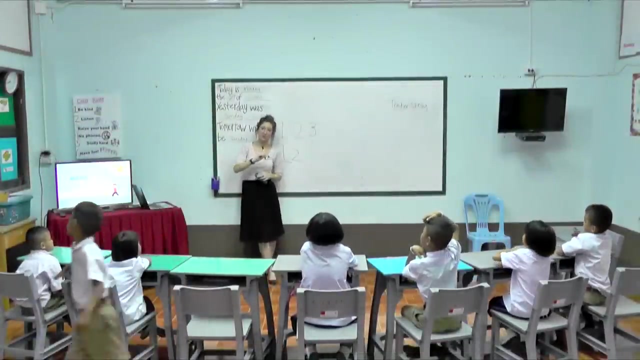 So what comes after two, Three, Three, That's right. Three is next. So for a three, we make a bump, Bump, Just like that. Who knows how to write a three? All right, Pot, come show us how you write a number three. 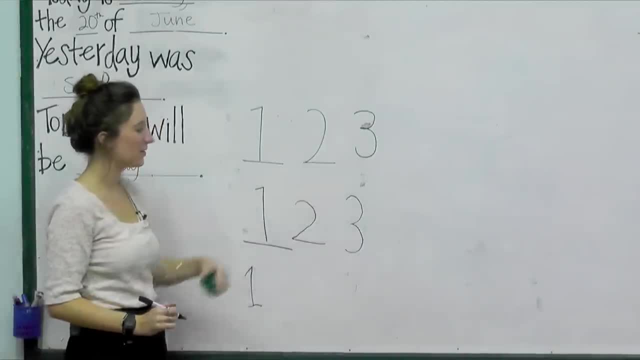 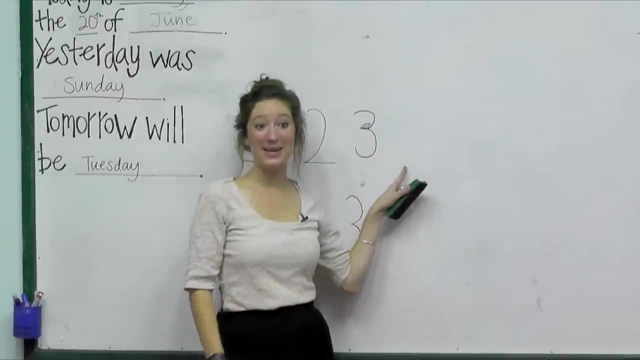 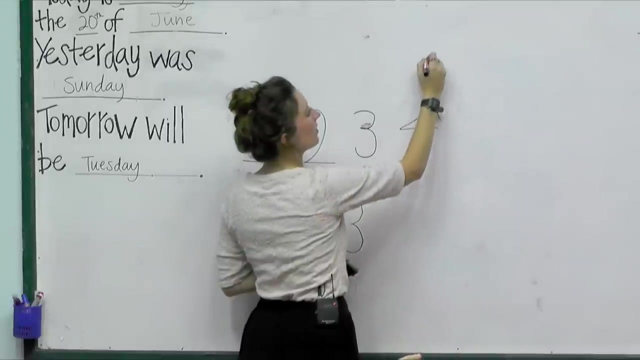 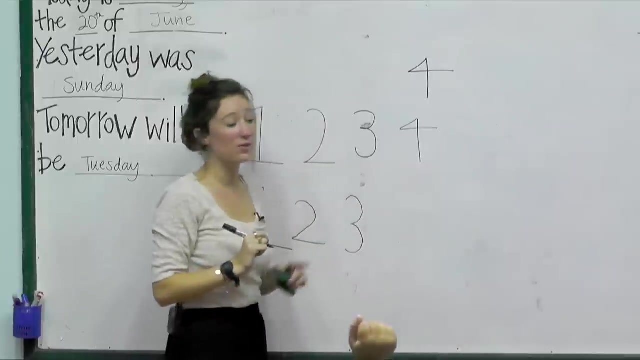 Very good, Perfect, everybody. So here's what a three looks like, And after three, the number four. Here's how we write the number four: Right, We go down, across down. And four is another one We can also write it. 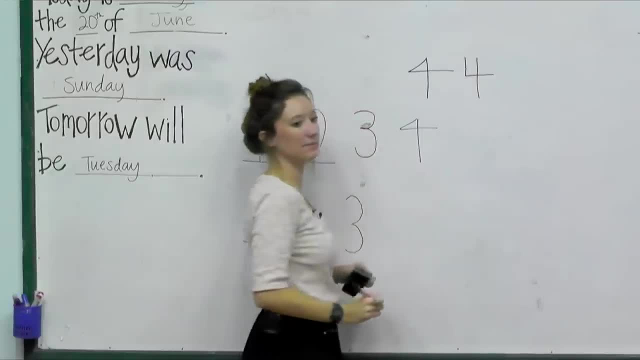 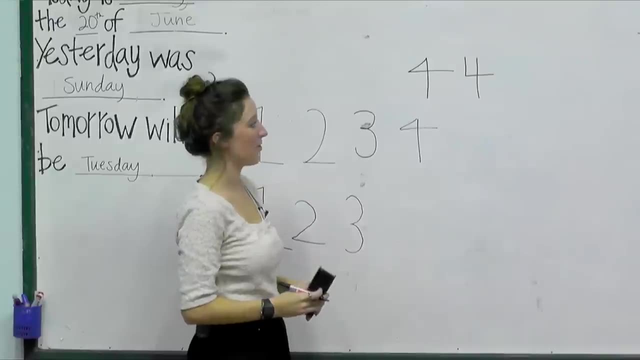 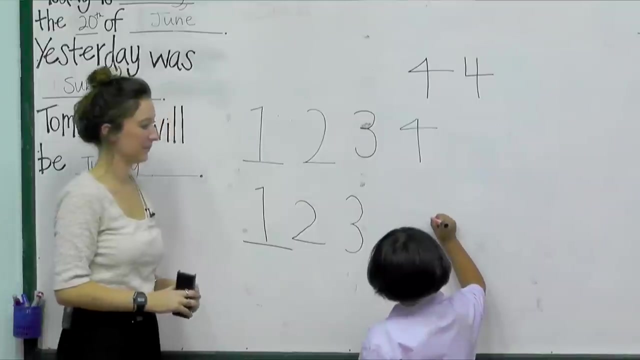 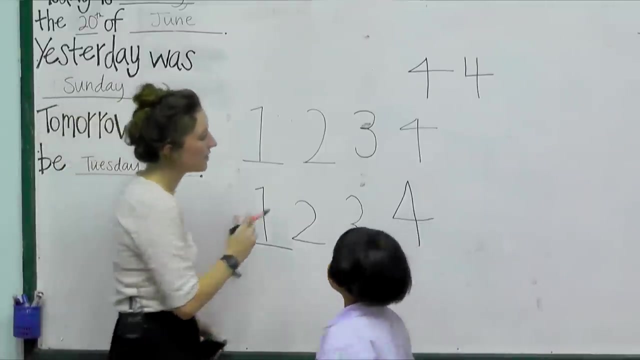 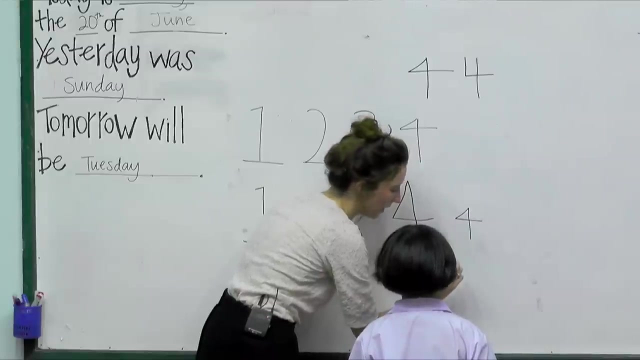 like this. This is also okay. Whatever is easiest for you. These are both four Same, Okay, So who wants to show me their four? Let go, Let go, Let go, That works, That works. Is it easier, though, for you to go like? will you try it that way instead of? 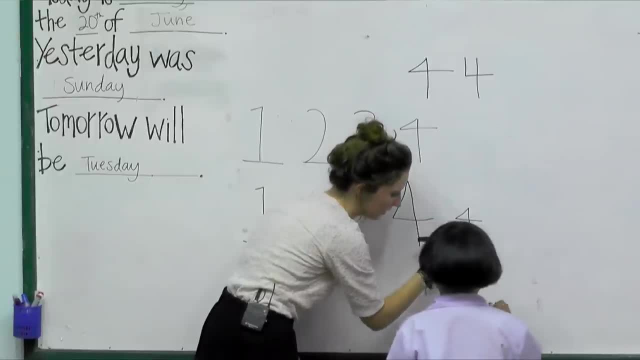 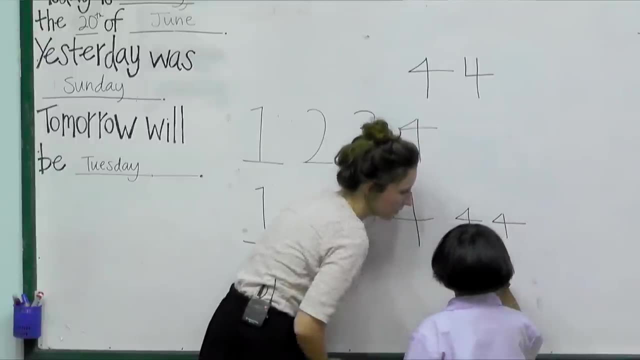 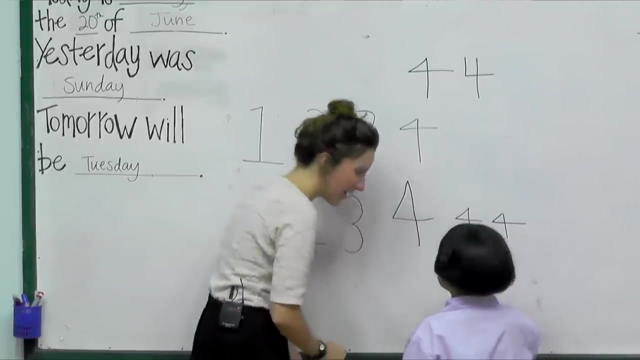 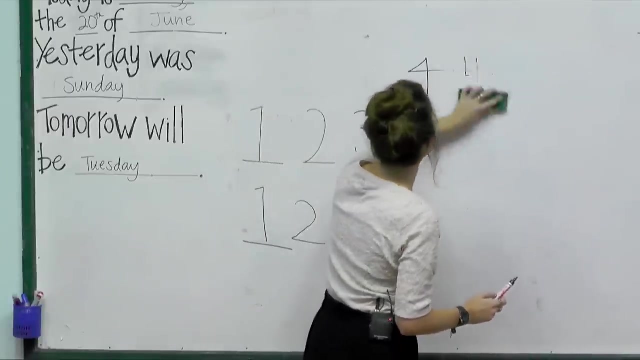 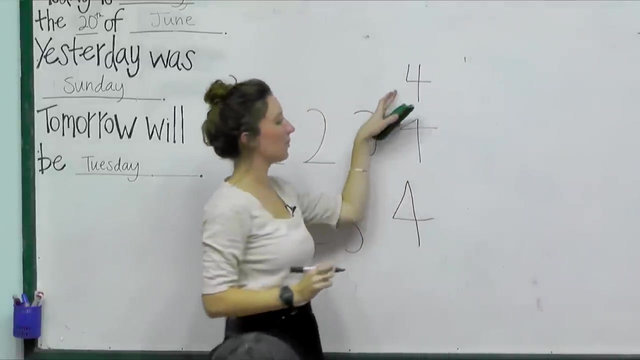 No, Yeah, Let's try it this way, See if it's easier. Try to go over and then down, Okay, Mm-hmm, Yeah, perfect, That was very good. I'll put this here too, just as an example. These are both correct. 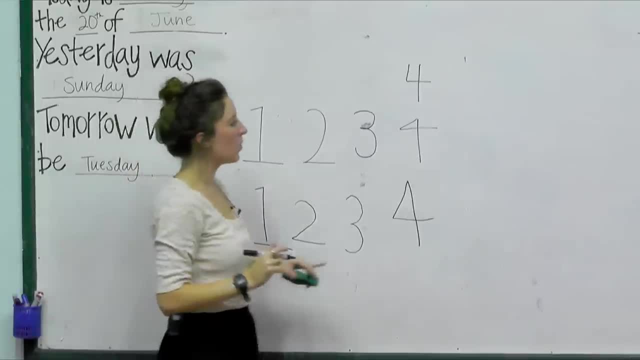 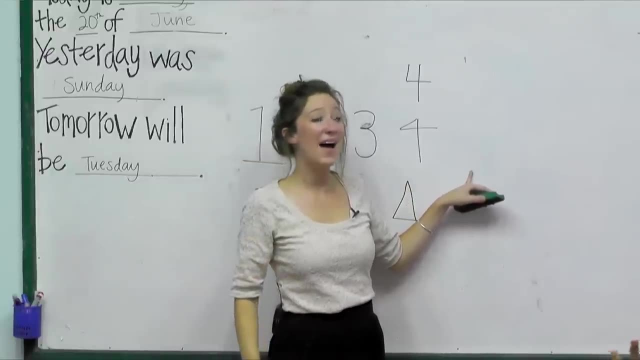 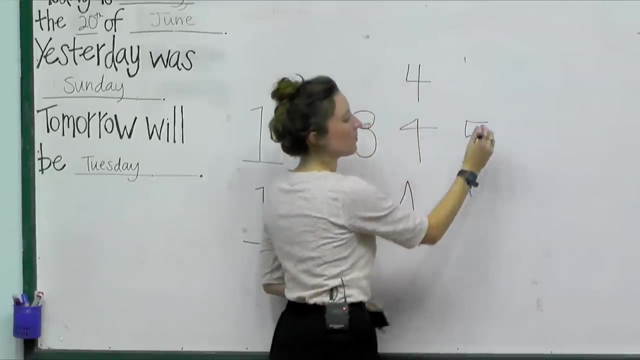 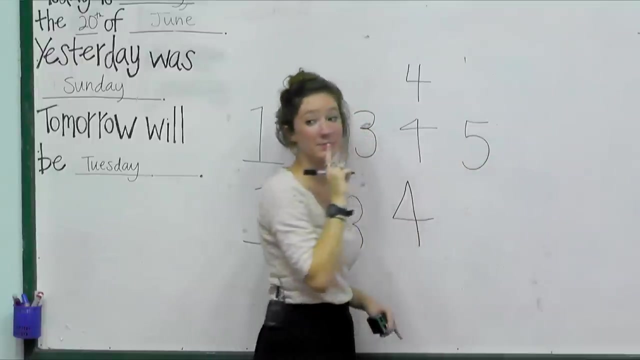 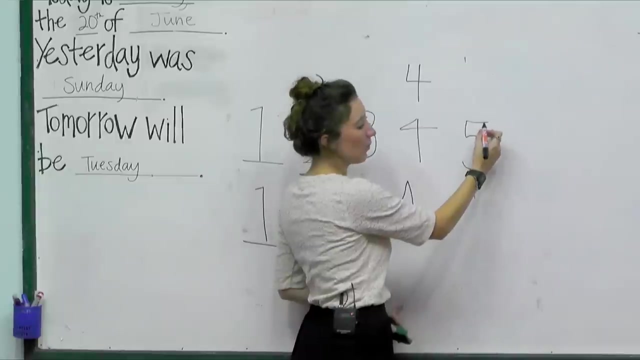 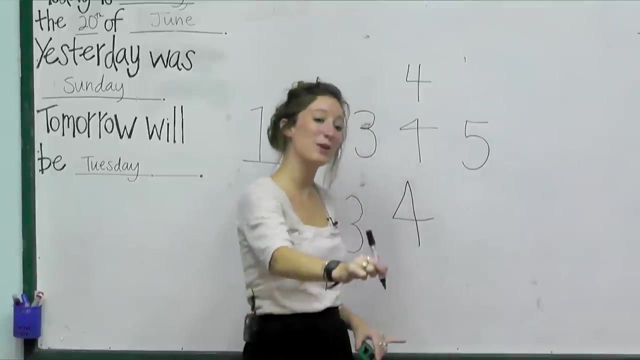 So what number comes after four? Do we remember? Do we know? Five, Five, Five, Five comes next, Five, five is next, remember? so we write our five across down and around five. no, I know, I know I got it, don't worry, so with five here one more time: across down and around. okay, come show me how you write a. 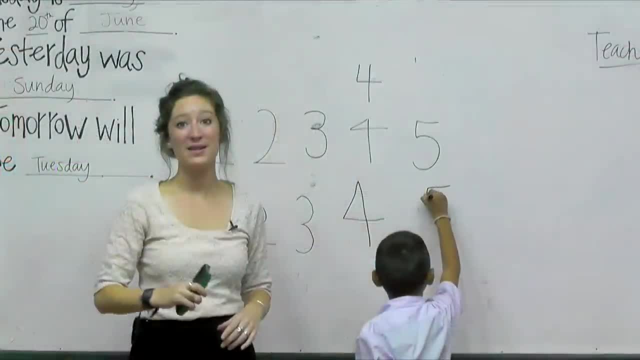 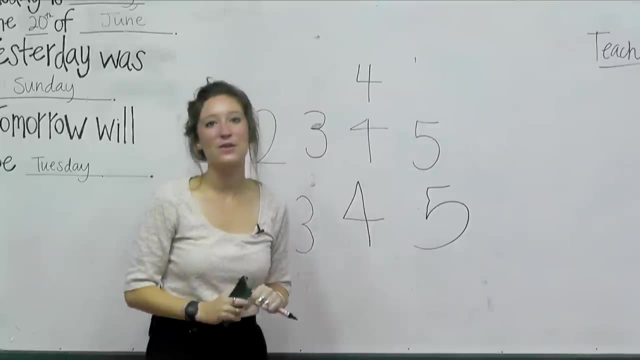 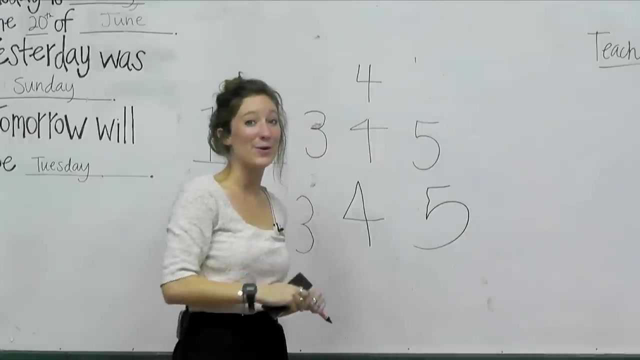 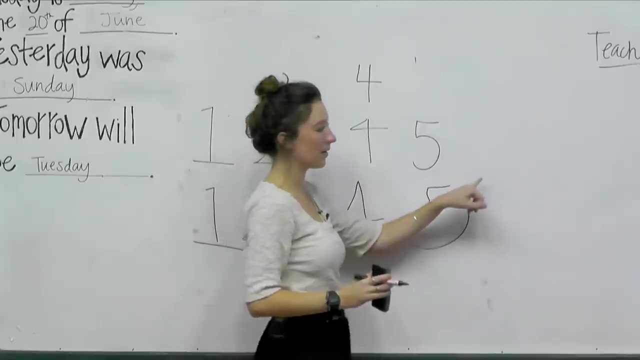 five, five for our friends watching this is a great practice, very good, very good, great practice for you guys to watch us go through numbers. if you have the ability and are able to practice along with us on your own whiteboard, even better. okay. so what's after five? what number? six, six is next. 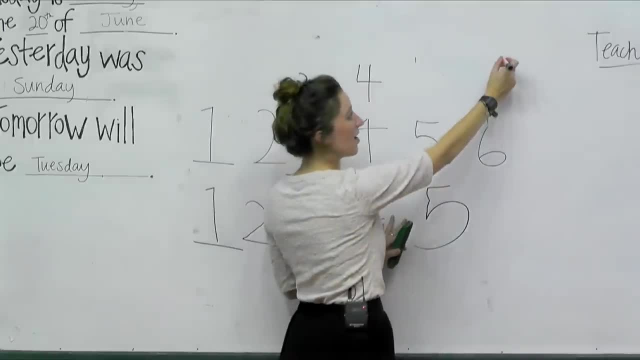 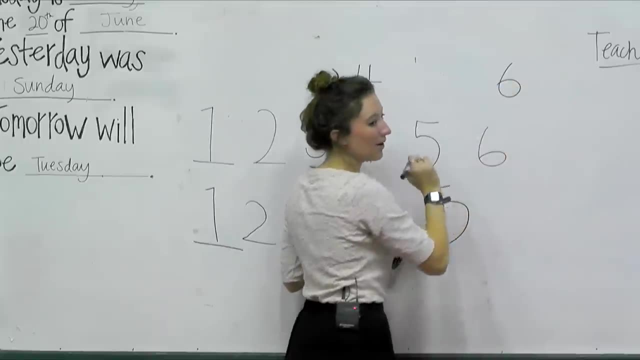 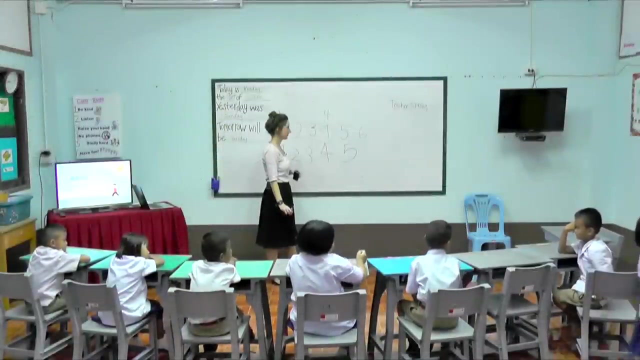 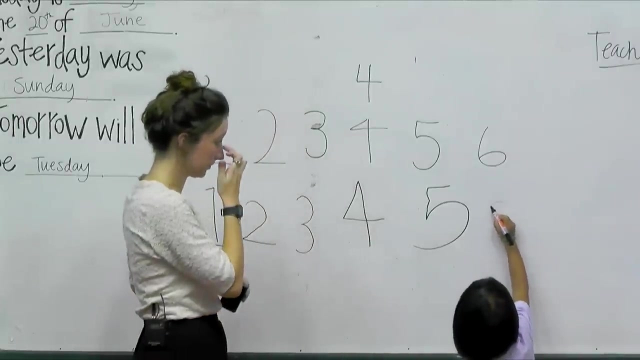 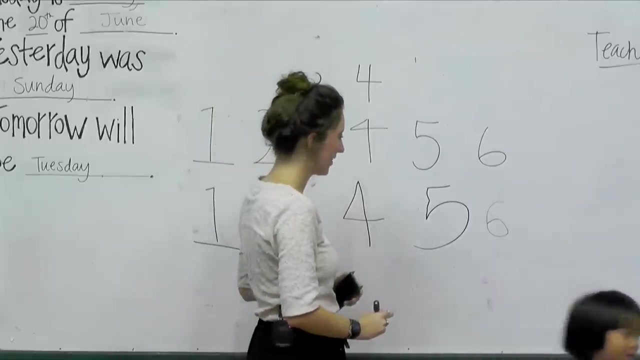 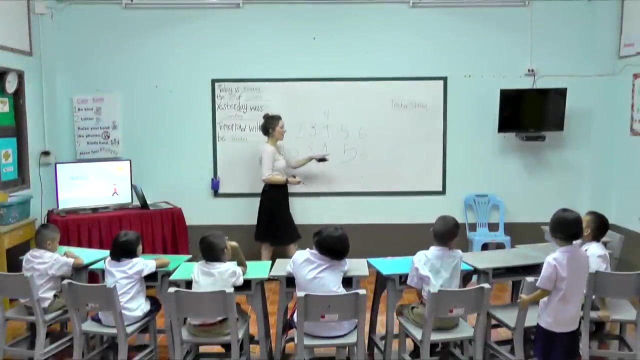 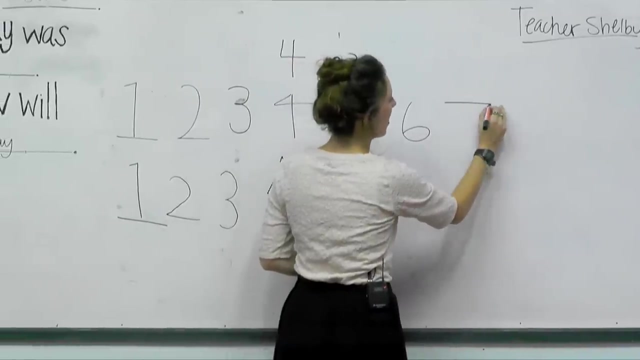 six, we start up and we go around. right, we start up and we go around. okay, show me how you make a six. very good, very good. six, oh, thank you. so who remembers what comes after the number six? seven, seven, that's right, seven comes next. seven, we go across. 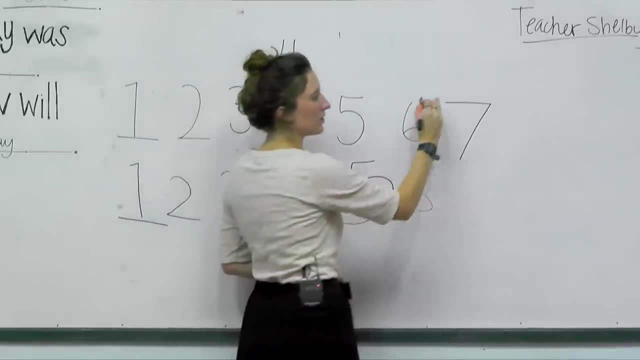 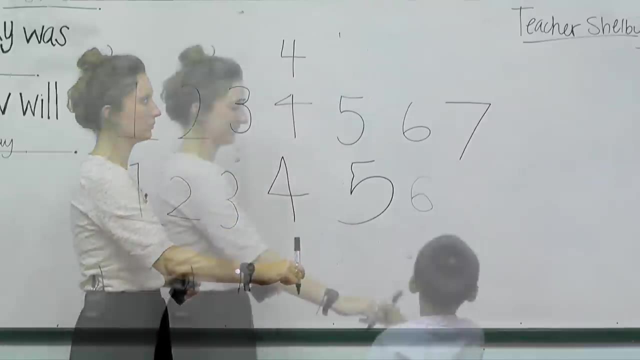 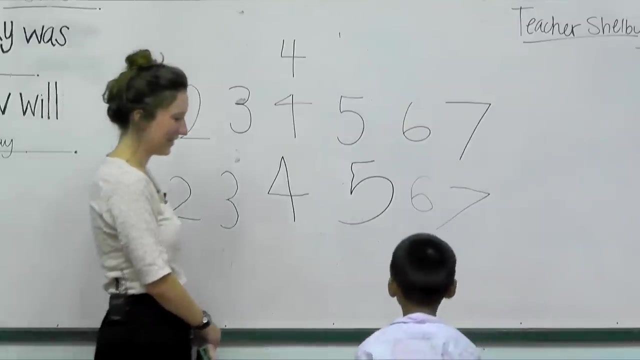 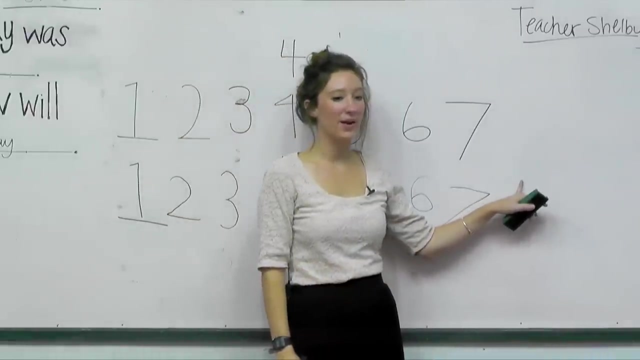 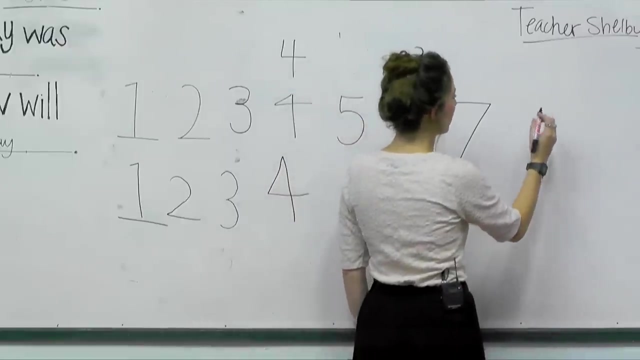 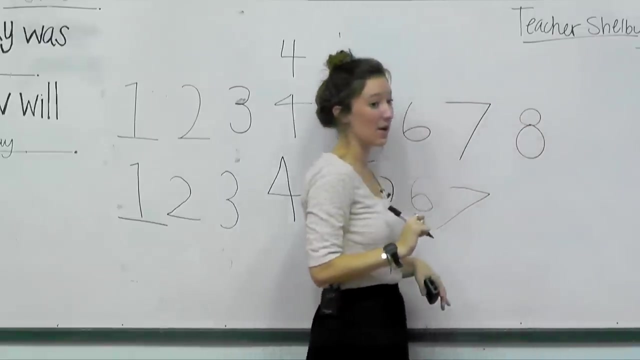 and down. seven's an easy one, just over and down, just like that. will you come, show me your seven? very good, that's very good. seven, great work. who knows what number eight, eight comes after the number seven. eight, eight's another one of those. I draw my eight like this, but. 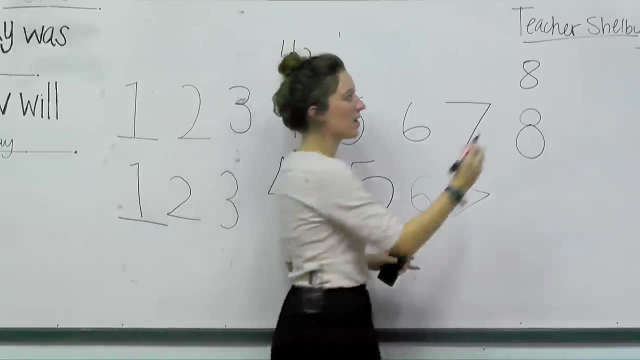 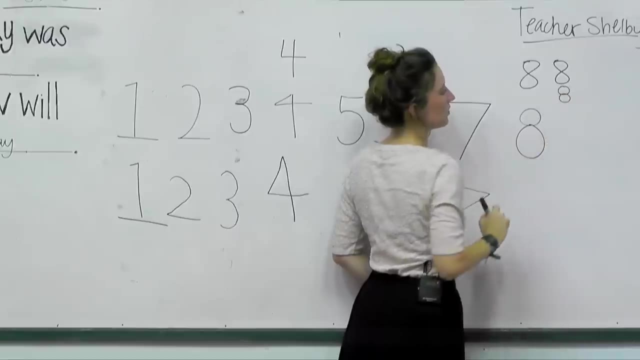 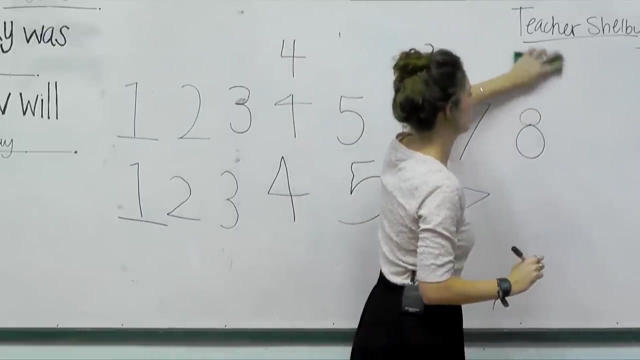 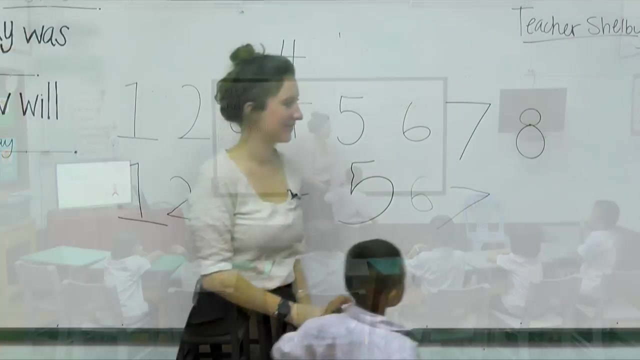 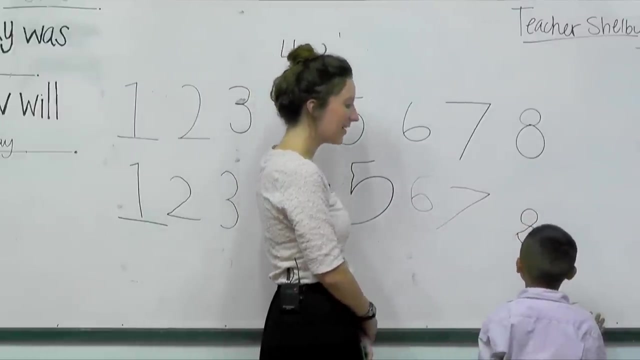 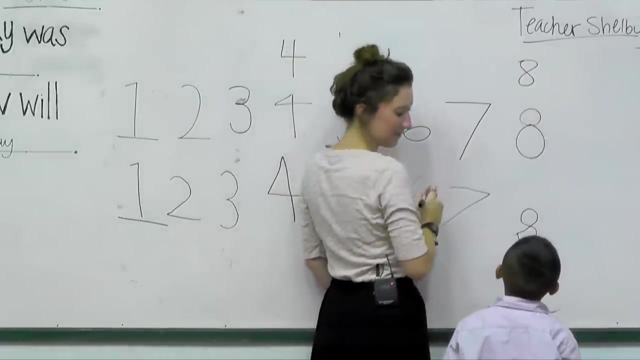 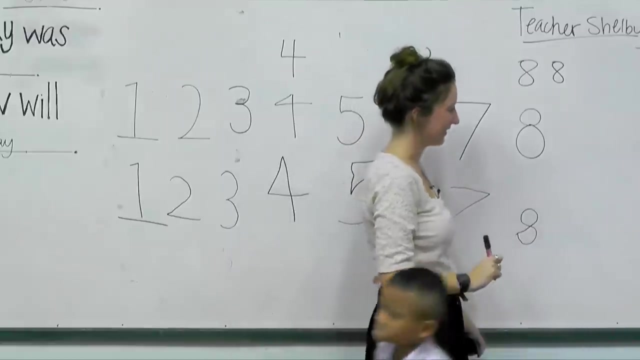 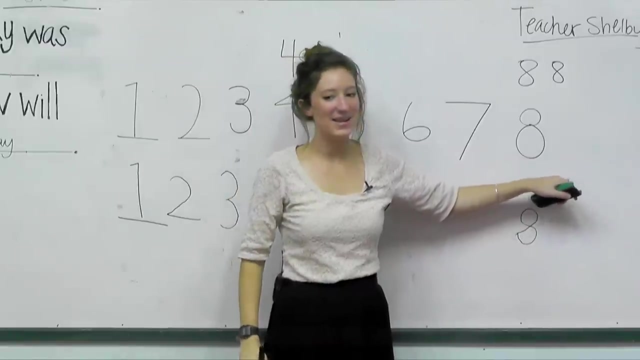 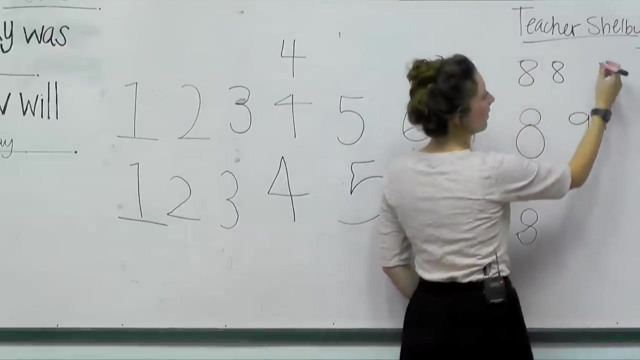 this is okay too. eight both ways, so we can do one movement or we can do two circles. they both, yeah, they both, make an eight. who wants to show me their eight? it's you, show me your eight. It's four. good five. three, four, seven, five. So our nine, right. 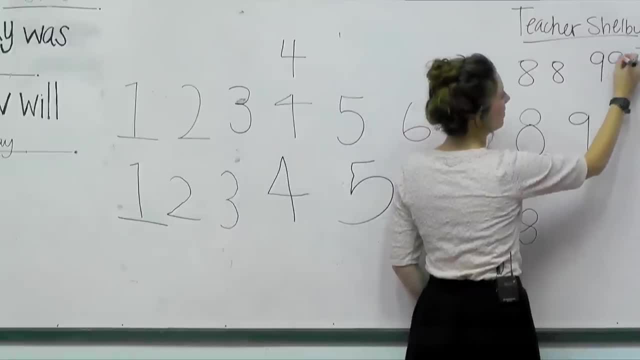 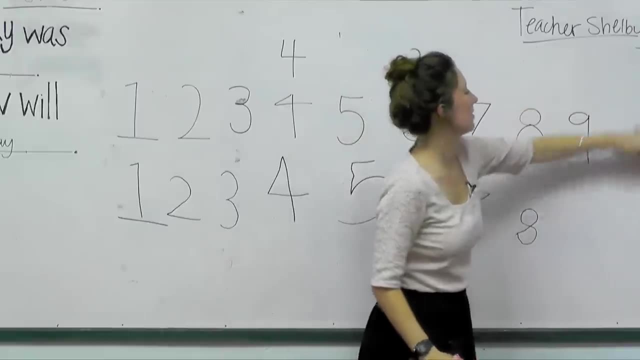 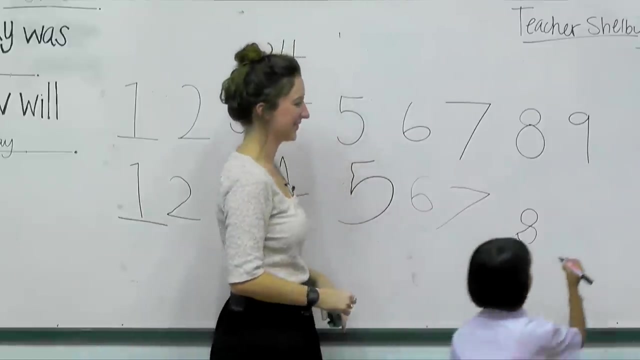 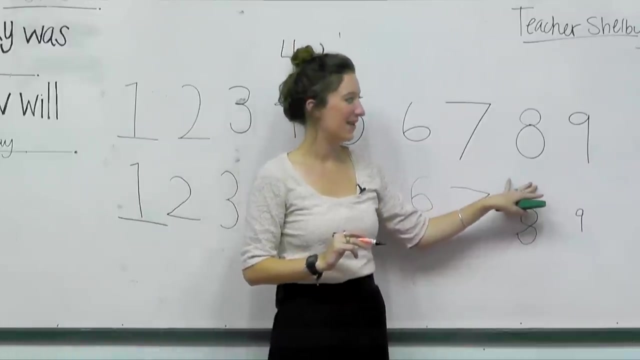 We make a loop and down, loop and down. So who can show me their nine? Very good, very good. Here's an excellent nine. It's nine. I'll leave this above here. So what's our last number? Ten? 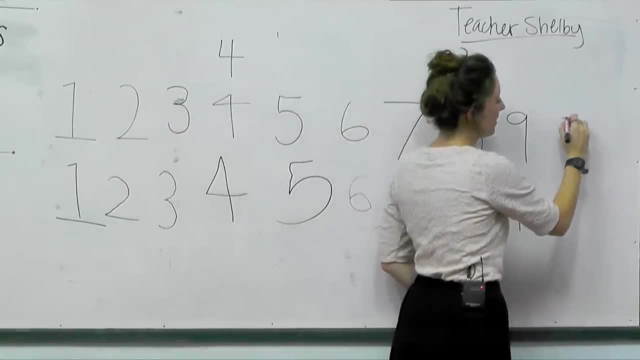 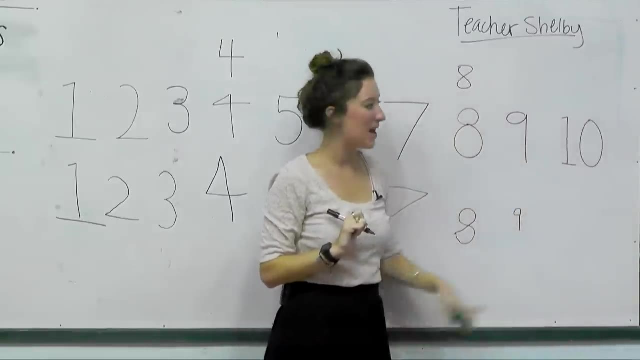 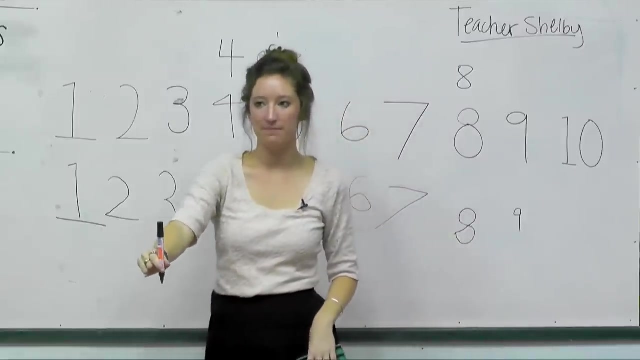 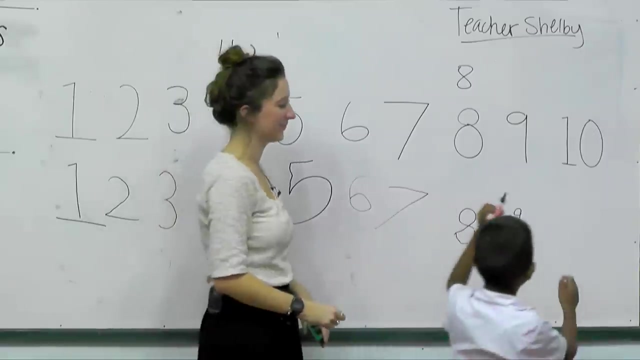 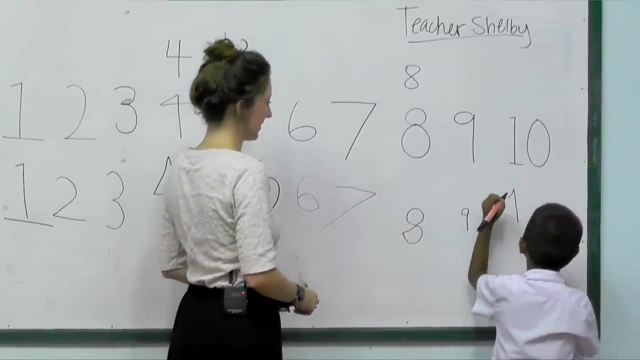 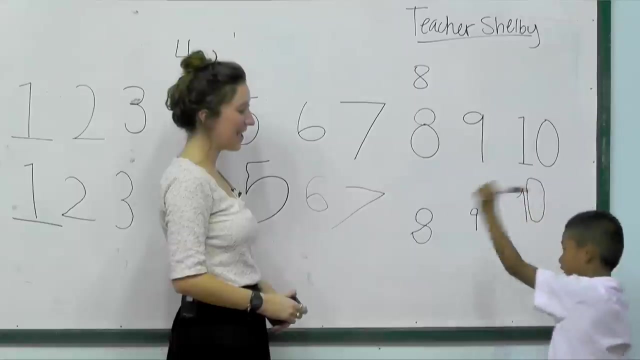 Ten, it's a ten, And we write a ten with a one and zero. right One, zero, ten, Ten. okay, show me how you write ten. Whoa Ten, very good. One and zero Ten, good job. 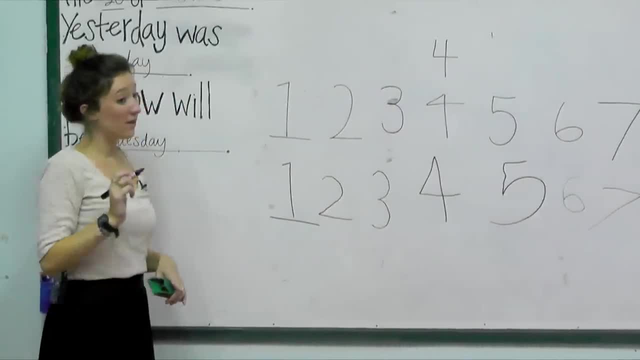 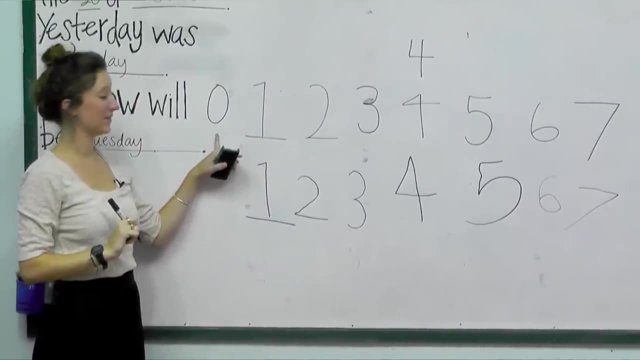 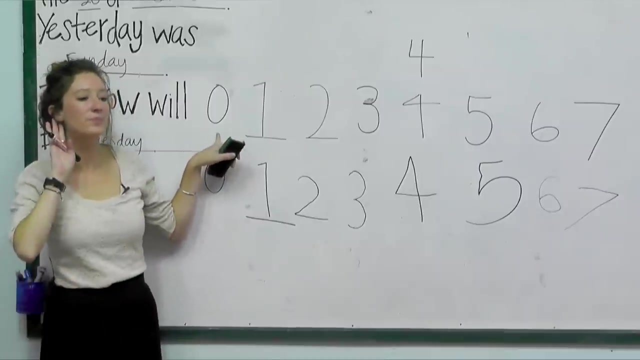 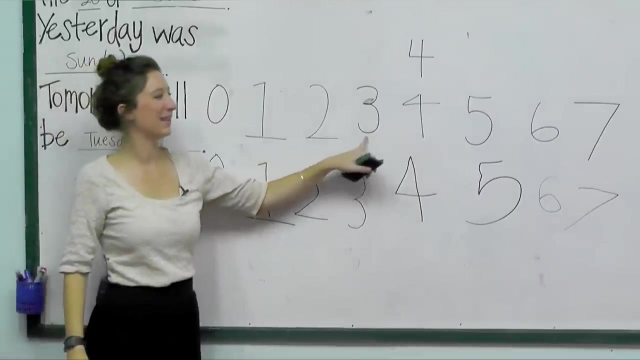 And that reminds me we can't forget about zero. Remember It comes before one. We don't want to forget about zero. Let me hear you say zero, Zero, Zero, Good, good, Zero is before one. Zero One, Two, Three, Four, Five. 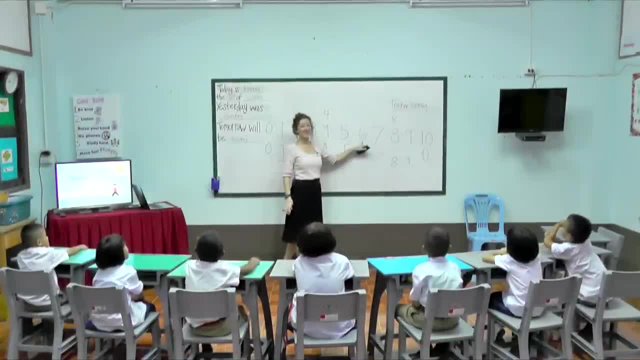 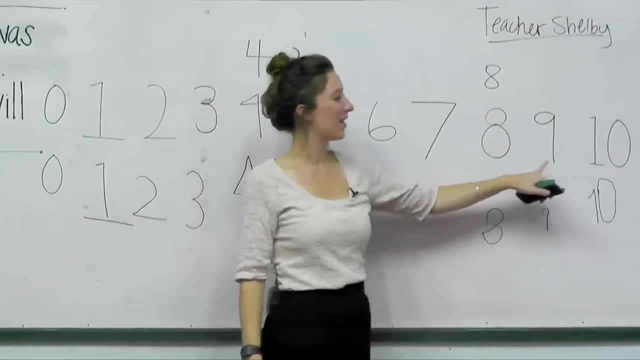 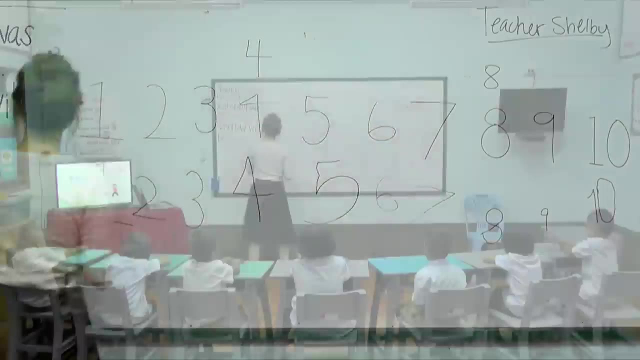 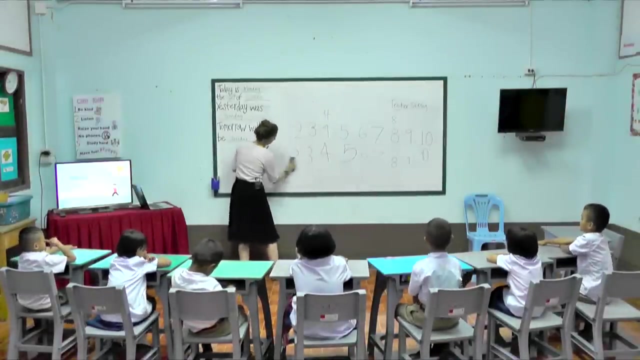 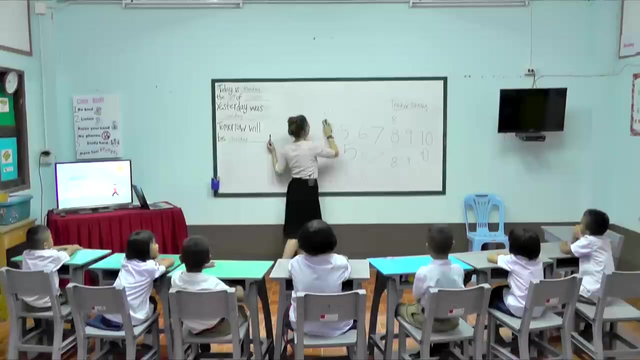 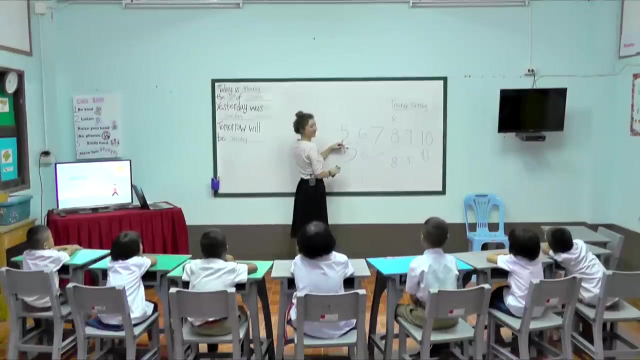 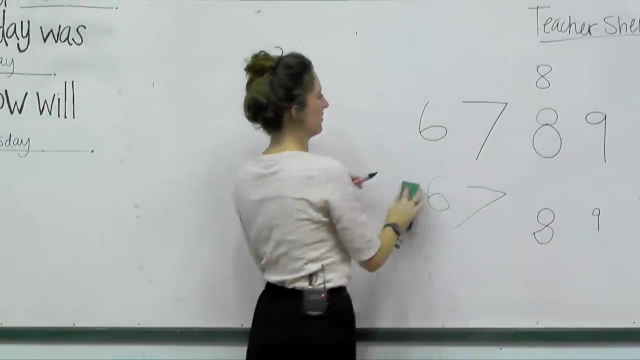 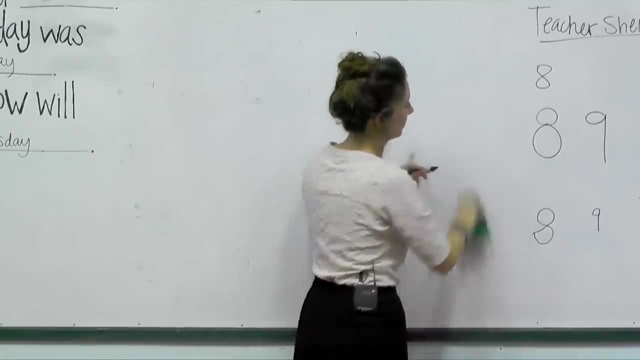 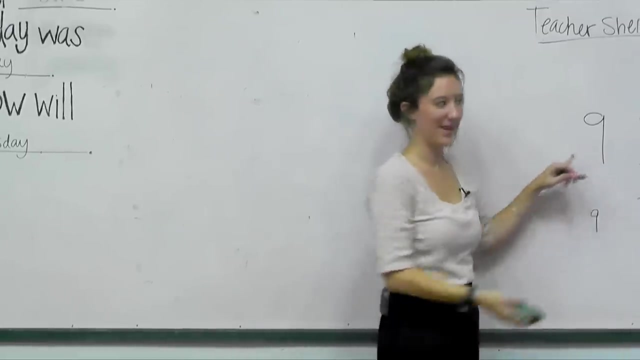 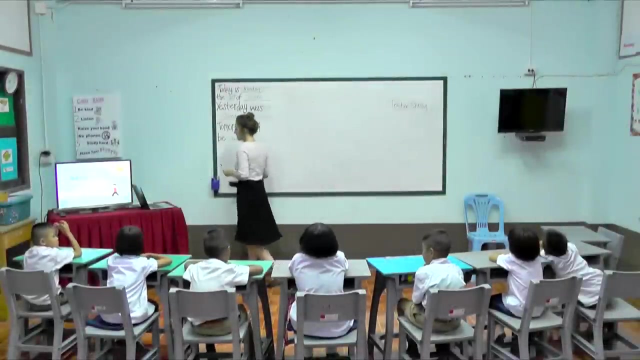 Six- Wait for me- Seven, Eight, Nine, Ten- Good job, This one. Four, Four, Four, Five, Five, This is a five. Six, Seven, Seven, Eight, Nine, Nine, Nine And ten. Okay, so let's see if we can repeat them with a little bit of rhythm. One: 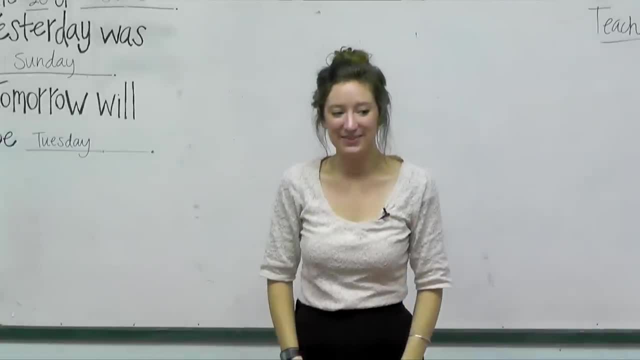 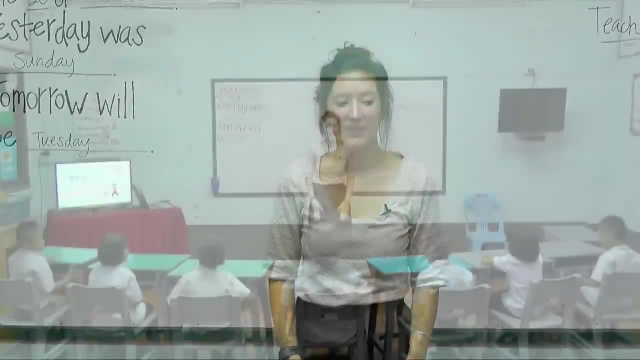 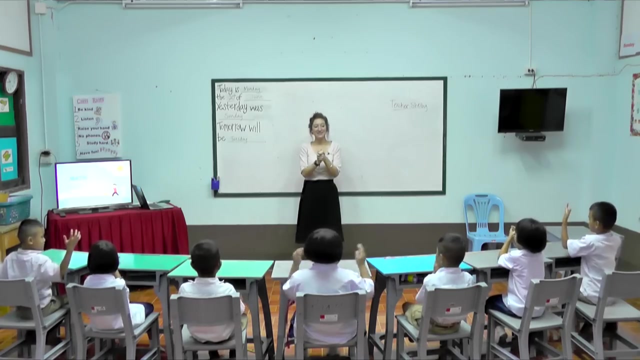 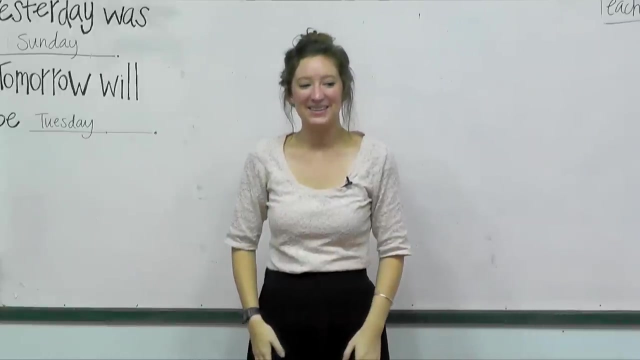 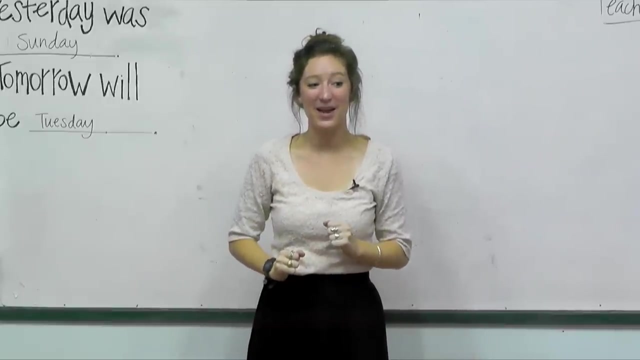 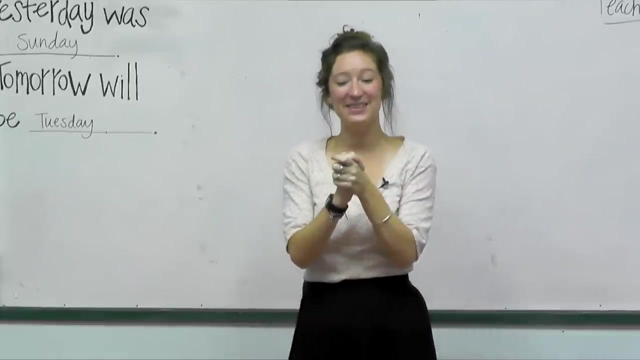 One, Two, Three, Four, Five, Six, Seven, Eight, Nine, Ten. Good job, Let's try. We'll get a little bit faster each time, okay, So do it with me. One, Two, Three, Four, Five, Six, Seven, Eight. 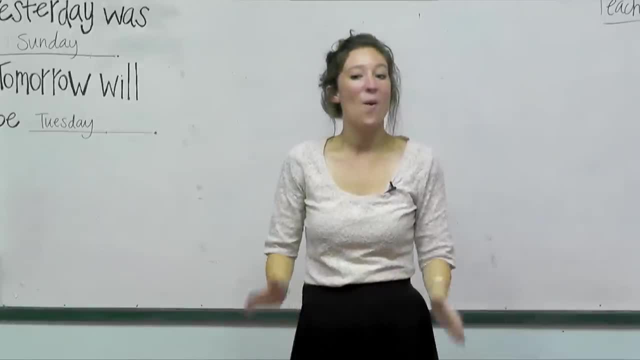 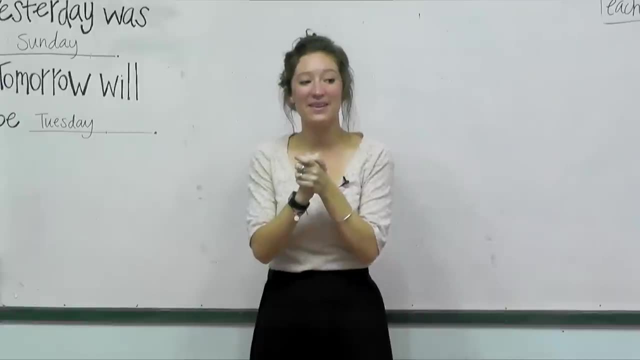 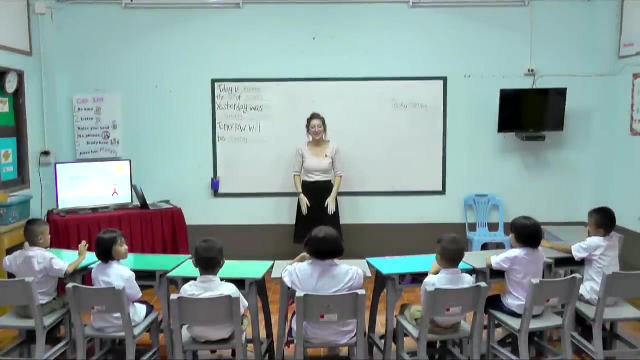 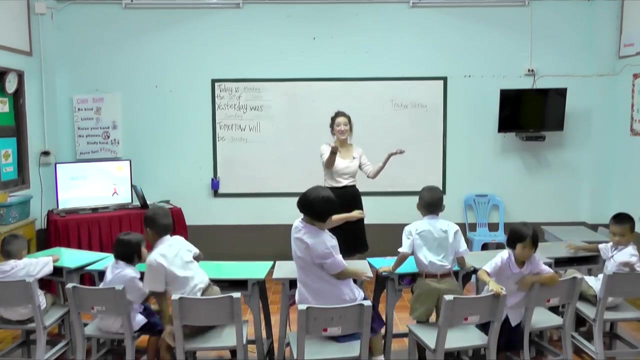 Nine, Ten, Ten, One, Two, Three, Four, Five, Six, Seven, Eight, Nine, Ten. Very good, Okay, and we'll try it one other way. Can you please stand up for me? Everybody stand up. 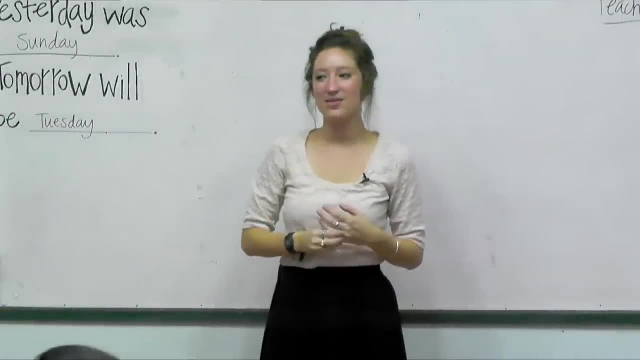 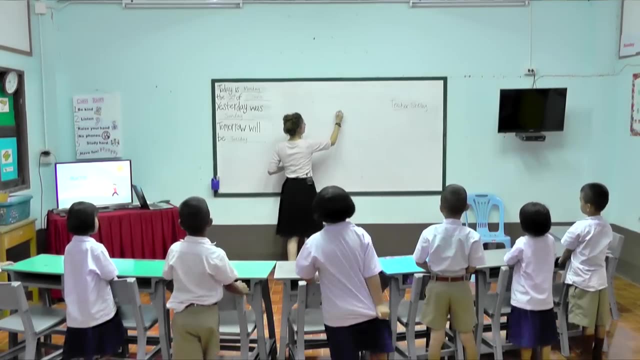 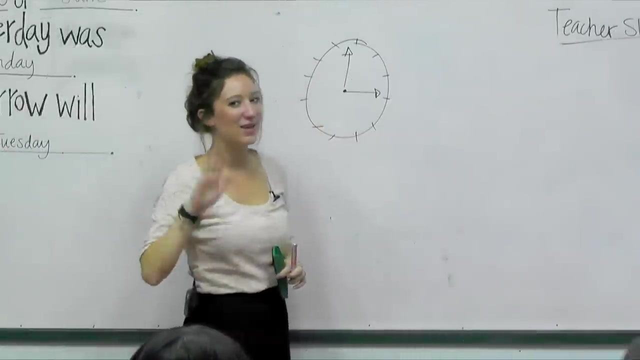 We're gonna practice counting like a clock. We know clock. We're going to pretend, So we've got our clock. I heard you guys saying some tick-tock, tick-tock, tick-tock. That's right, That's what a. 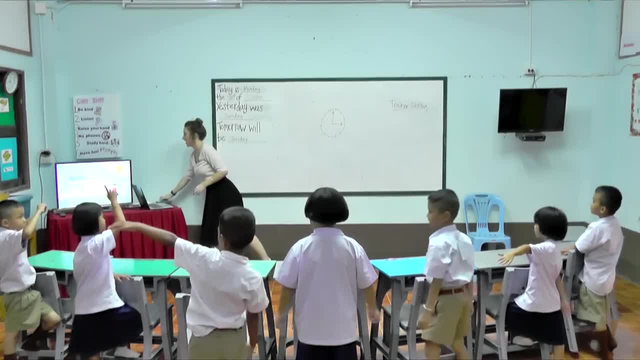 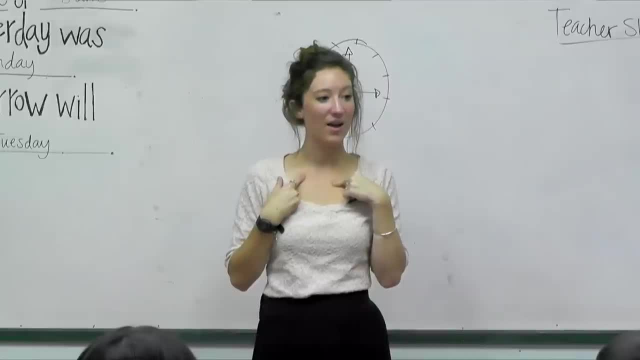 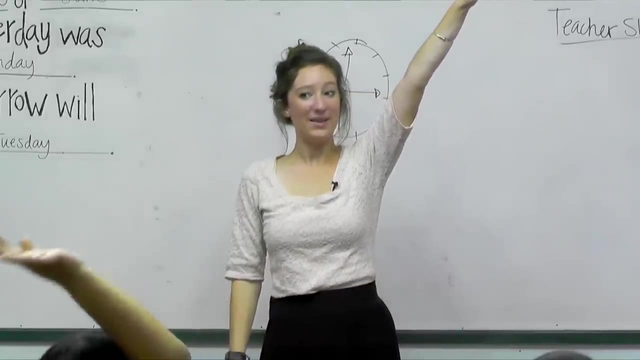 clock makes Tick-tock. Okay, so let's practice our counting, pretending that we are a clock Right. So let's start here. Everybody start here. One, two, three, four, five, six, seven, eight, nine, ten. Great job, Let's do it one more. 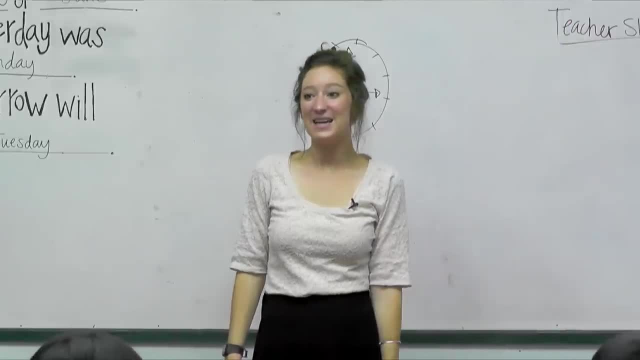 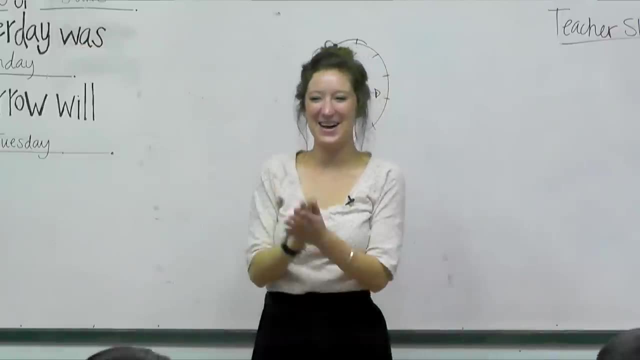 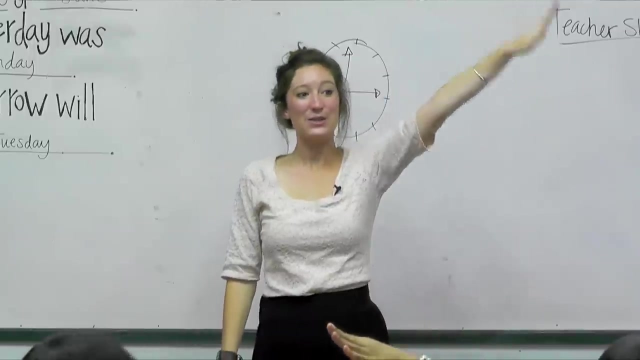 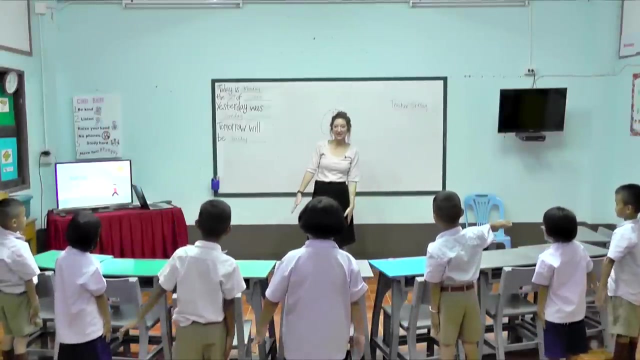 time. Show me your one, Show me your one hand. everybody, One, two, three, four, five, six, seven, eight crack Ten, Four, five, six, seven, eight, nine, 10.. Very good, excellent. 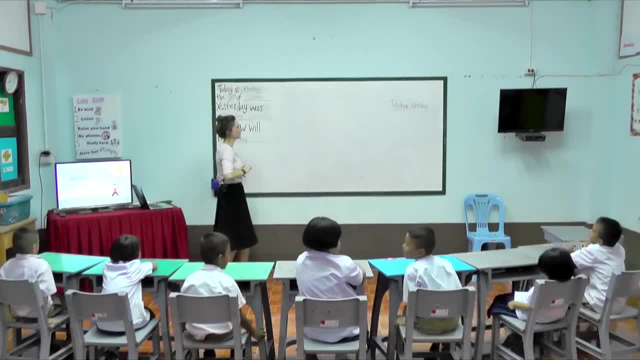 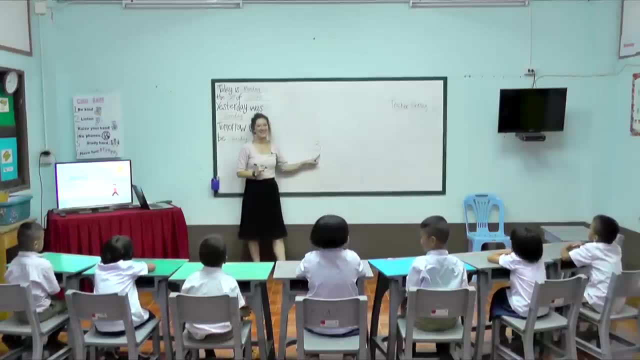 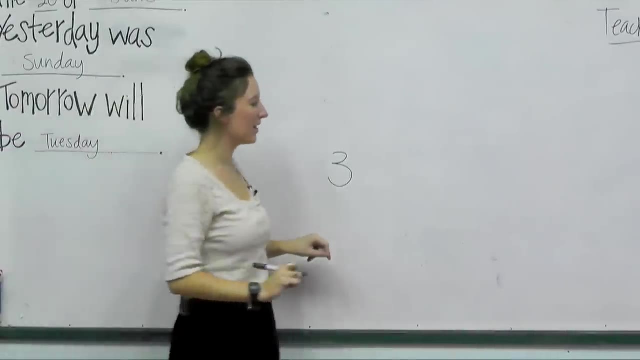 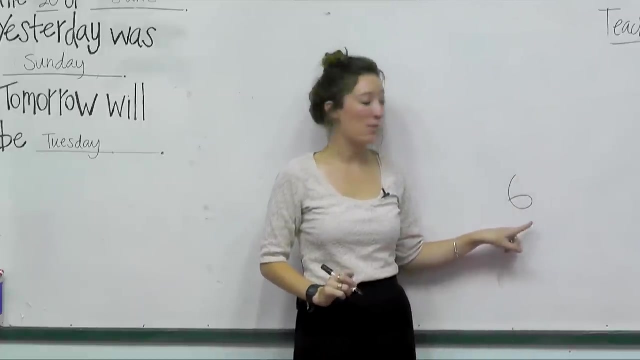 We'll play that again later. Thank you, have a seat. This is recognizing our numbers Three. What number is this? Three, Three, Three. this is the number three. Three, Very good, So Six. Oh, you guys are so smart. 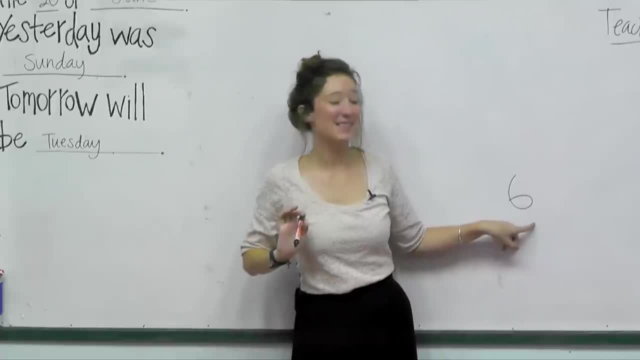 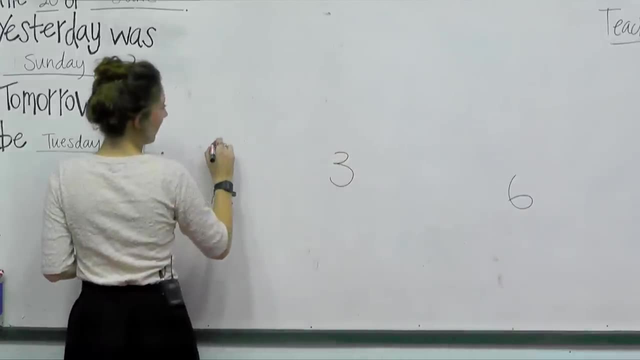 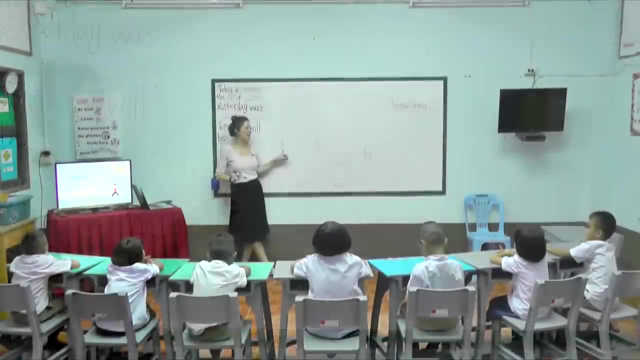 What number is this? Six Six, this is the number. six, Six, Six, Six, Six, Six, One One. That's an easy one. yeah, What number? One? One, this is the number one. So what about? 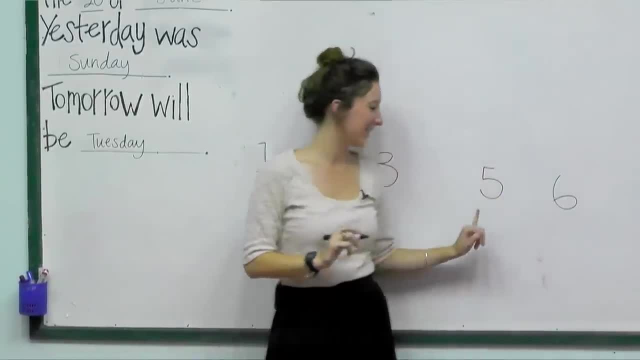 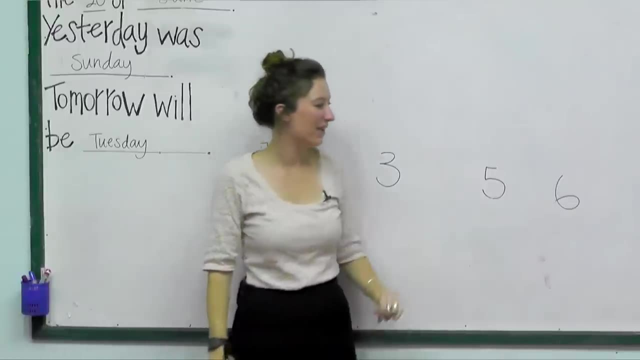 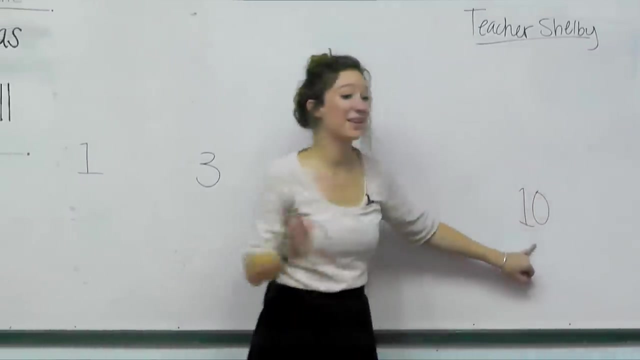 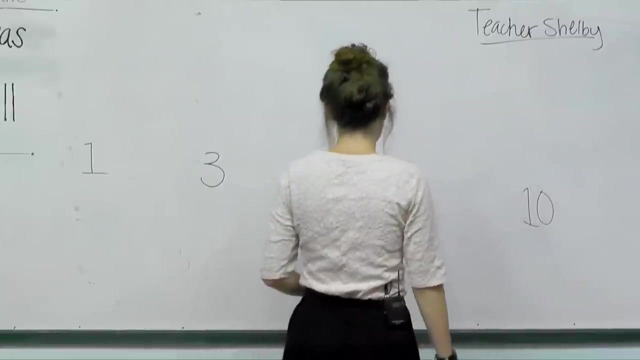 Five. How did you know? Five, Five, Five, Five, Five, This is the number five. Five Good Seven. Seven, Ten, Ten, Ten: This is the number 10.. Very good, So what about? 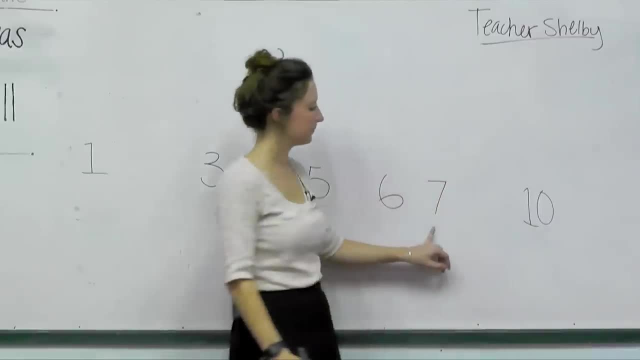 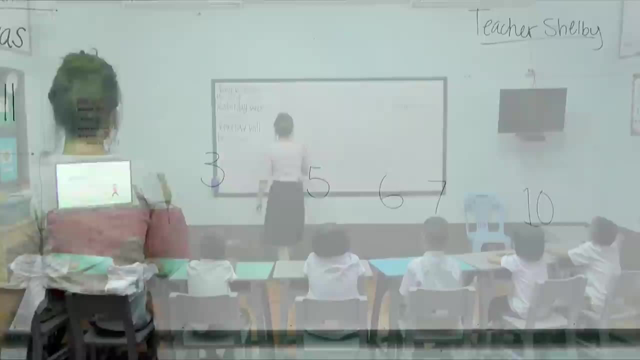 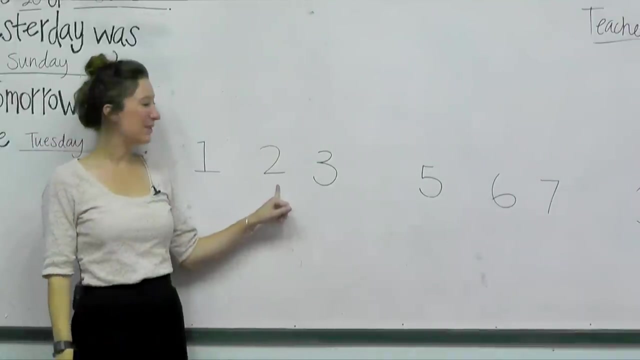 Five, Six, Six, Seven, Seven, Seven. That's right, this is the number. seven Seven Seven Ten Ten Two, Two, Two, Three, Four, Four Two Two. This is the number two. 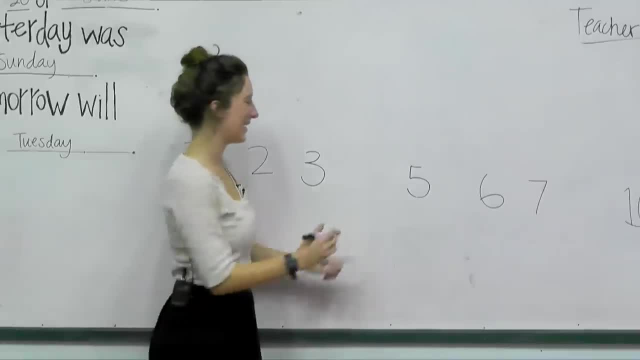 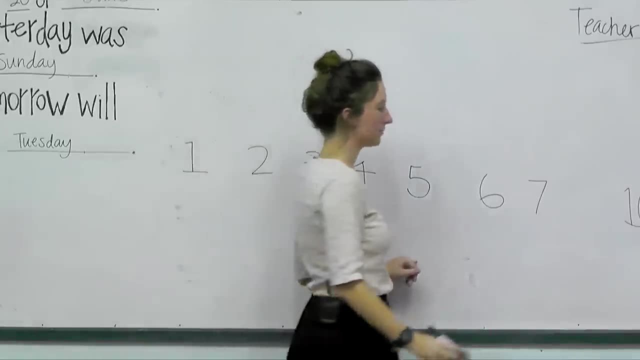 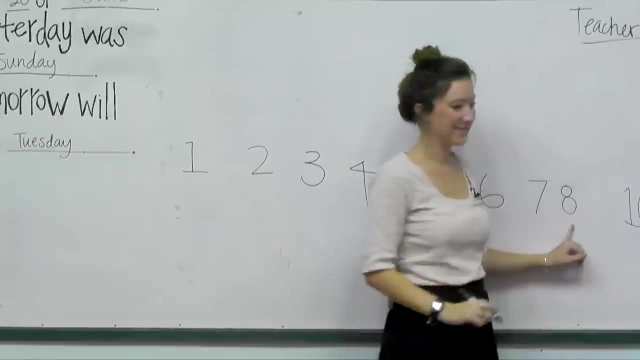 So what goes here? Four, Four, Four, That's right, the number four. The number four goes here: Seven, Seven, Six, Six, Nine, Nine, Nine, Nine, Nine, Nine, One, One Eight. 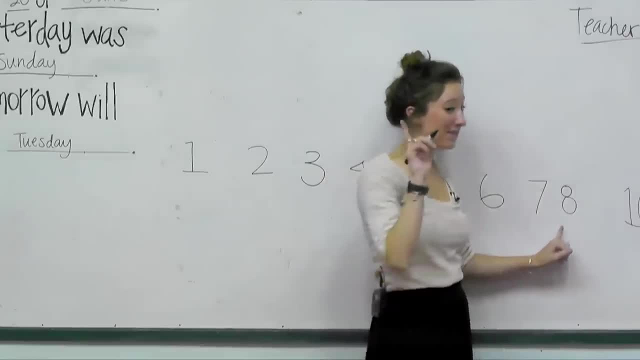 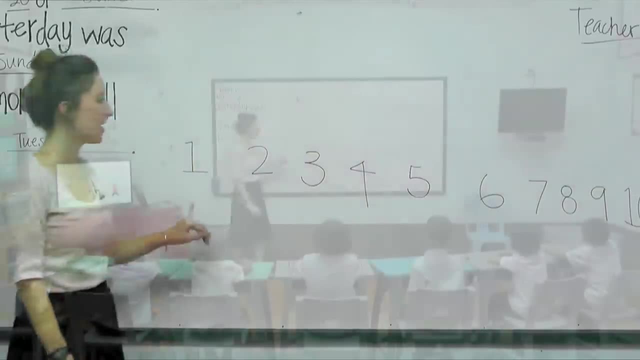 Eight, Eight, This is the number eight. And then what was Nine, Nine, Nine, And then nine, Nine, Nine. So let's say them all together: One, Two, Two, Three, Four, Five, Six. 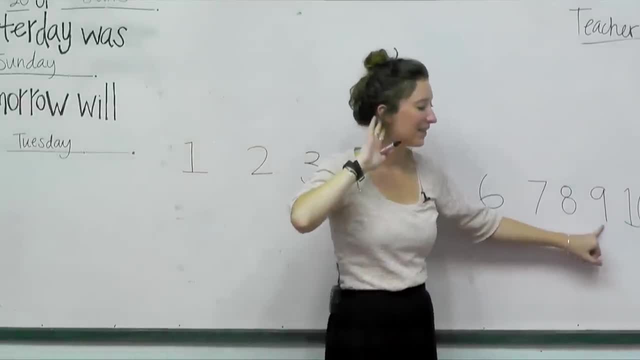 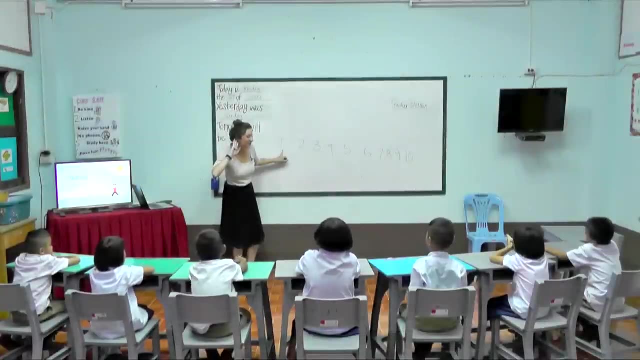 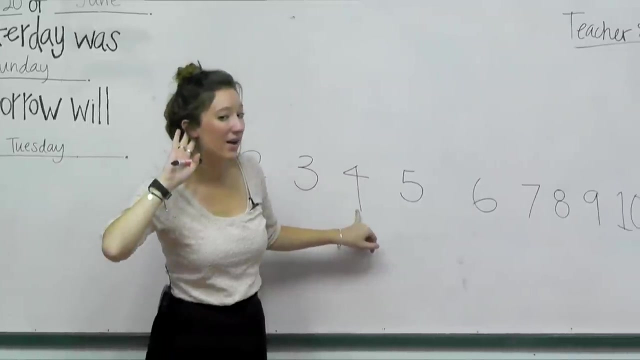 Seven, Eight, Nine, Ten, Two, One, Two. Good job. One One, One, Two, Two, Three, Three, Four, Four, Four, Five, Five, Five, Five Five, Six, Six. 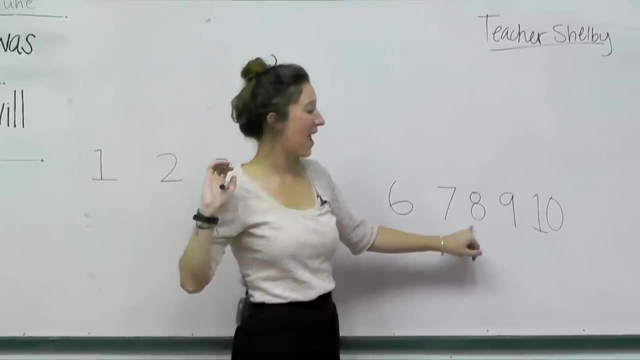 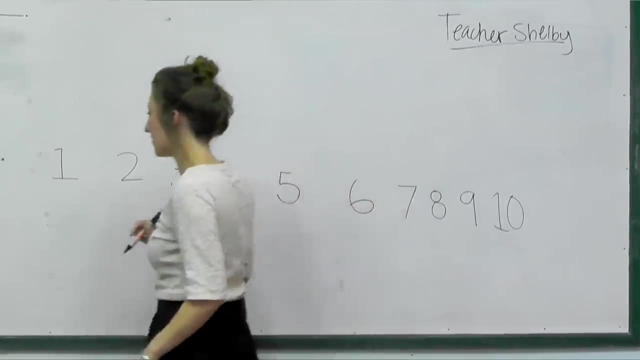 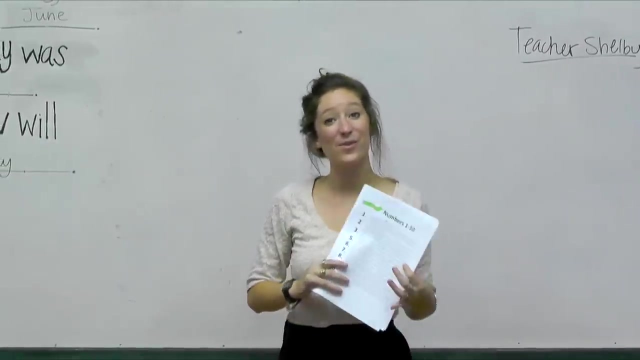 Six, Seven, Seven, Seven, Eight, Eight, Eight, Nine, Nine, Ten, Ten, Ten. Good job For our next activity. I'm going to pass out a worksheet and I want everyone to work on writing out the English numbers one through ten. 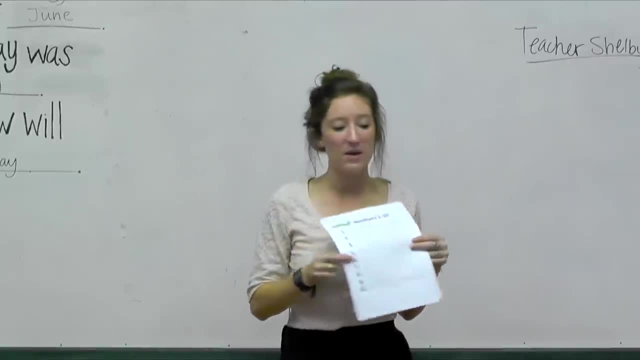 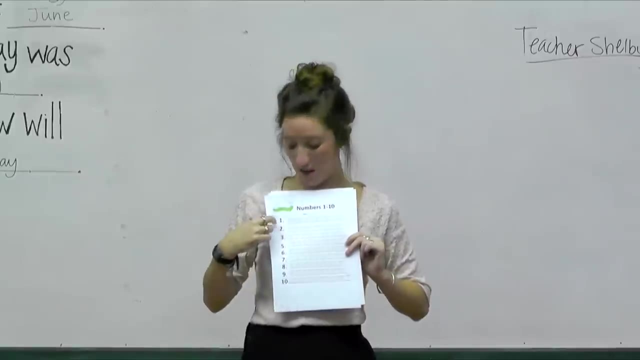 So your worksheet should look something like this: I'll give you a few minutes to pass it out, And then I want you all to complete on your own. Make sure that you are familiar with writing One, two, all the way to ten. 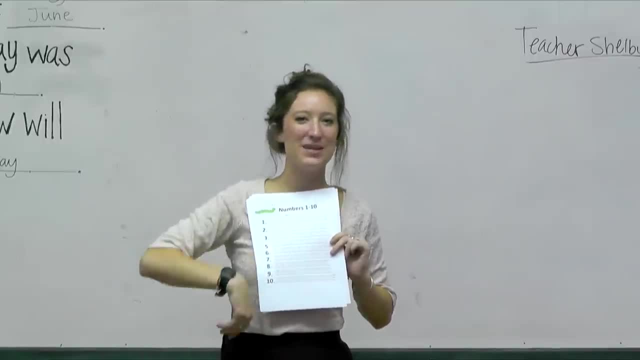 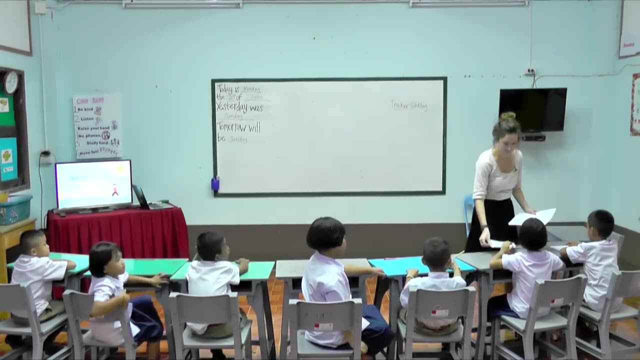 So I'll pass these out now and give you guys a few minutes to work. Join us back for our next activity. One two, One two. Welcome, Thank you, You're welcome. That's very good, Pat Boom. 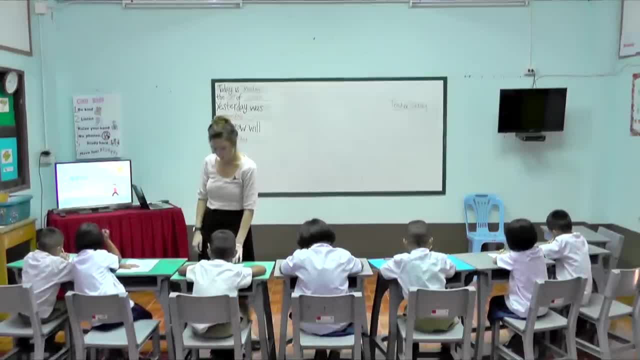 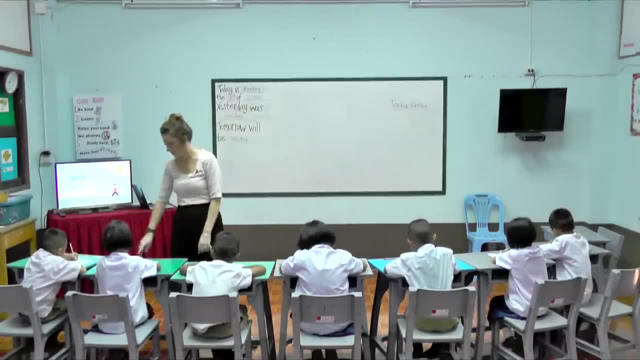 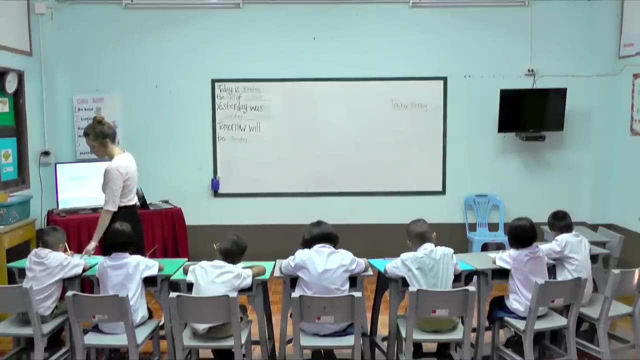 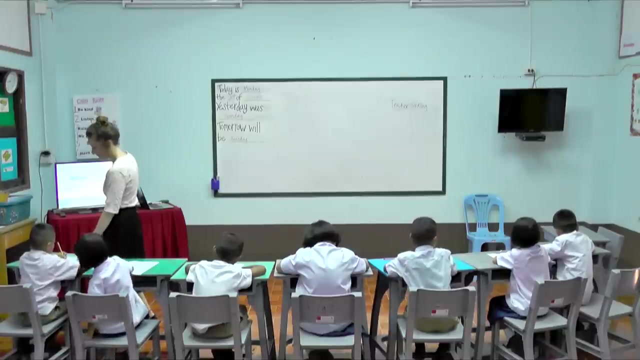 It's good. Do you remember, pat? You can look up here for help, Pat. What number is that? Two, Two. What number is this? Two? This one, One, One. That's the number one. What number is this one? 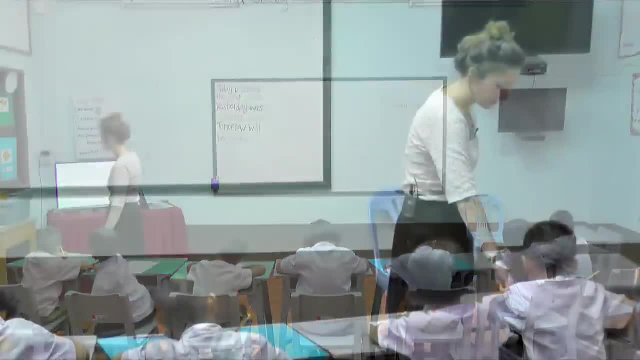 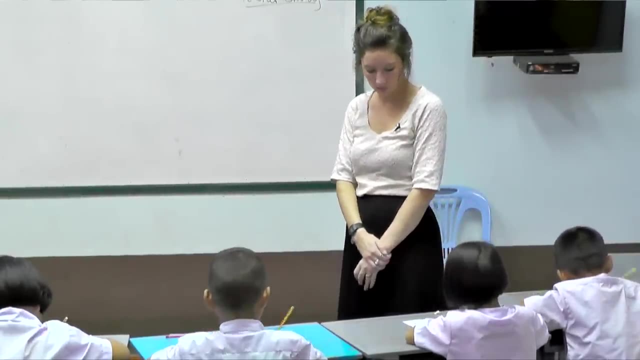 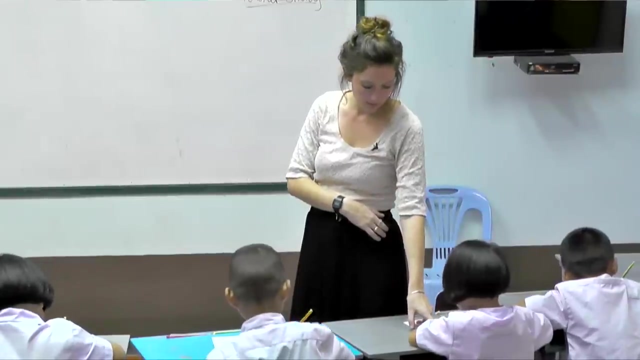 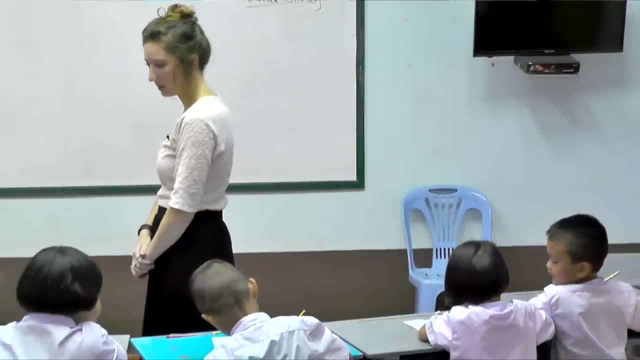 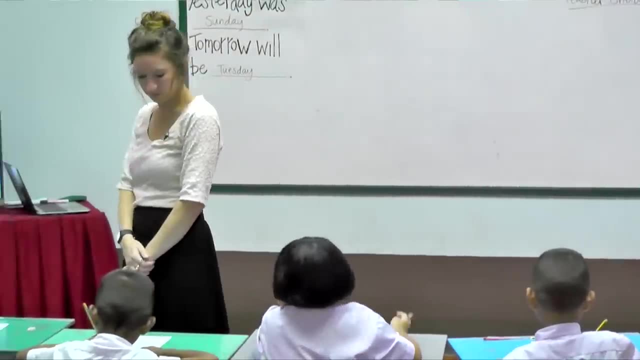 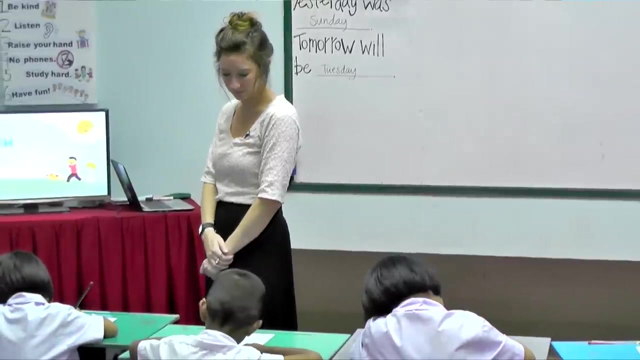 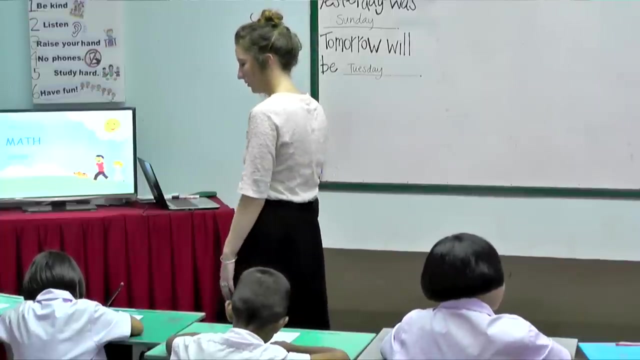 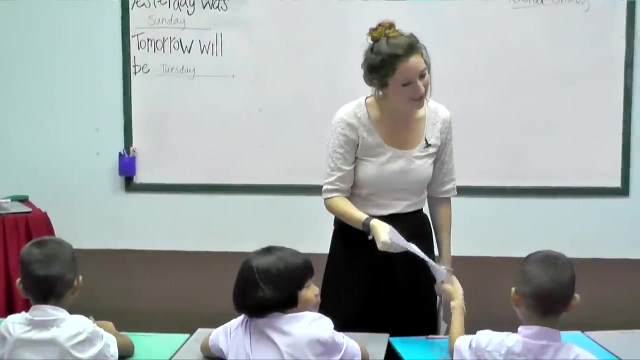 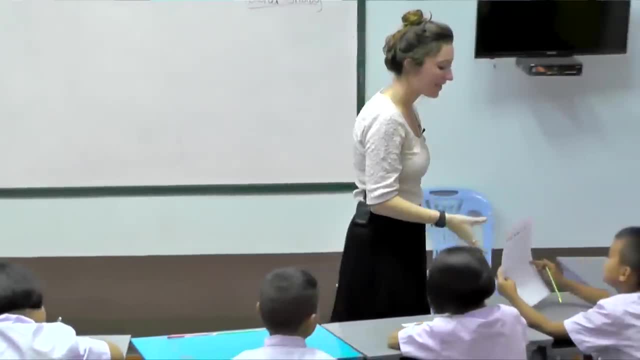 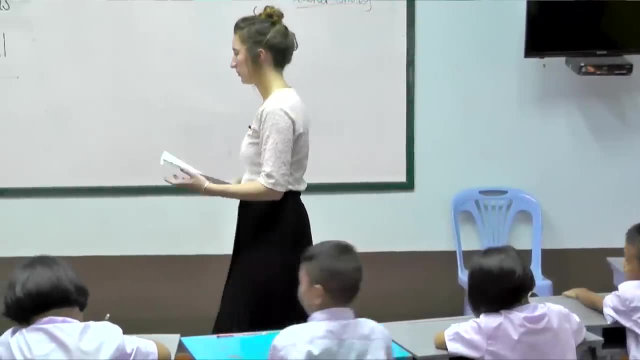 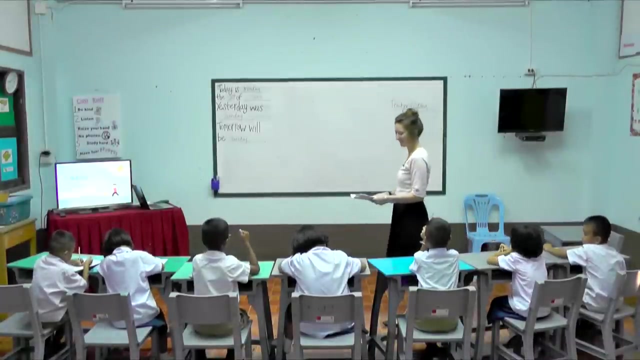 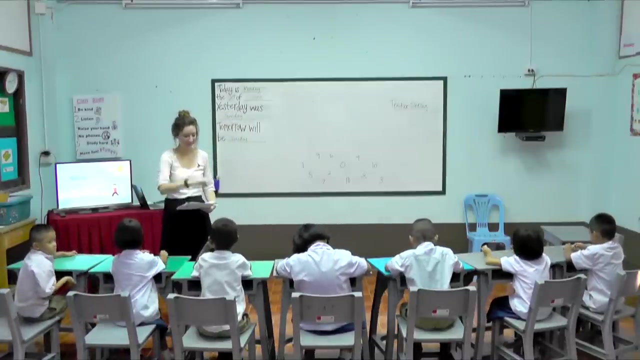 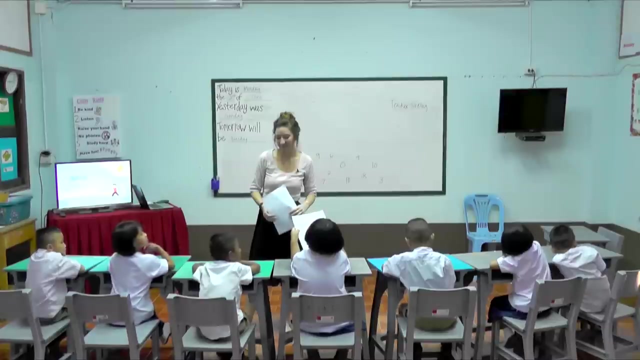 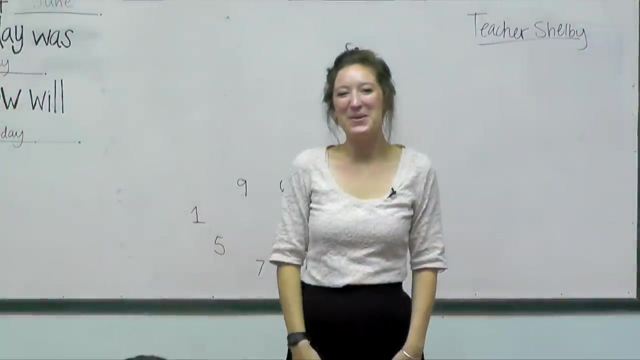 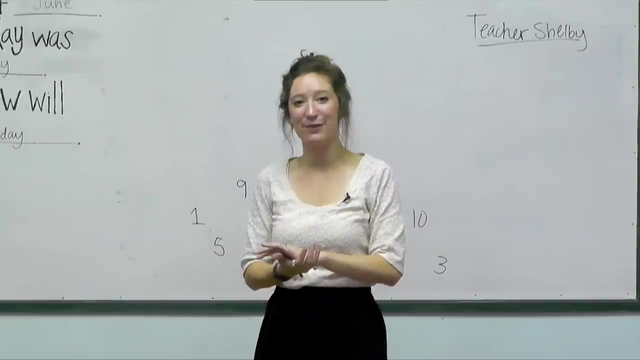 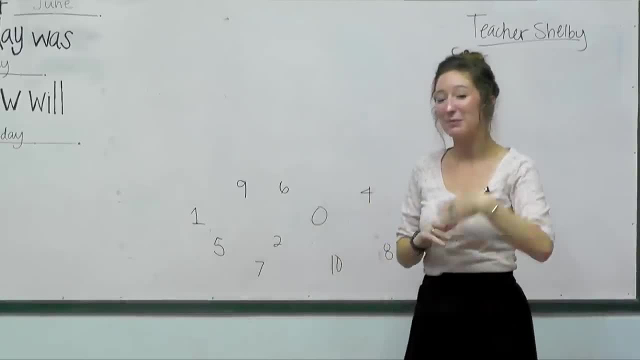 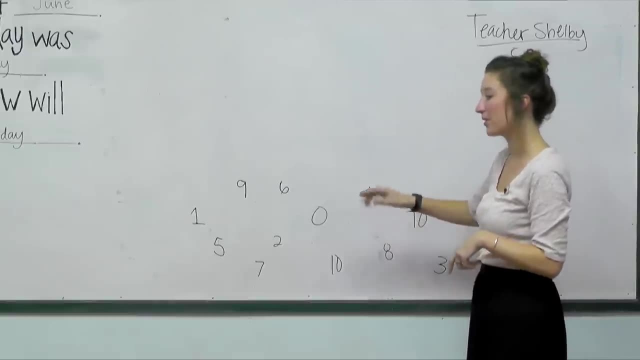 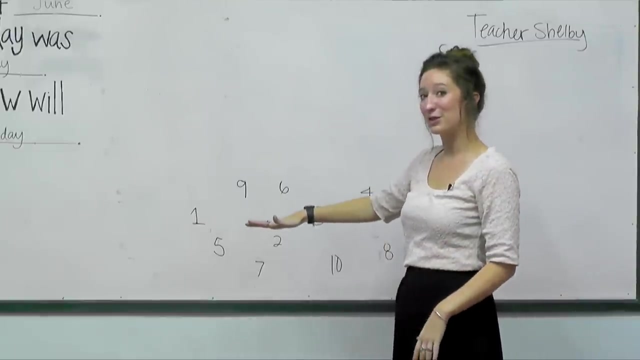 you can either watch us play or, even better, play in your own classroom with your volunteer. You want the board to look something like this: I've got the numbers zero through ten in jumbled order here on the board, within reach of the students. What I'll do is call. 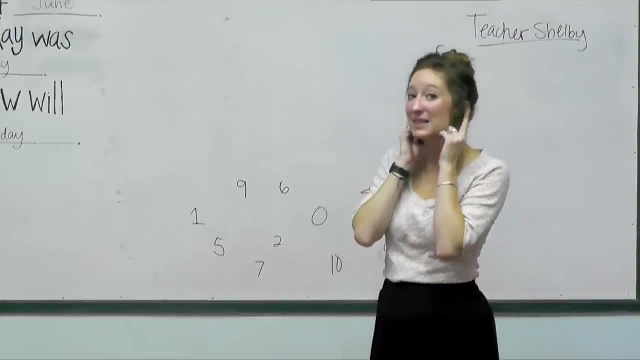 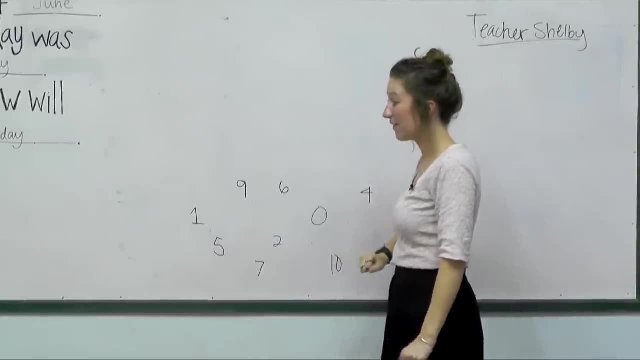 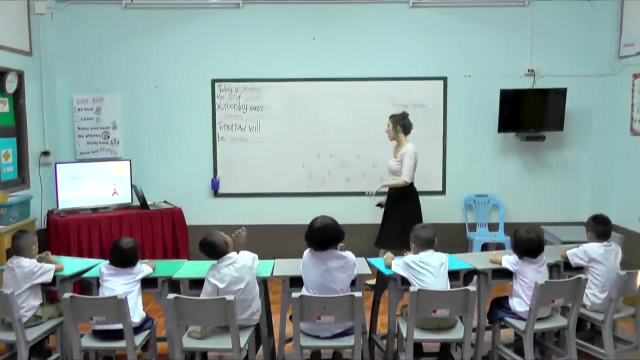 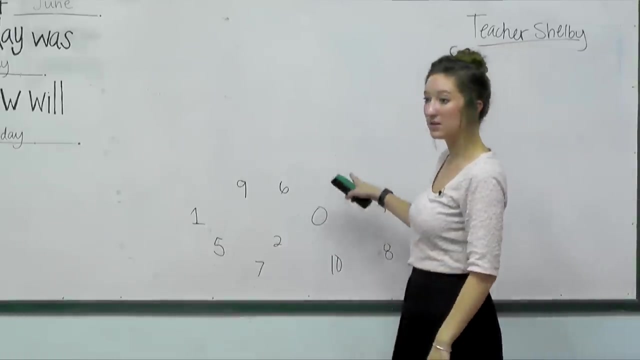 on one of you individually and you'll listen to the number that I ask and I want you to erase that number. So if I said we're listening, if I said show me six, I would want one of you to come show me. Does anyone see six? 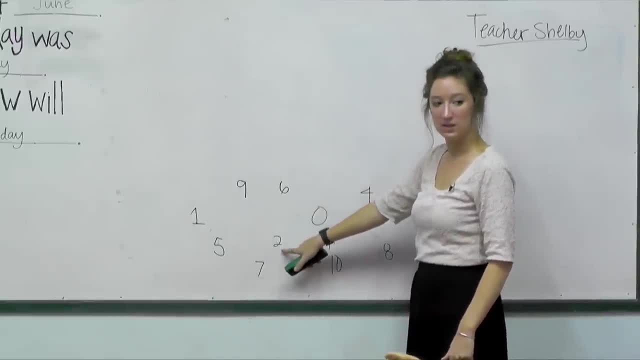 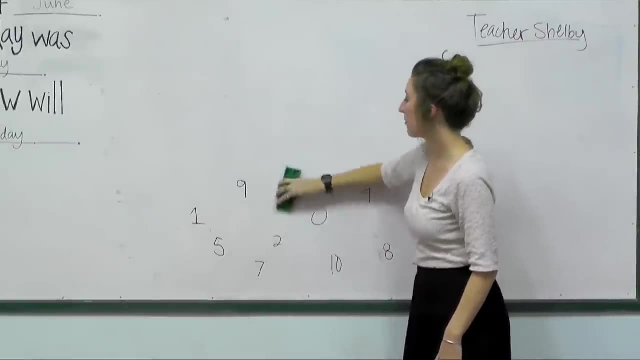 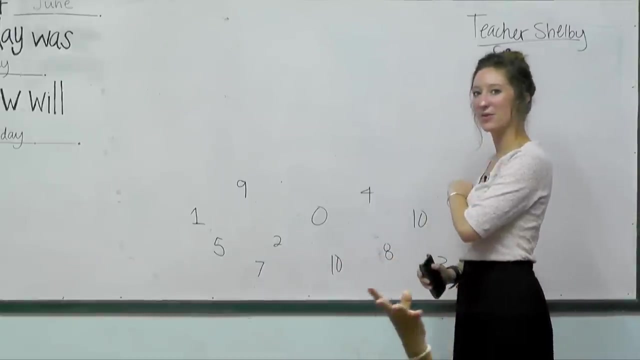 Where's six? Is this six? No, Is this six? No, Is this six? Yes, So we would erase it, right. So we're going to play like that until all of our numbers are gone. So if you guys will play with, 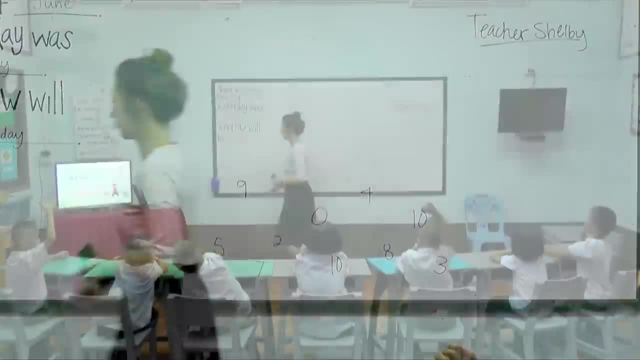 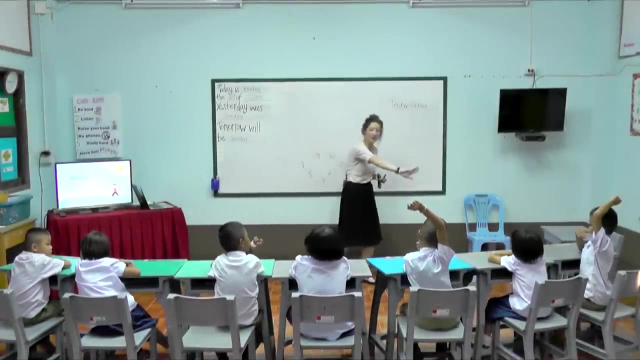 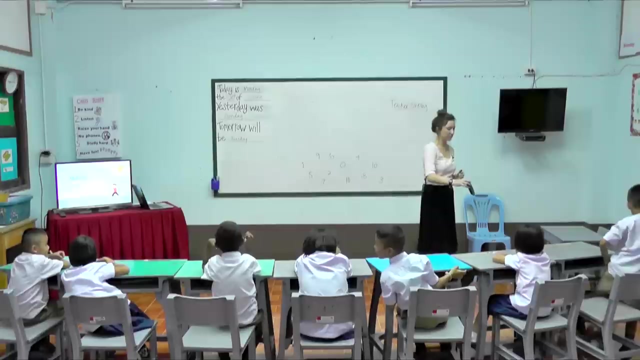 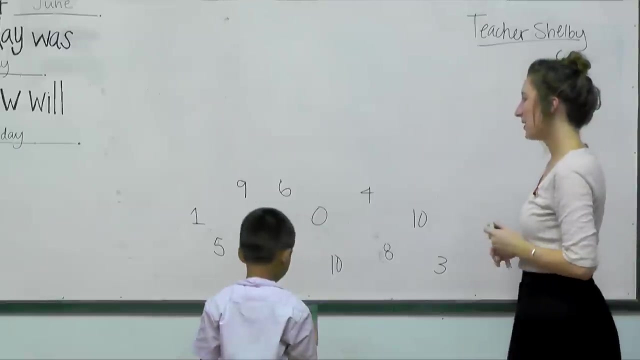 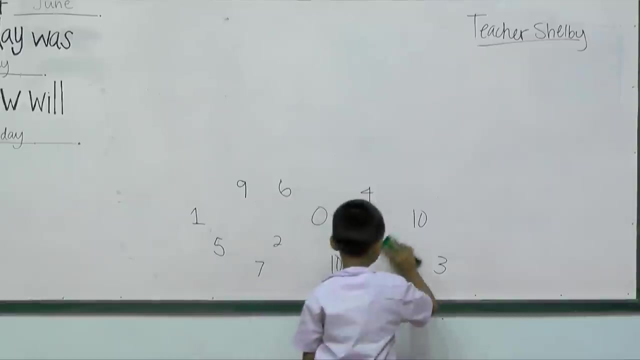 us and watch, for example. Okay, this time we'll start on this side and go this way. So, Patthe, you're first Listen. Patthe, will you show me eight, Eight, Eight, Very good. 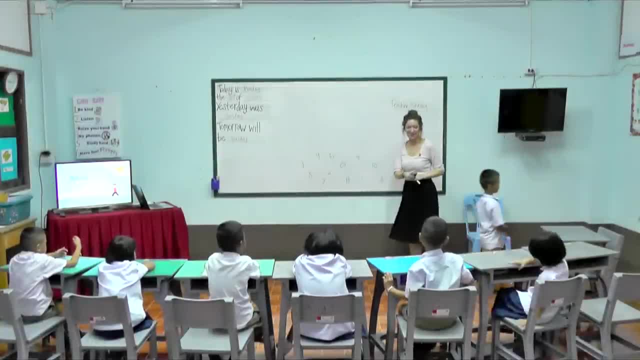 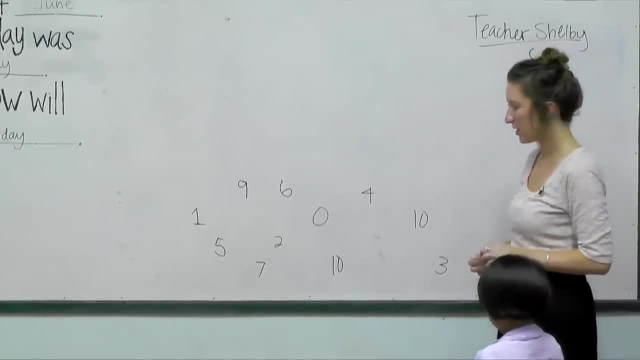 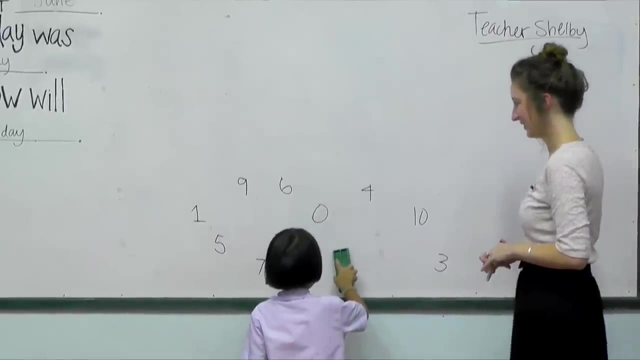 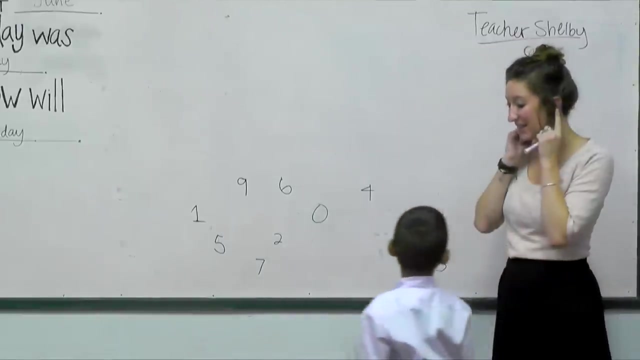 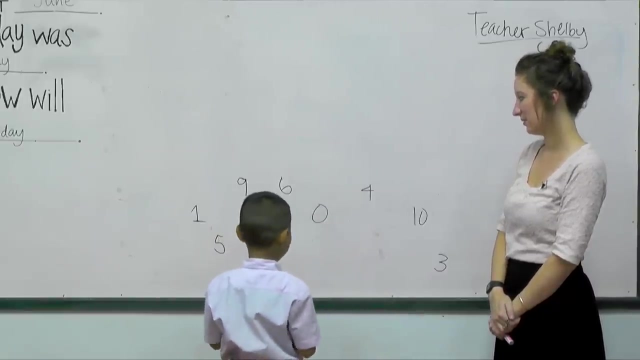 Good job, Very nice, Very nice. Okay, Will you show me ten? Very good, Very good, Thank you, Ready Listen. Will you show me seven, Seven, Seven, Seven Seven. 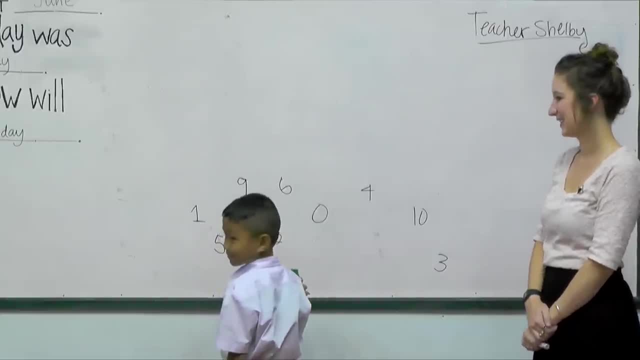 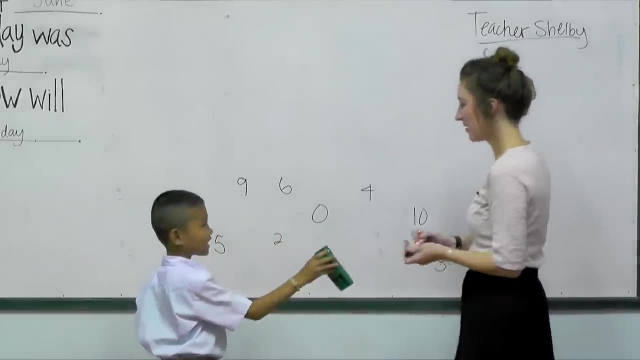 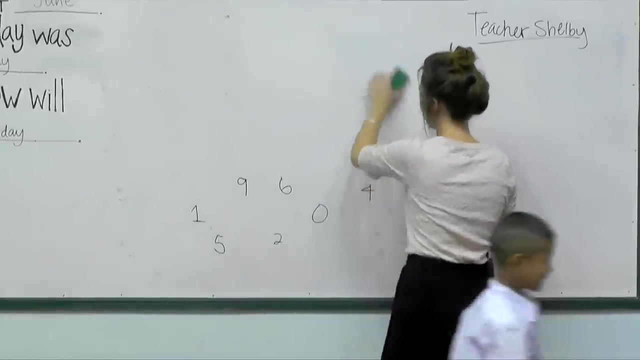 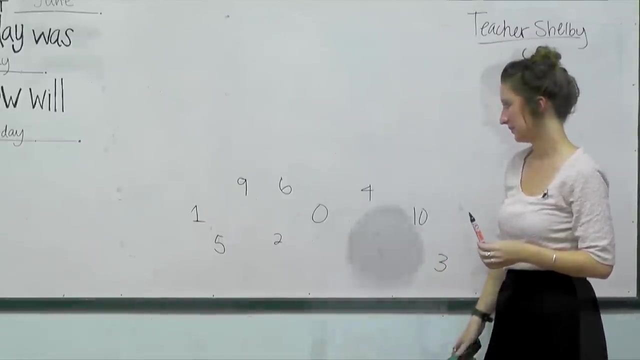 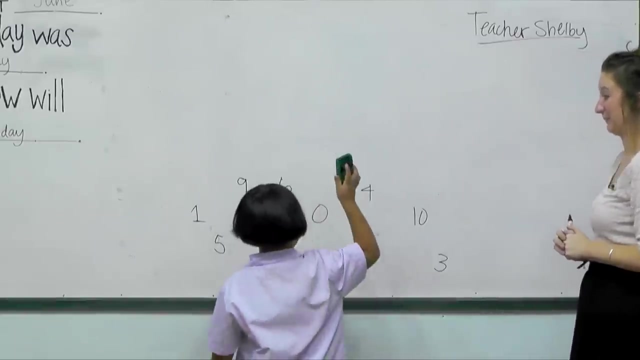 Seven. Don't tell him He knows That's right. Seven, Yeah, So look, Seven, Seven, Good job, Thank you, Okay, Will you show me five, Five. 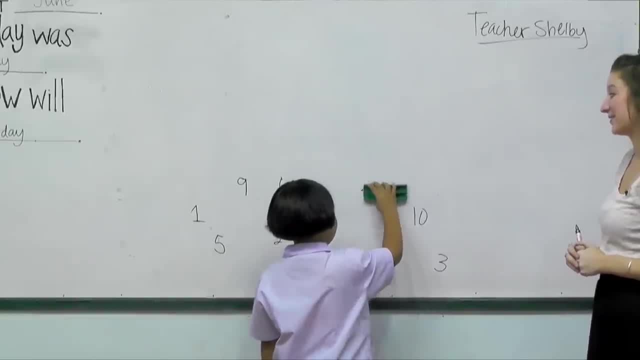 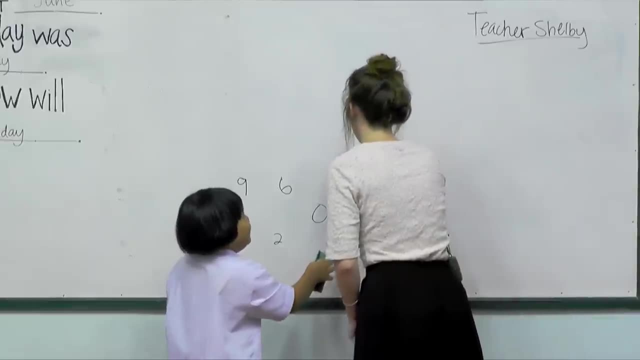 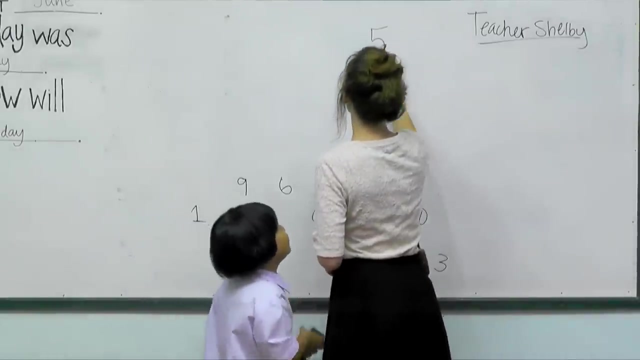 Five, Is that five? everybody? No, No, Take one more. look, This one is four, Five, Good job, Let go. What number is this? Five, Five, Hey, what number is this? 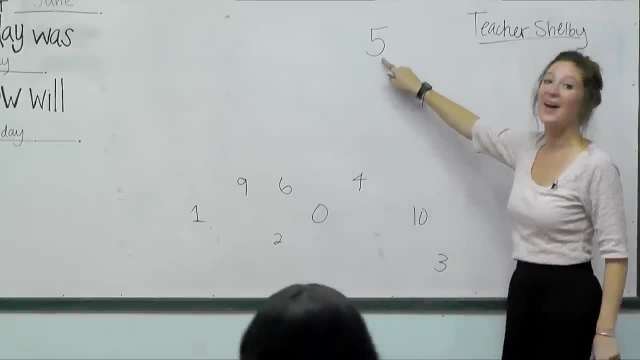 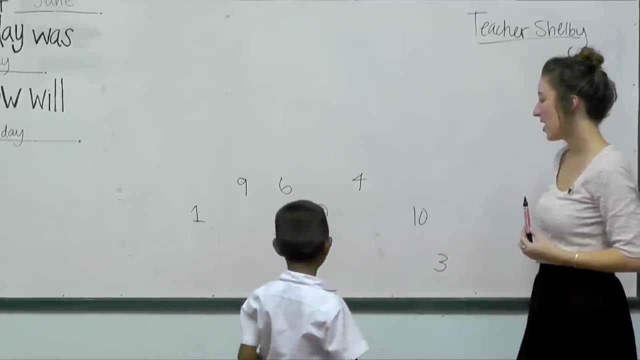 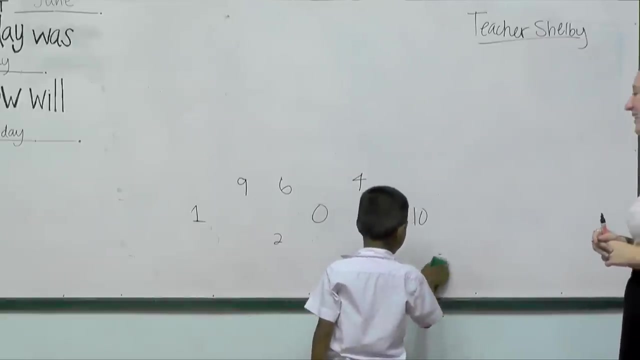 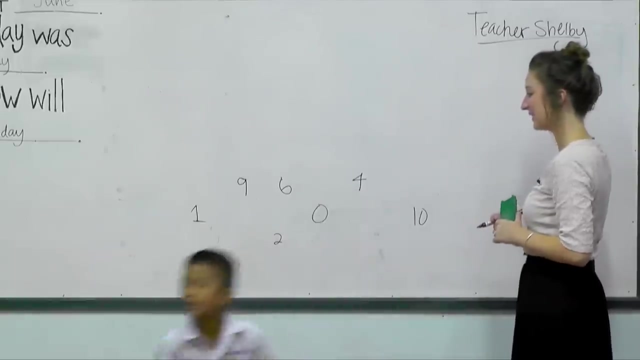 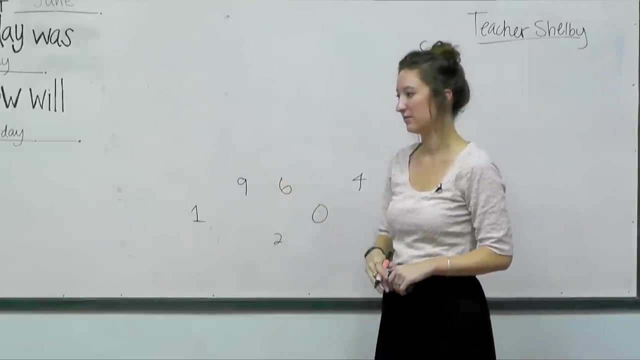 Five. What number is this? Five, Five, Very good. Show me three. Three, Three Very good Five. Very good Three. 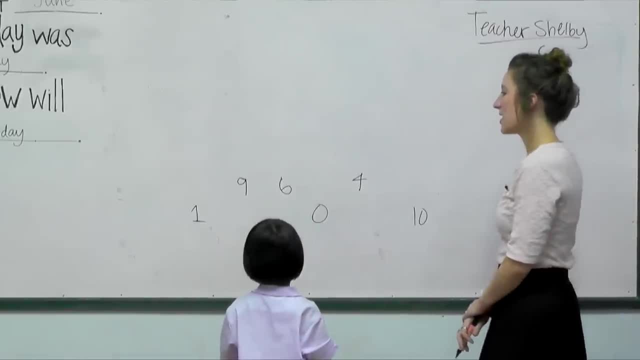 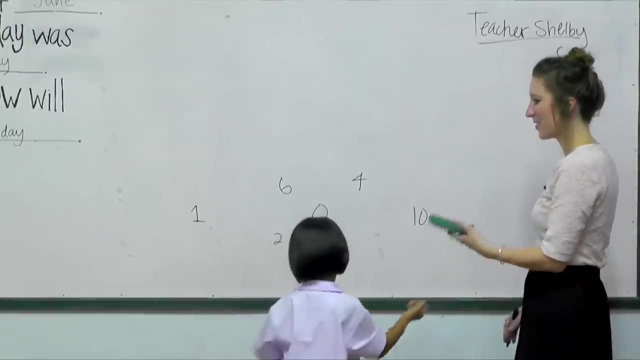 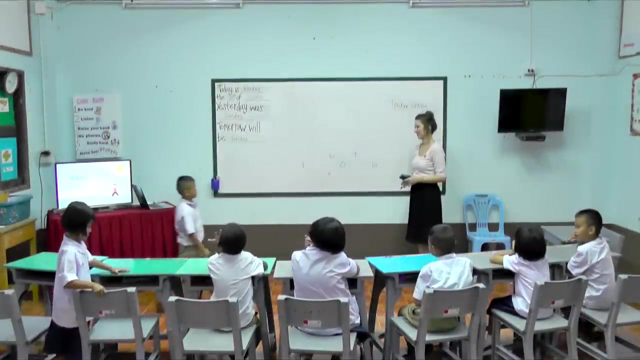 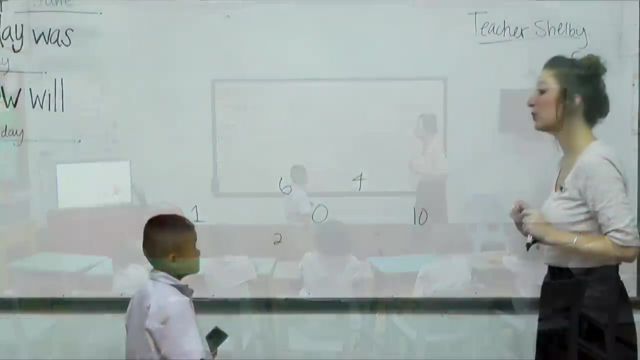 You're welcome. Will you show me nine? Very good, That's a nine, Great job. Now it's your turn. Will you show me Two, Two, Two. 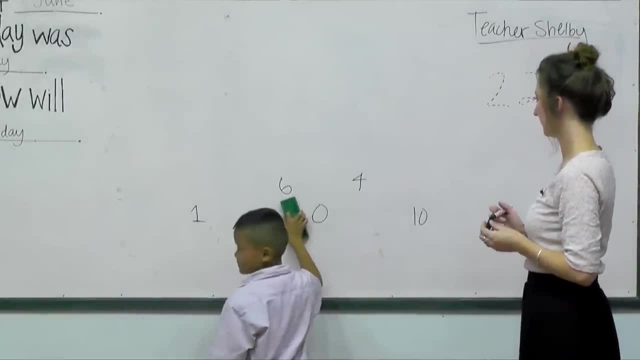 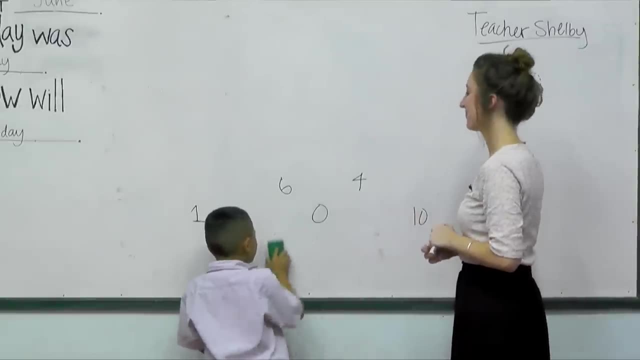 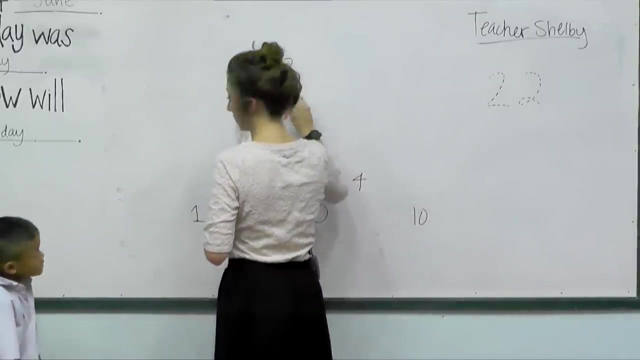 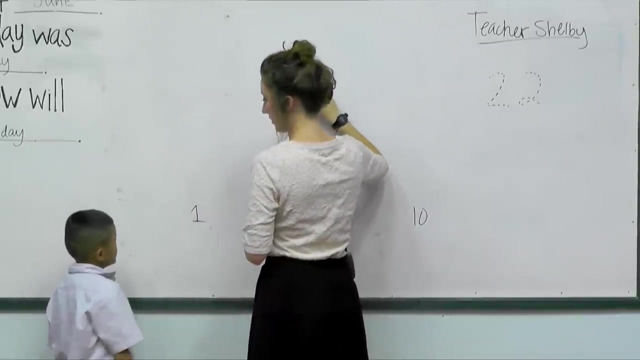 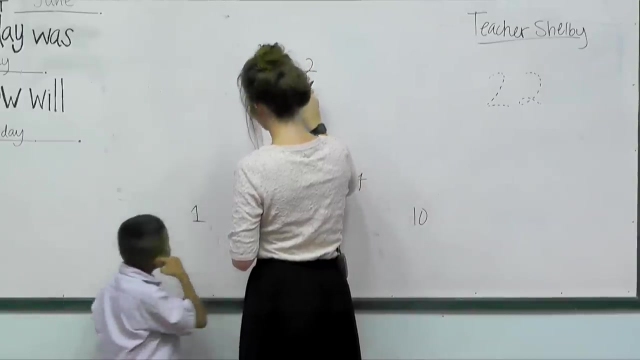 Two, You know it. Great, Two, Good job. So wait a minute. Two, Look at it. Two And this, Two, Two Same. 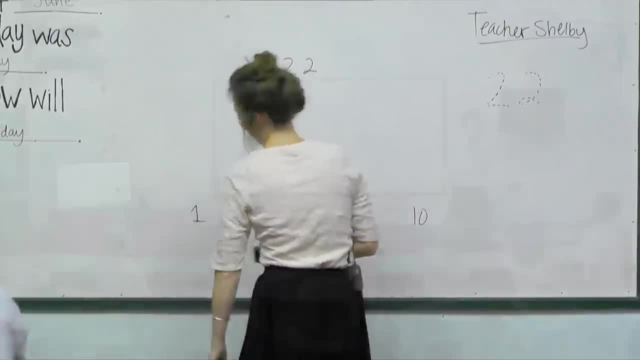 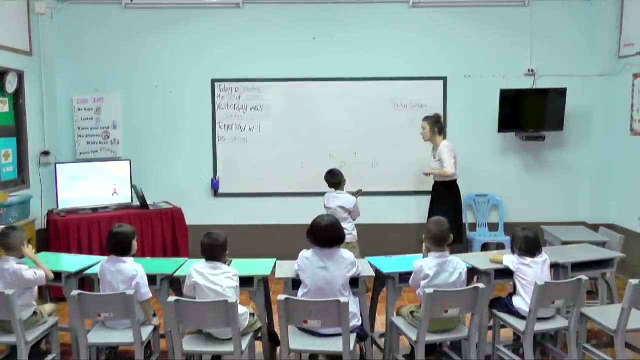 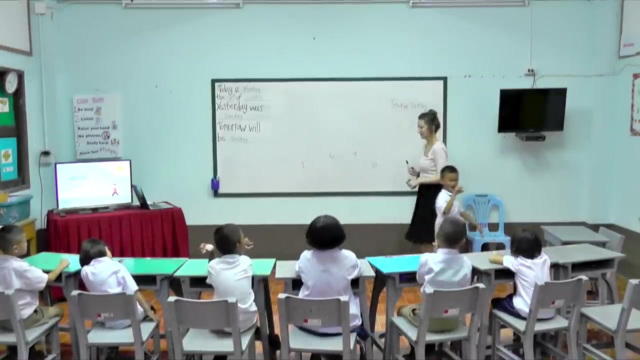 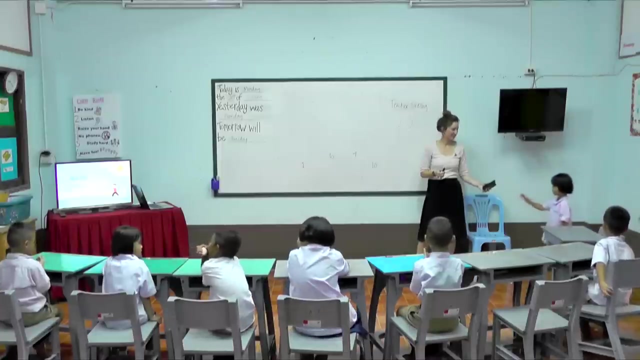 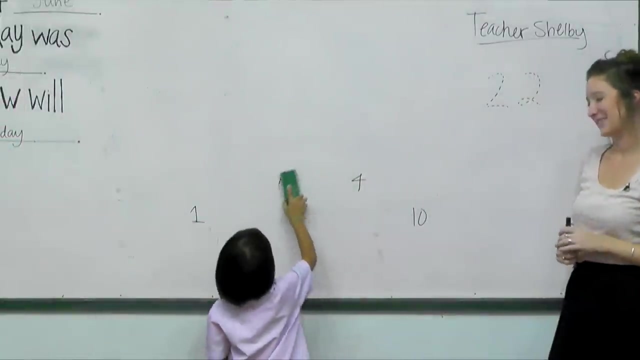 Three, Same Two, Two, Two, Two, Get it Two. Show me zero. Very good, Very good. Now show me Six, Six, Very good Six. 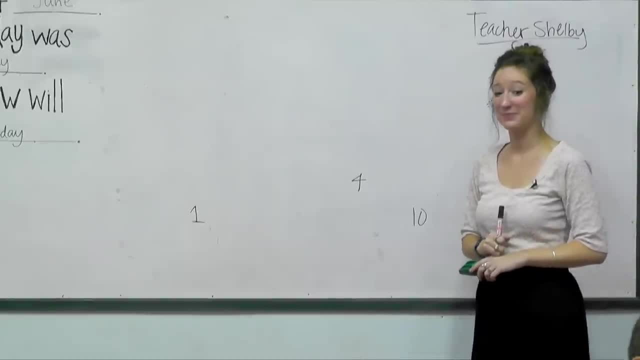 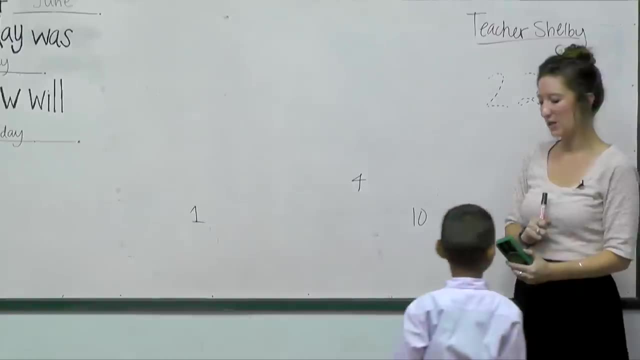 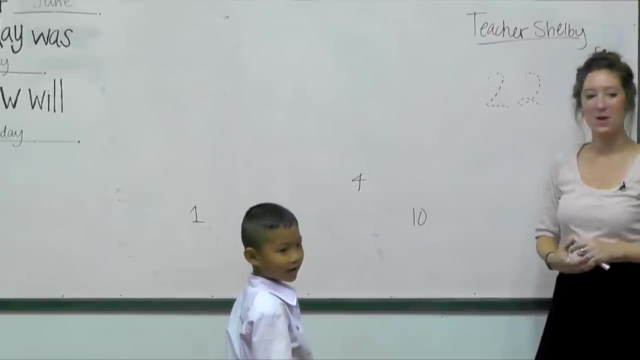 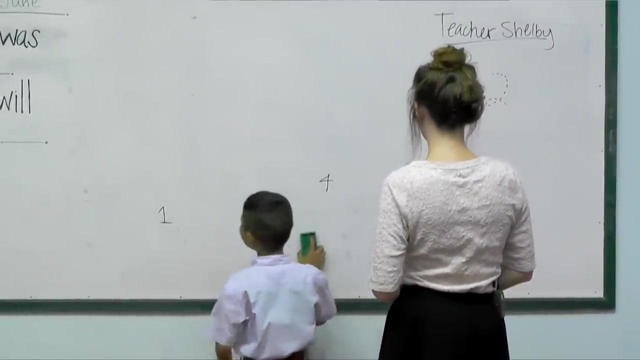 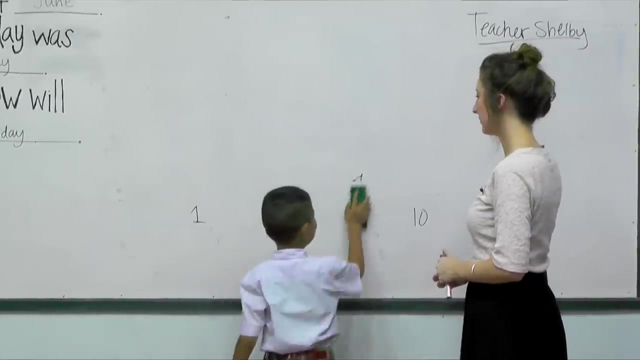 Great job, Show me Four, Four, Four. Don't look at them. Four, Four, Four, Four. One, Two, Three, Four, Four. Wait a minute. You wait a minute. 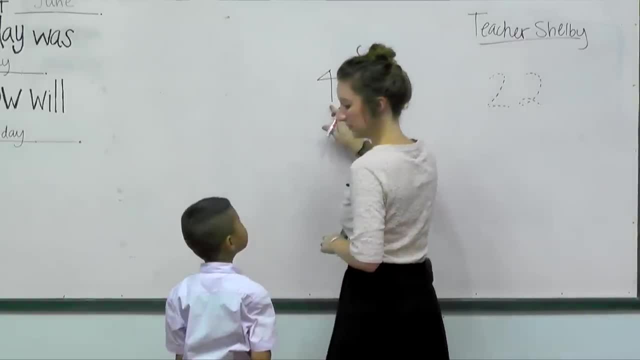 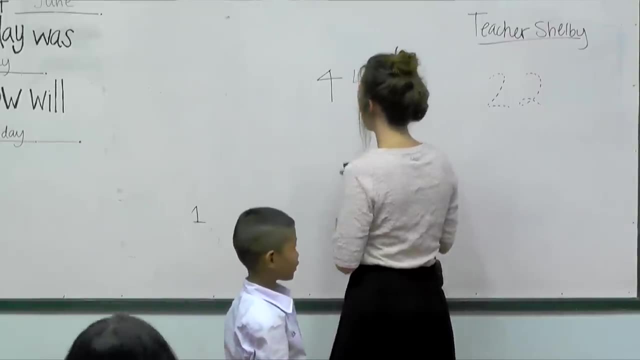 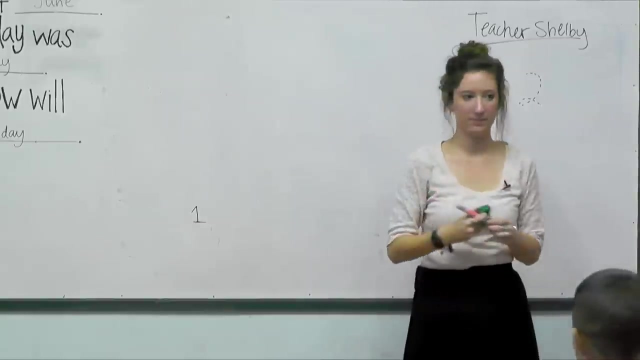 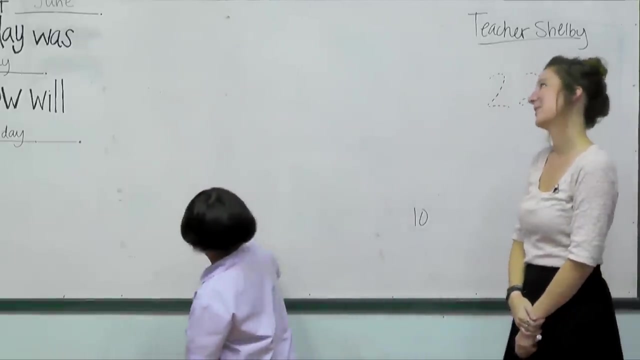 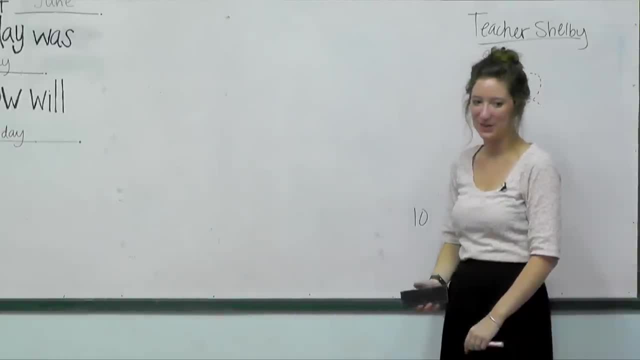 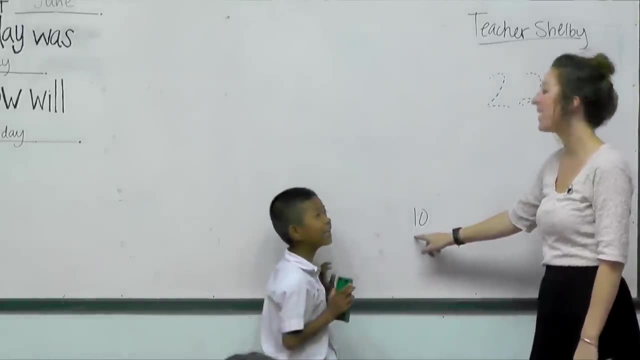 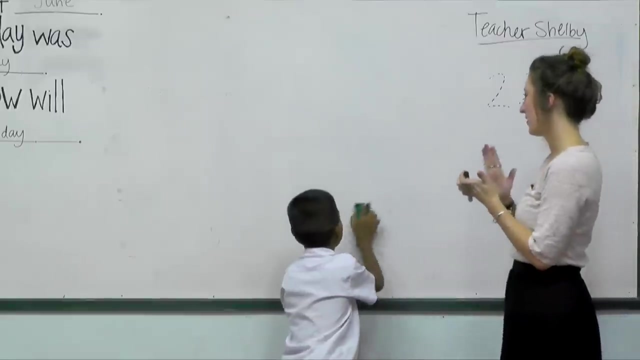 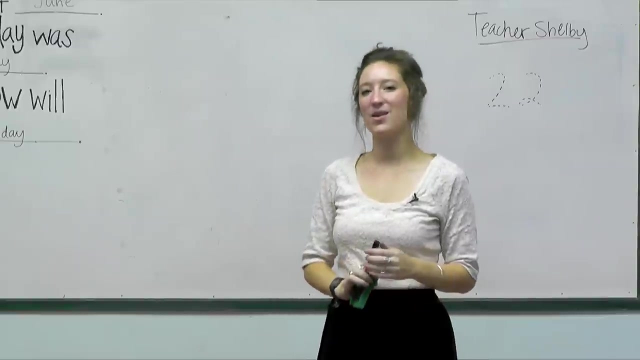 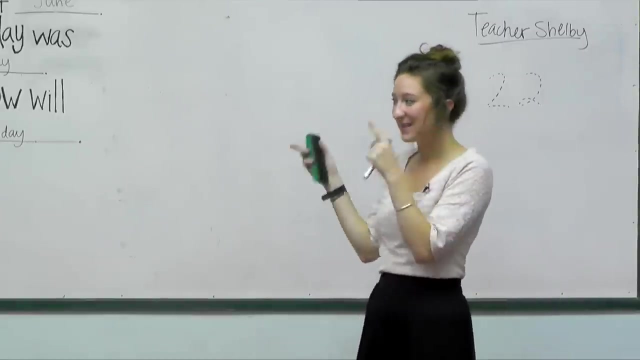 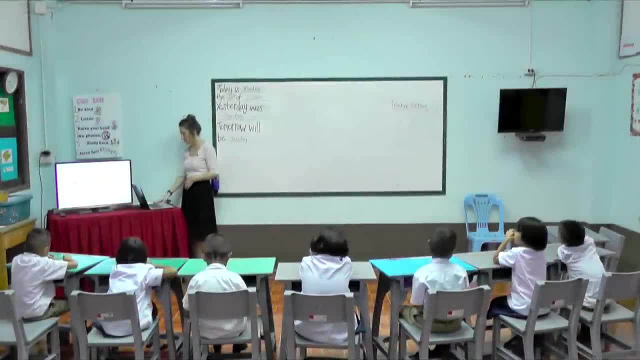 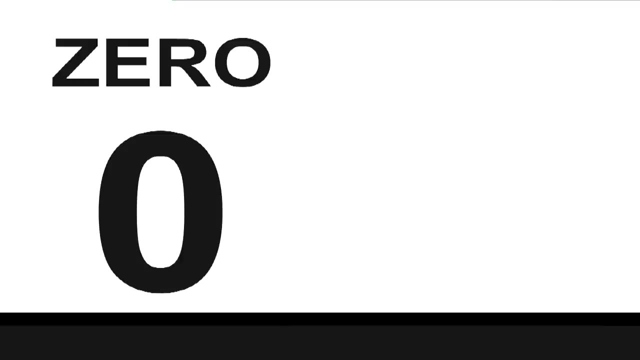 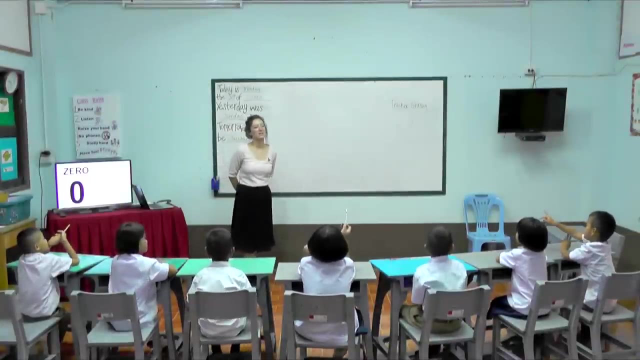 We're gonna go through something together: Numbers. we're talking about numbers, Zero. So what number is this? Zero, Zero, Zero. that's right. This is the number zero. Everybody say zero, Zero, Zero, Zero. Very good. 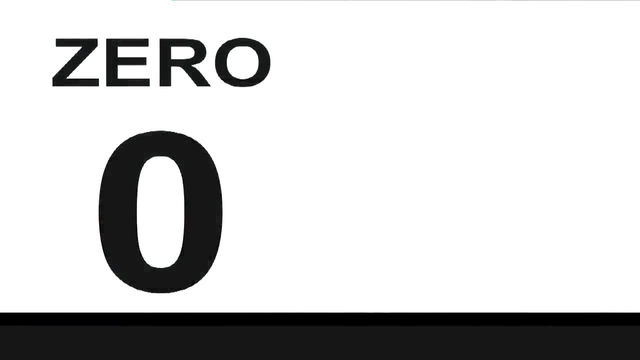 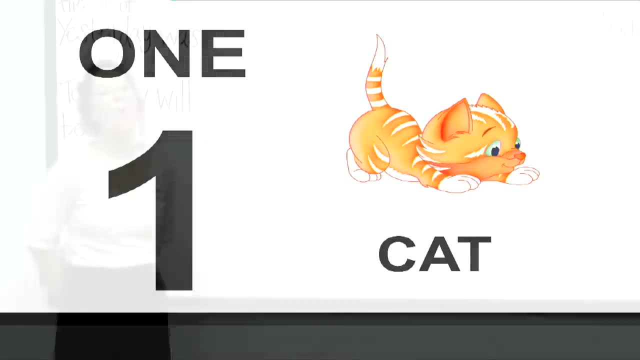 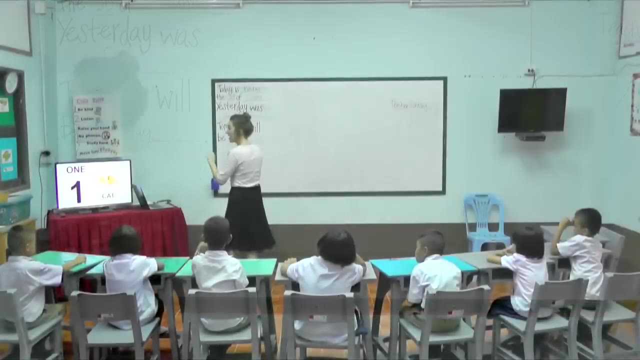 Zero. See how there's nothing for us to count One. What number do we see here? One One, One, One, One, One. So let's count One. Let's count together: One One, One cat. 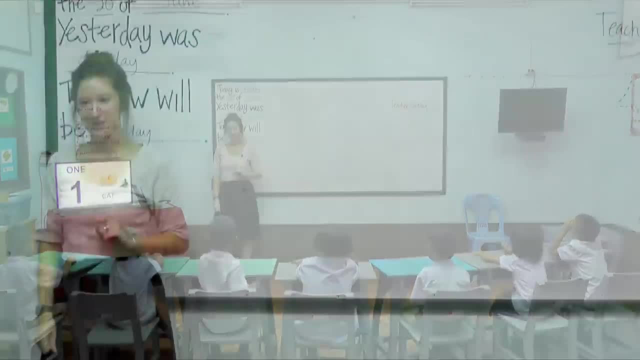 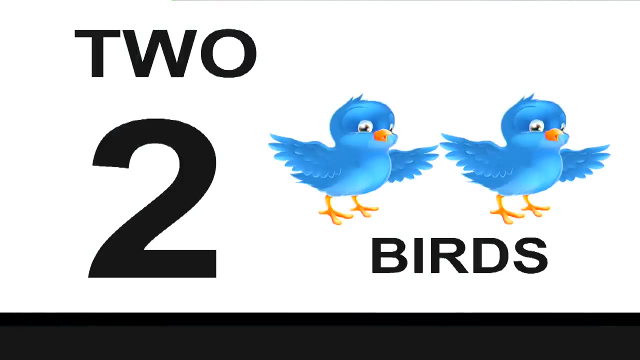 One cat, that's right. There's only one Cat. Very good, One cat. Two, Two, Two, Two, Two, that's right. This is the number Two, Two, Two, Bird, Bird Bird is right. 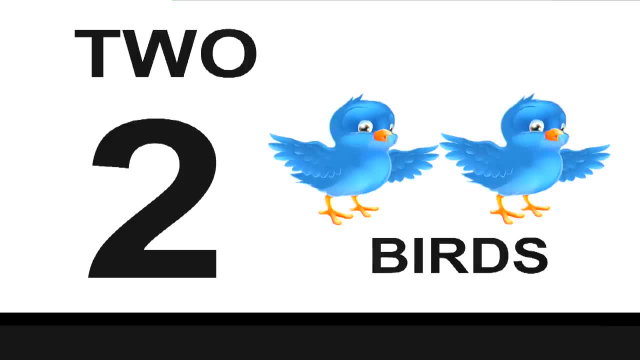 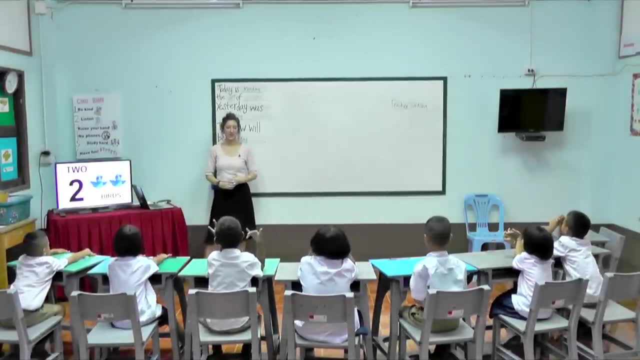 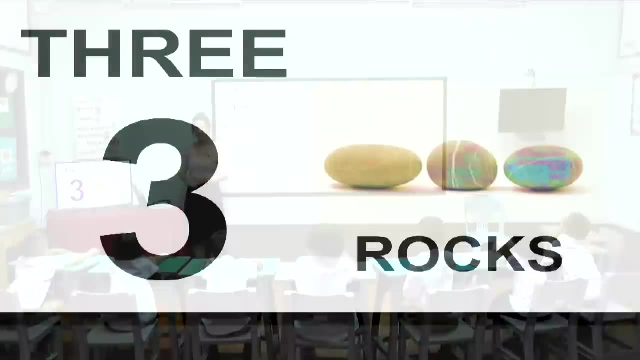 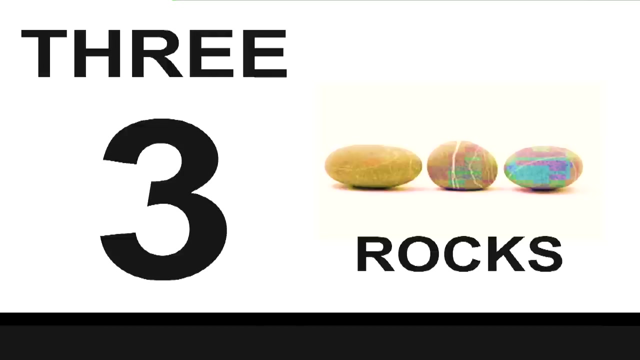 So let's count them: One, One, Two, Two, Two, Two, Two Birds, Birds, Two, Birds, Birds, Birds. Good, Two Birds, What number Three, What number Three, Three? Let me hear you say three. 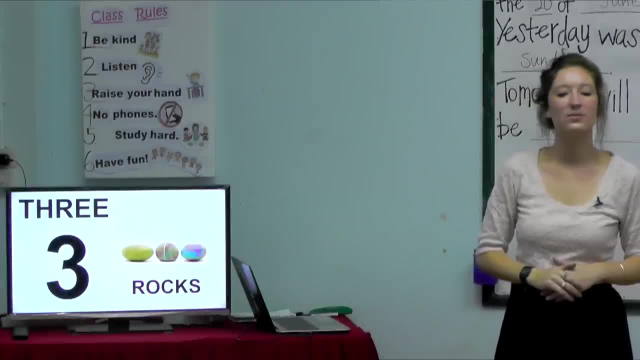 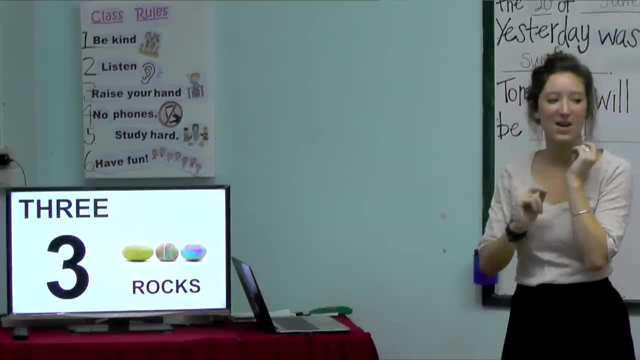 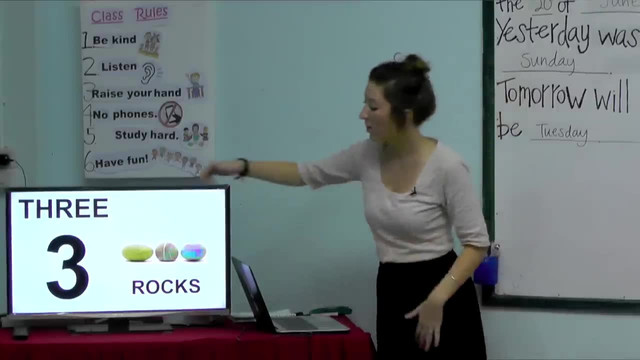 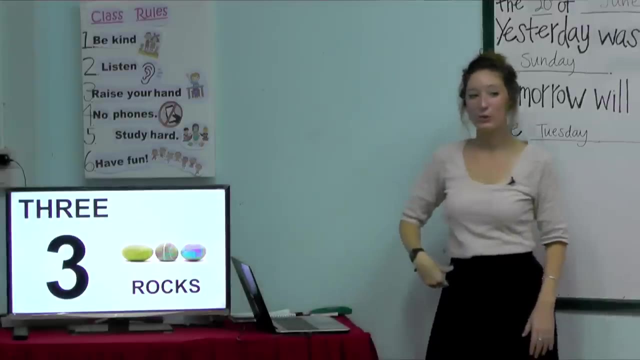 Three, Three, Three, Three. There you go. You kind of have to stick out your tongue. Three, Three, Three, Three. Let's count: Rocks One Rocks, Two Rocks. Three Rocks, Three Rocks. 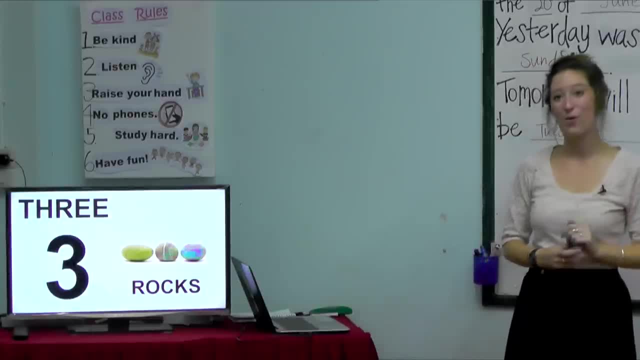 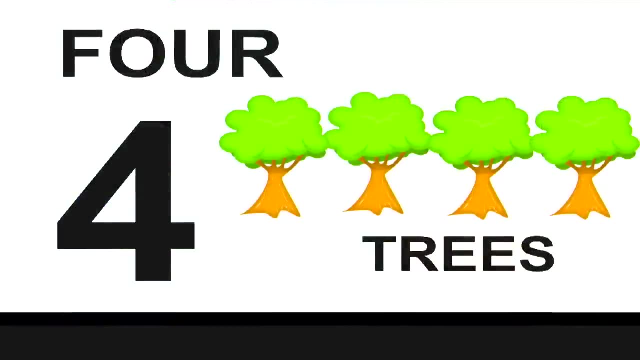 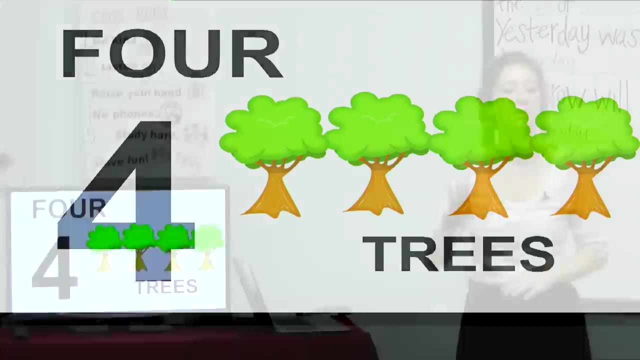 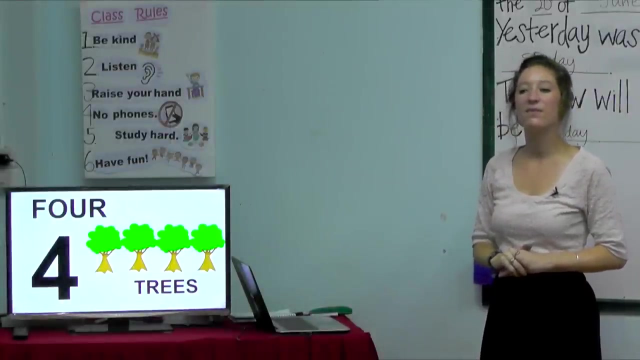 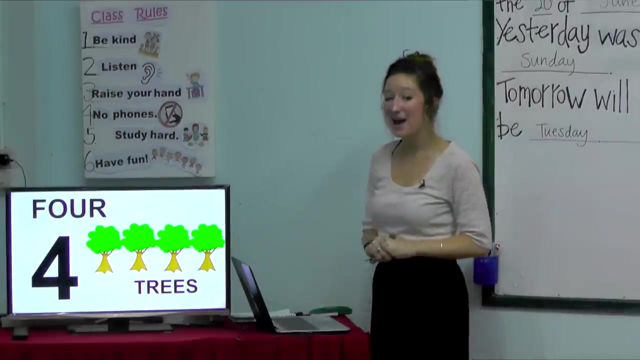 Rocks, Rocks, Rocks, Rocks, That's right. Three rocks, Rocks, Rocks. So what number's next? Four, Four, Four, Four, That's right. this is the number. Four. Rocks, Rocks, four. There you go. F sound at the beginning, Four, Four, Good, So let's count One. 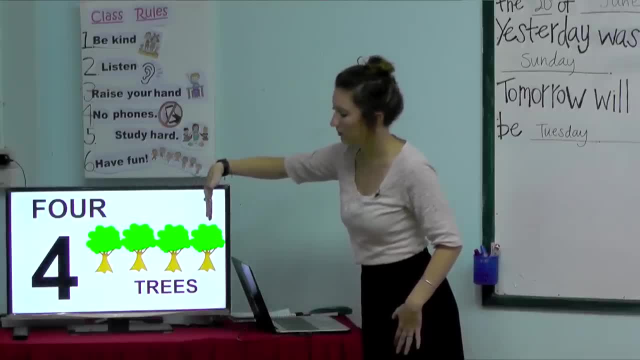 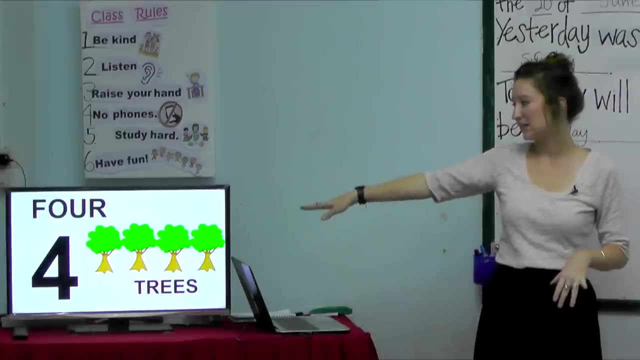 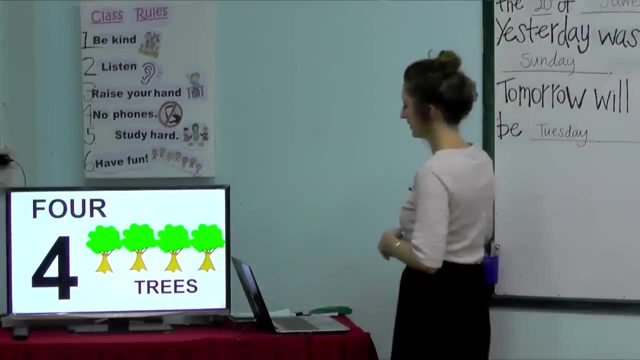 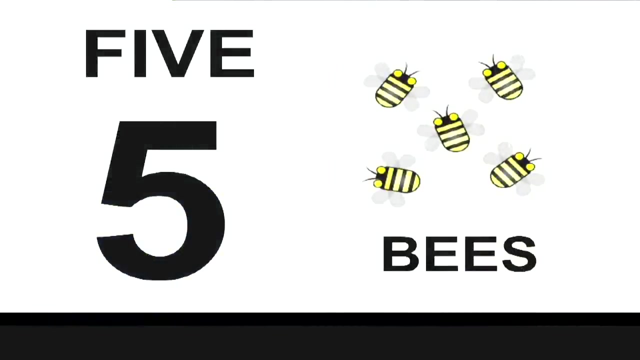 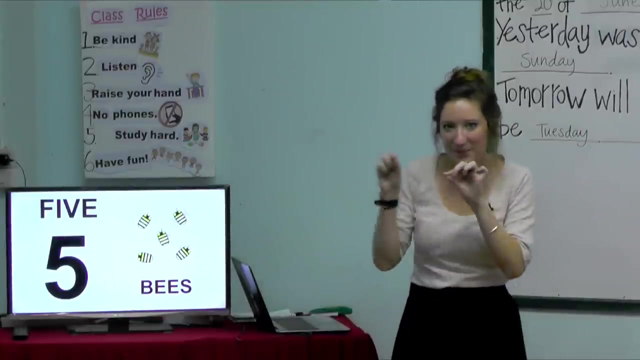 two, three, four, Four, Four trees, Tree, Four trees. Good, What number is this? What number? Five, Five, That is the number five, Five. And what do we call these? Do you remember? Bzzz, Bzzz, Bee, We call these bees, So let's. 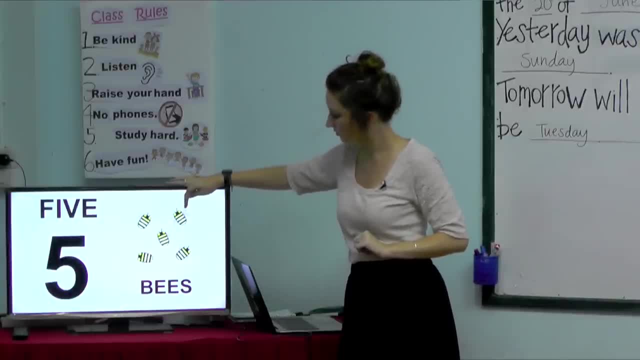 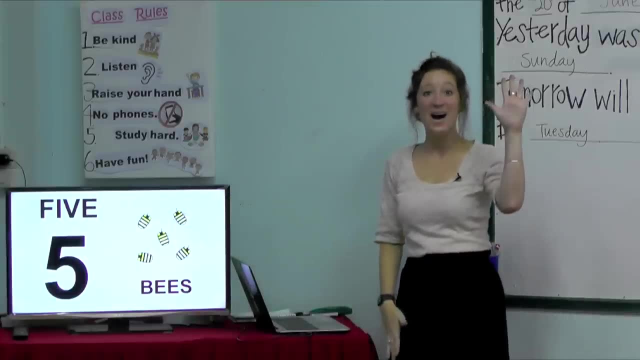 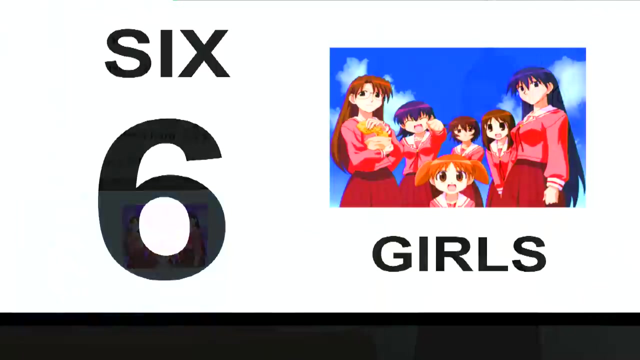 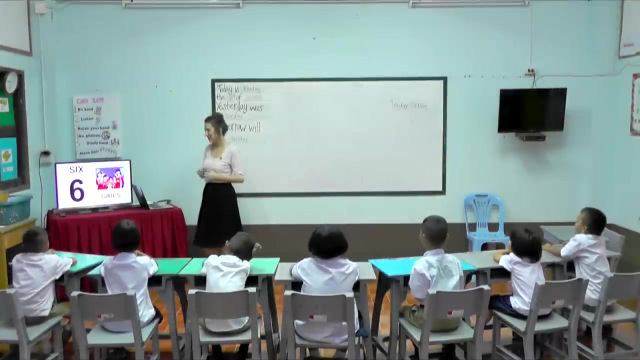 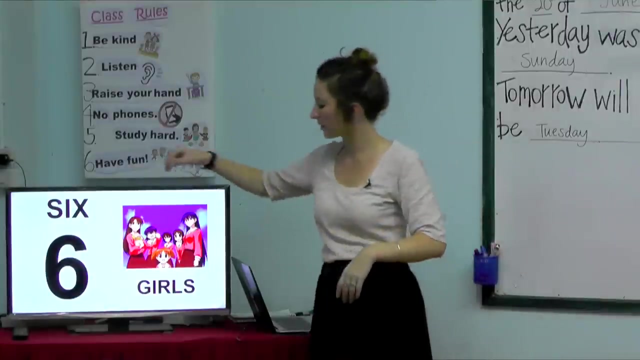 count One, Two, Three, Four, Five. How many? Five, Five, Five, Five bees. What number? Six, Six, That's right, This is the number six, Six, Six, Six, girls, Girls, Yeah, these are girls. Let's count One, Two, Three, Four, Five. 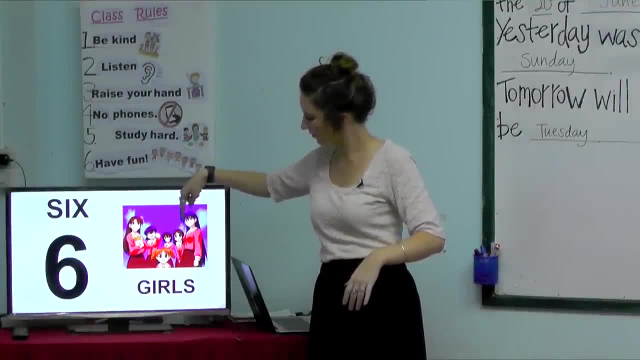 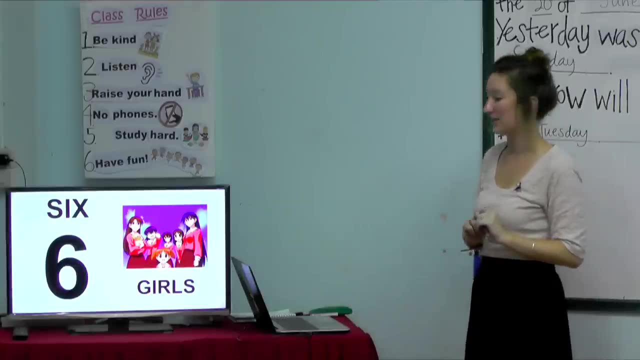 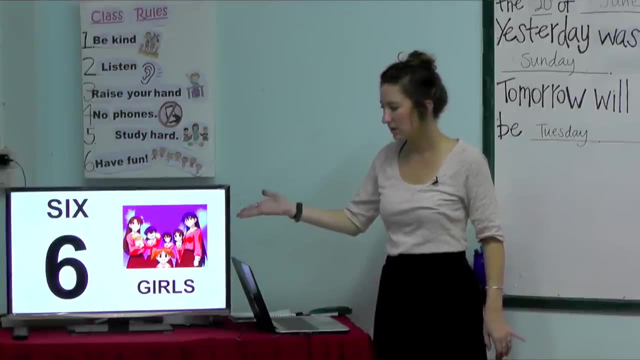 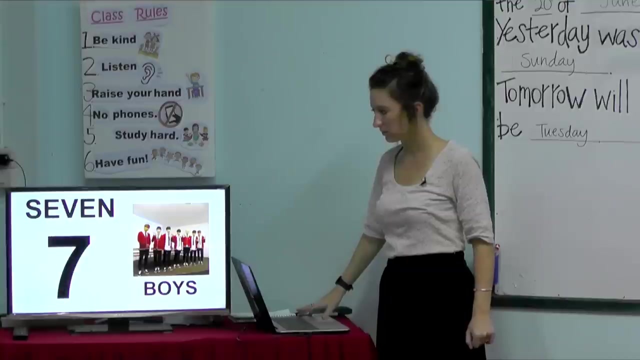 Two, Three, Four, Five, Six. So how many, Six, Six girls, Six girls, How many Two? How many? How many girls? Six, Six, Good job, Seven, Seven, That's right, This is the number seven, Seven, Six girls. 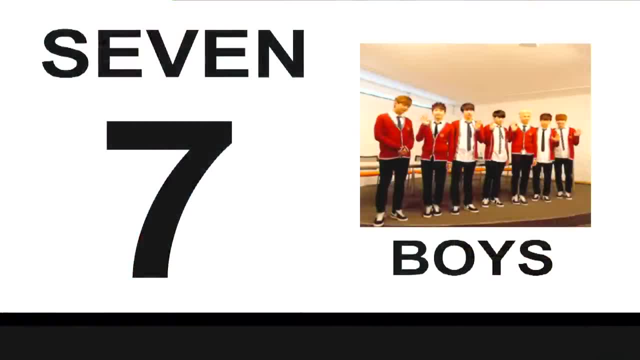 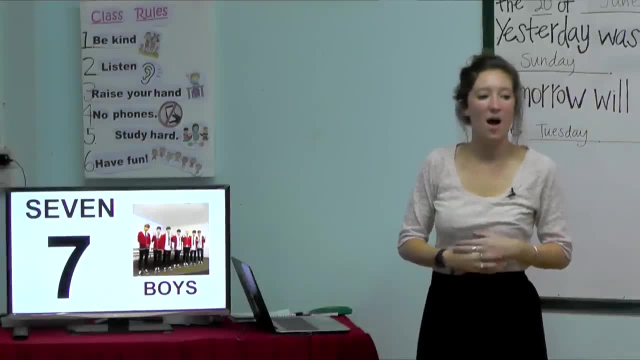 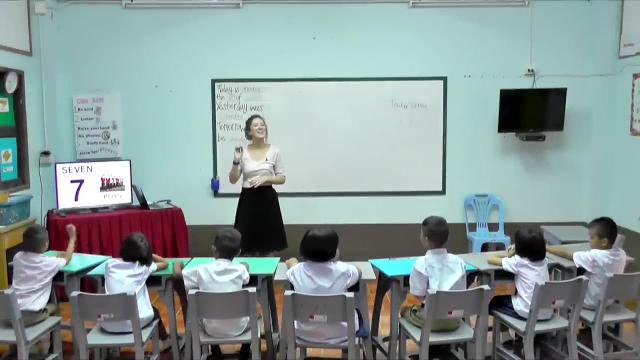 Thanks guys, Thank you so much, Thank you so much. Thank you for joining us here today. Seven, seven, seven. there you go, Pengpeng, let me hear you say seven, Seven, seven, seven, very good. 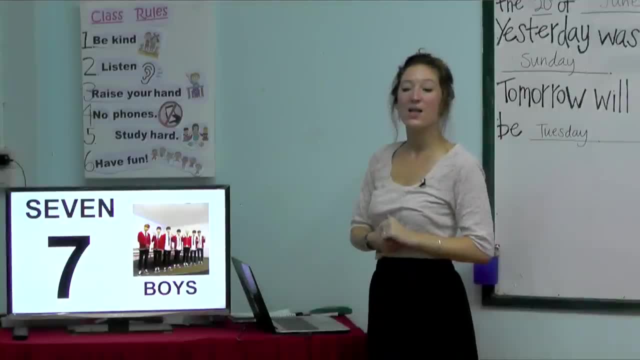 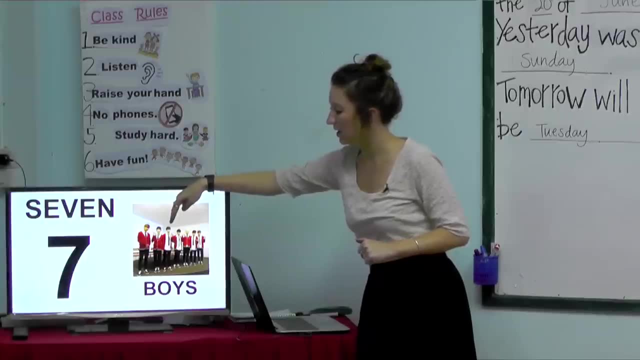 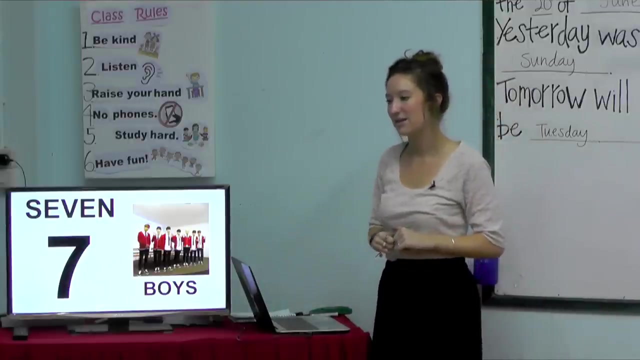 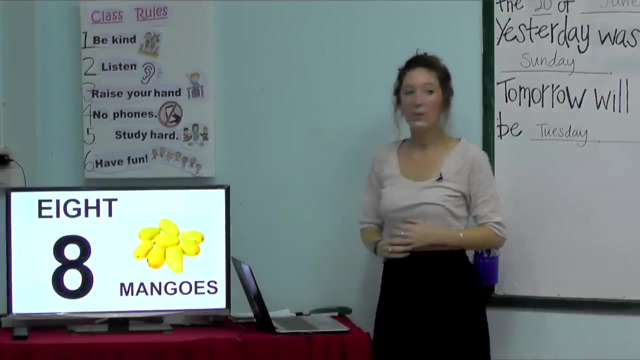 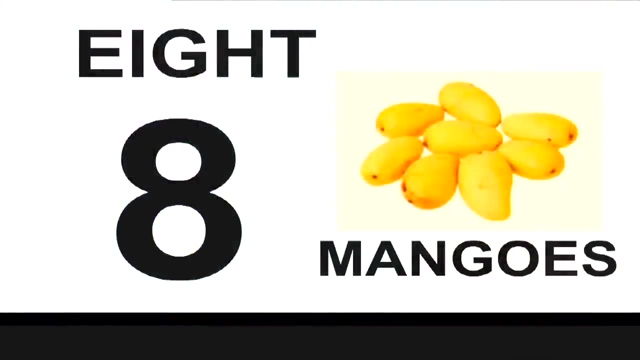 Boys, boys. let's count one, three, four, five, six, four, five, six, seven. how many? Seven, seven, seven boys. that's right, seven, seven boys. What number? Eight? this is the number eight eight. 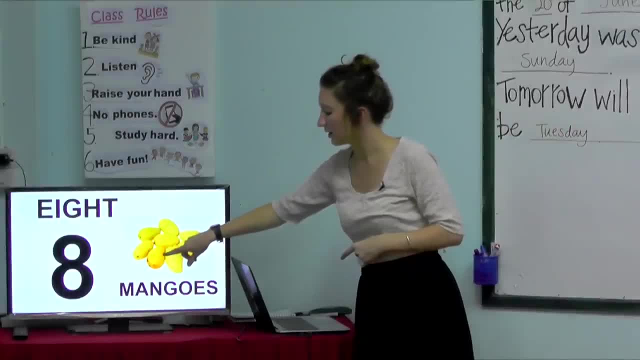 Do we remember what we call these? Wait, wait, wait, wait. mangoes, mangoes, mangoes, great. So let's count. one, three, four, five, six, seven, eight. How many? Eight, eight. 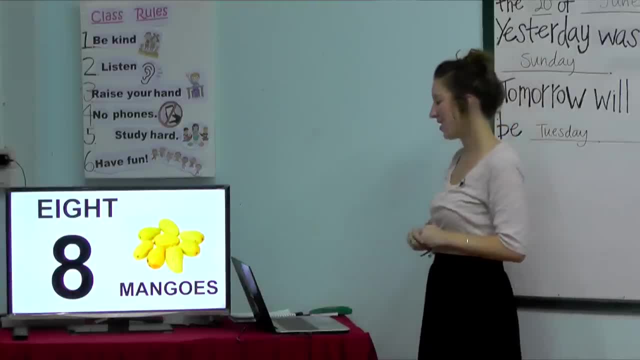 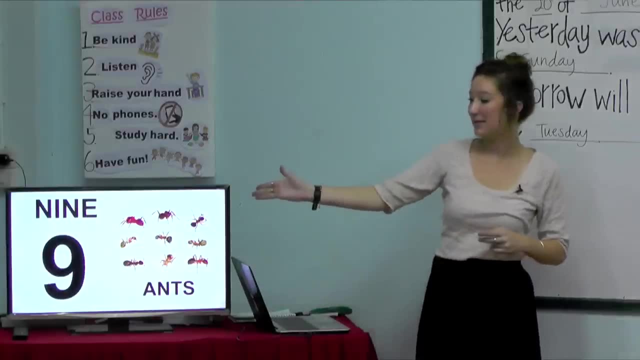 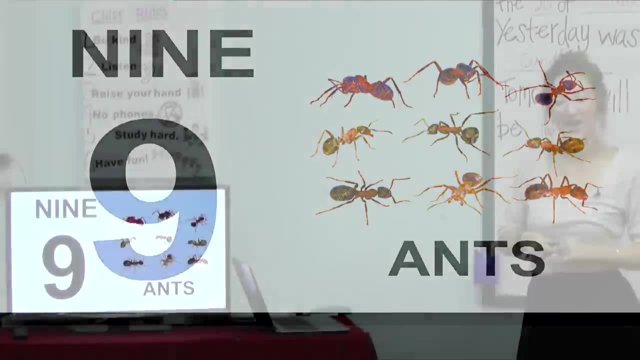 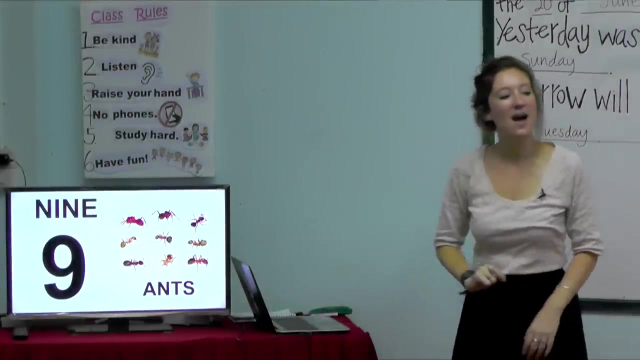 Eight mangoes, Mangoes. Yeah, there's eight Mango, mango nine. What number? what number is this? Does anybody know what number? It's the number nine. Let me hear you say nine, Nine, Nine, Nine. 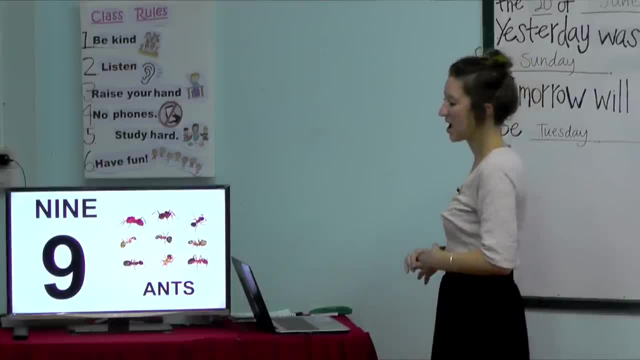 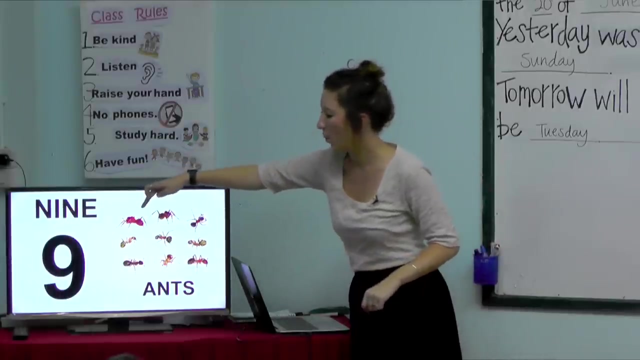 Very good. nine, Nine, Nine, Nine. These are ants, Ouch, Ouch Ants, Ouch Ants. So let's count: One, two, three, four, five, six, seven, eight, nine. 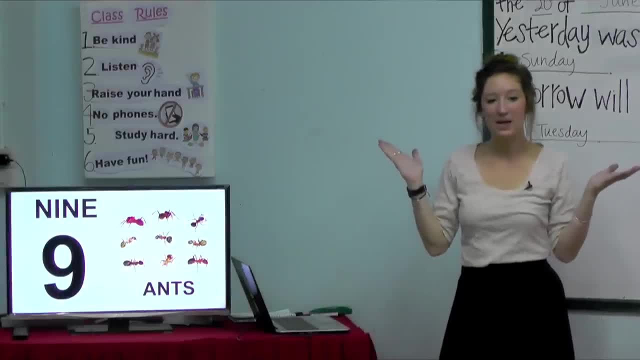 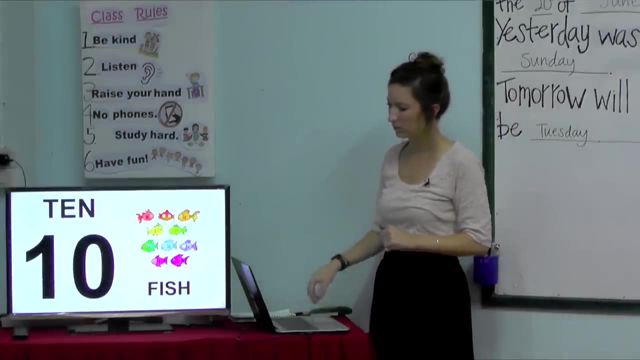 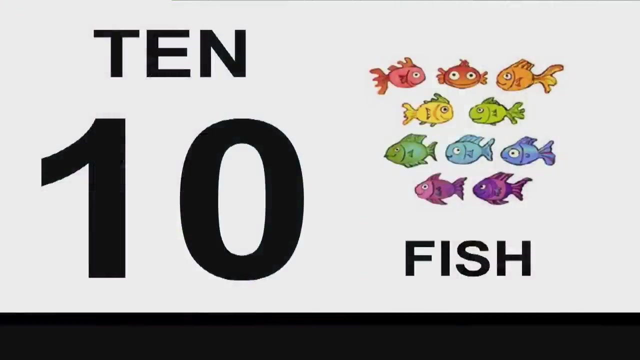 Ten. How many? Ten And ten, Nine, Nine, Nine ants. How many? Nine, Nine, Nine ants? There's nine ants. Uh-oh, What number. Ten, This is the number ten, Ten, Ten. 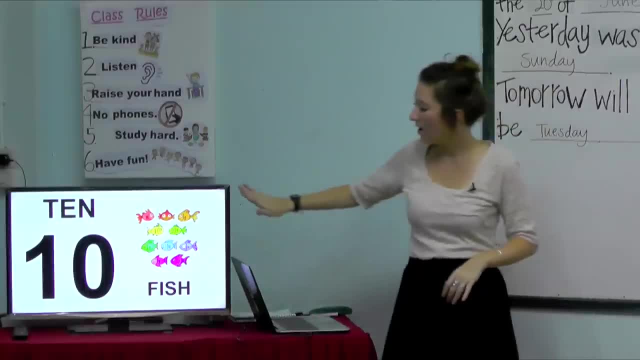 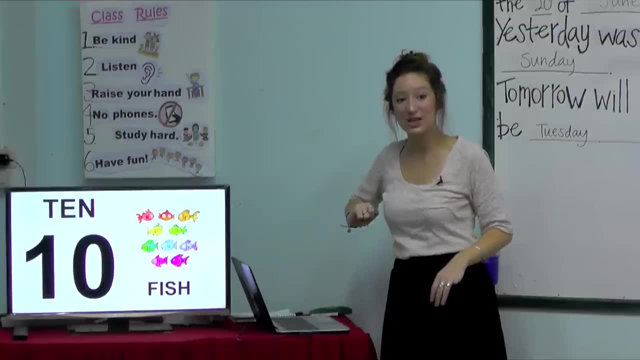 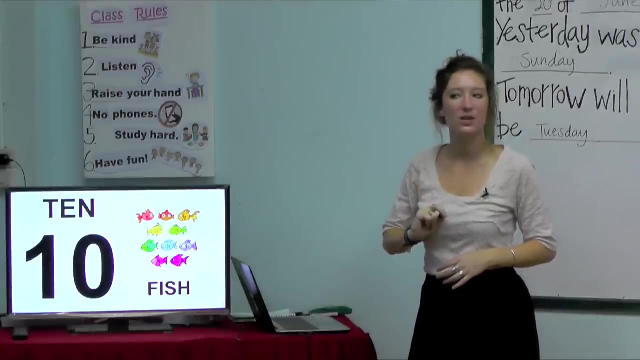 This is the number ten. What do we call these? Do we remember Fish, Fish, Fish Fish? Yeah, these are fish, Fish, Fish, Fish. Let me hear you say ten, Ten, Ten Fish Fish. 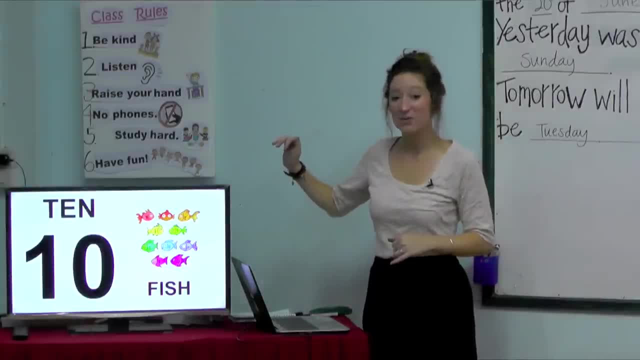 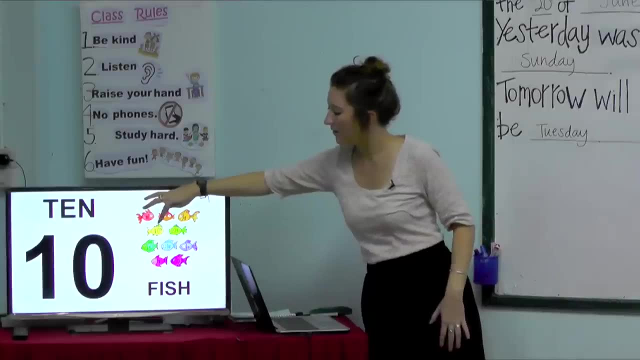 Fish, Fish, Fish, Great, Let's count. One. One, One, Two, Two, Three, Three, Four, Four, Five, Five, Six, Six, Seven, Eight, Nine, Ten, That's right Ten. 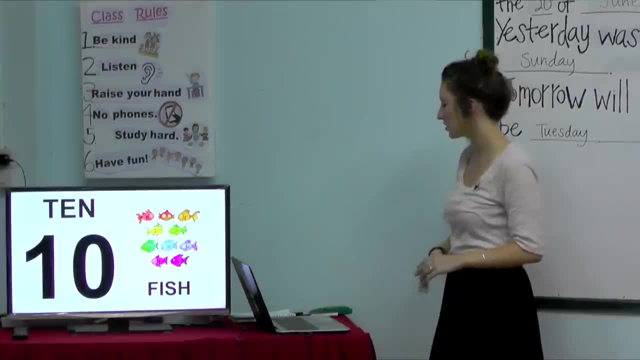 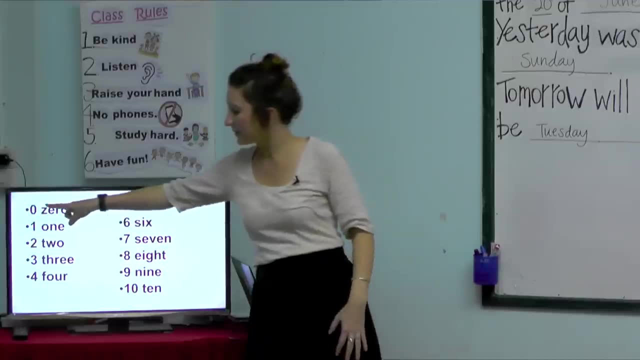 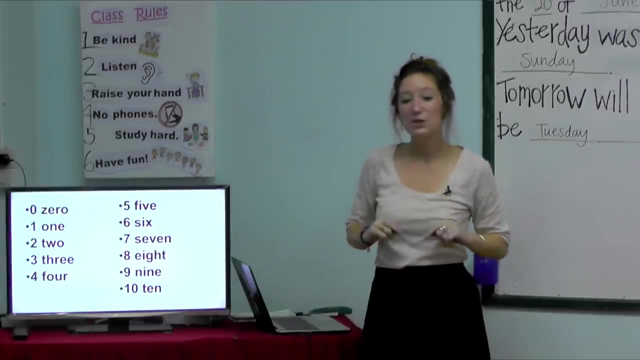 Ten fish, Ten, Ten fish, Ten fish, Ten fish. So let's go over them together. Zero, Zero, Zero, Zero. One, One, Two, Two, Wait for me. Two, Two, Three, Three, Four. 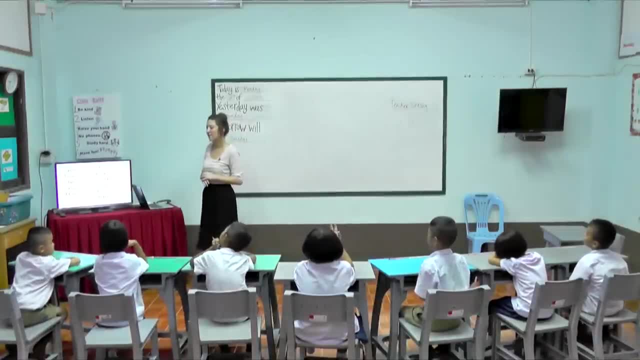 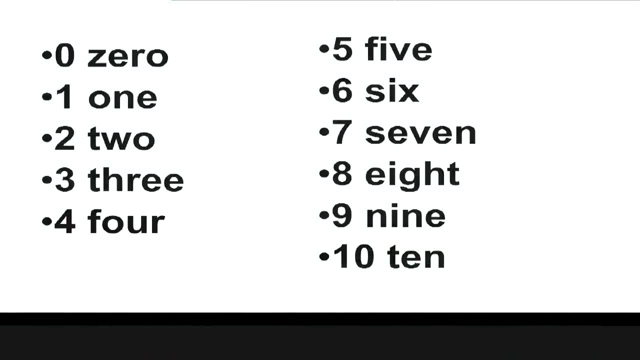 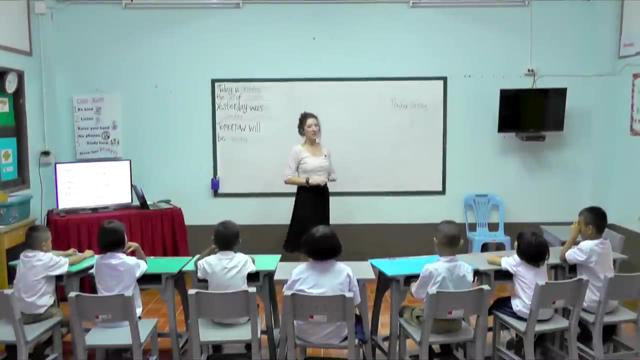 Four, Four, Five, Five, Five, Five, Six, Six, Seven, Seven, Seven, Eight, Eight, Nine, Nine, Ten, Ten, Ten, Great job. Now I want you guys to practice counting with us with a song. 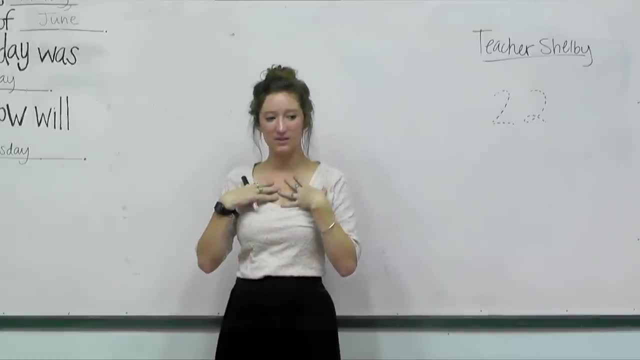 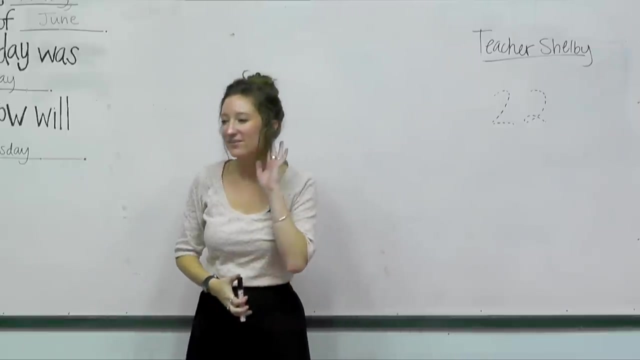 With a song. So first I will sing and then you repeat after me. We'll try it. One, two, three, four. One, two, three, four, Five and six, Five and six, Seven, eight, nine and ten. 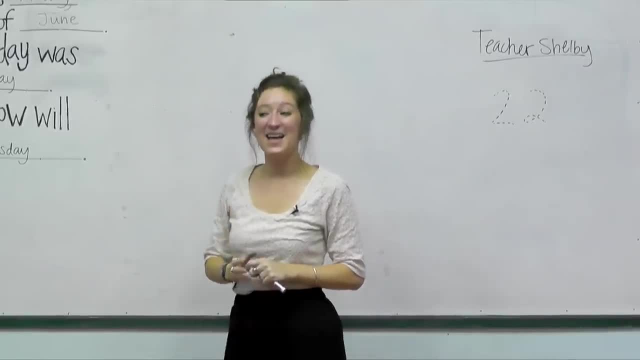 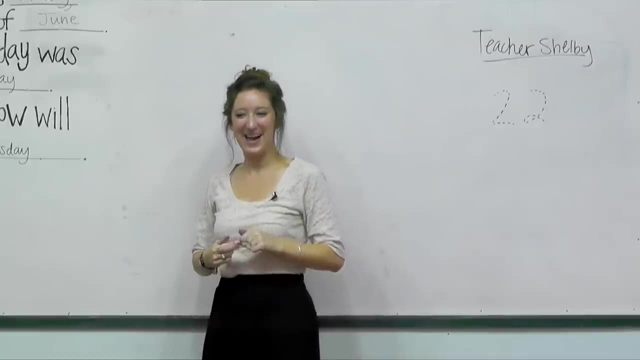 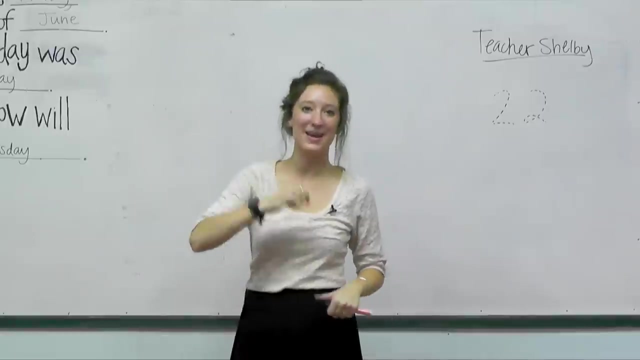 Seven, eight, nine and ten. Let's begin. Let's begin Very good. I know the seven, eight, nine and ten. It can be a little tricky. You did a great job. We're going to do it again. 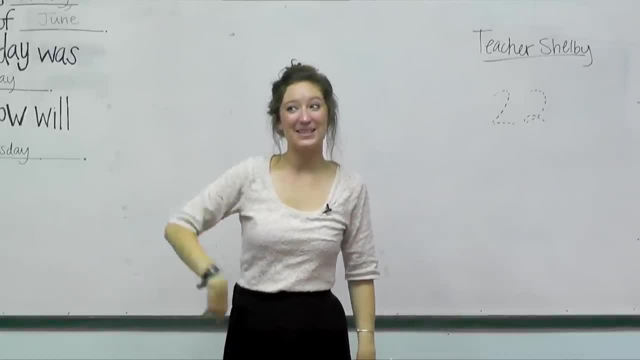 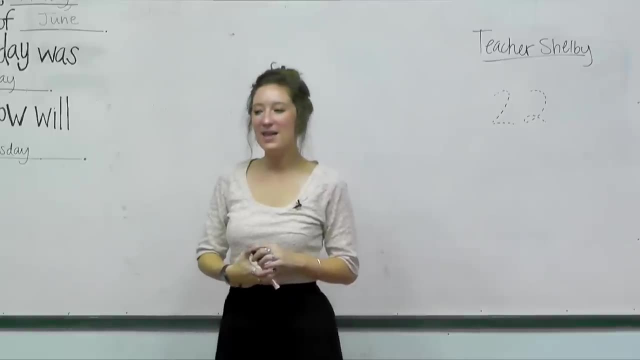 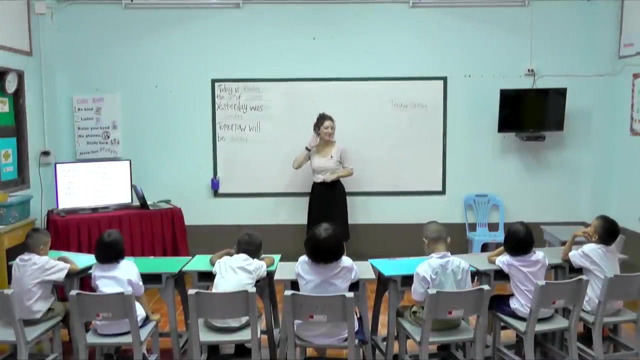 So listen up and sing along with us. One, two, three, four. One, two, three, four, Five and six, Five and six, Seven, eight, nine and ten. Seven, eight, nine and ten. 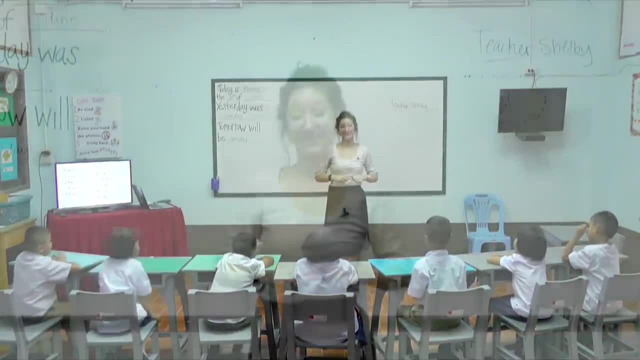 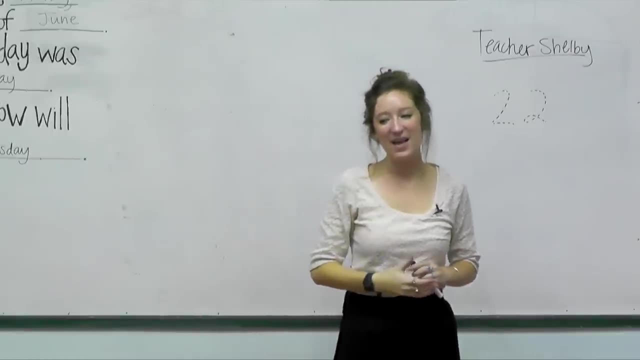 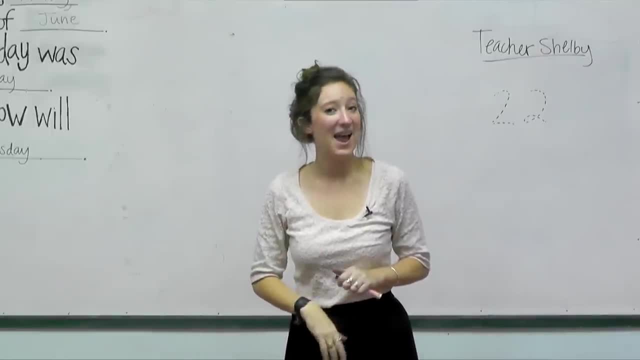 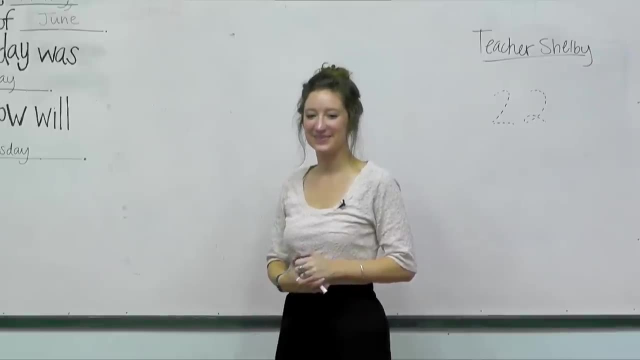 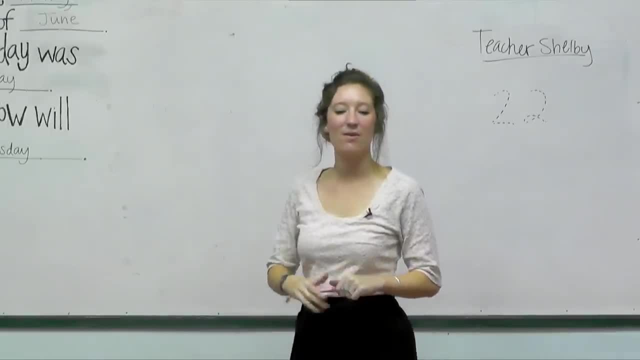 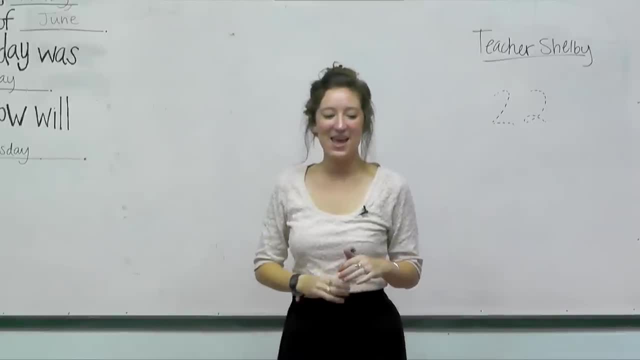 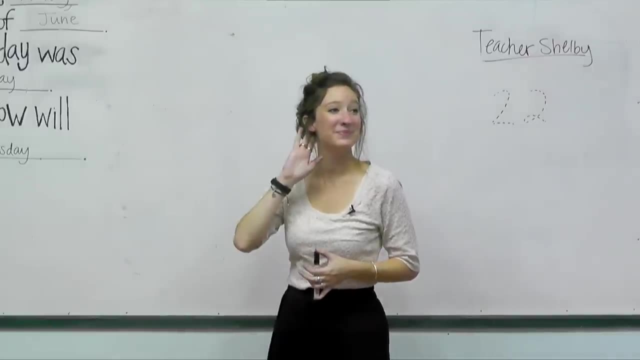 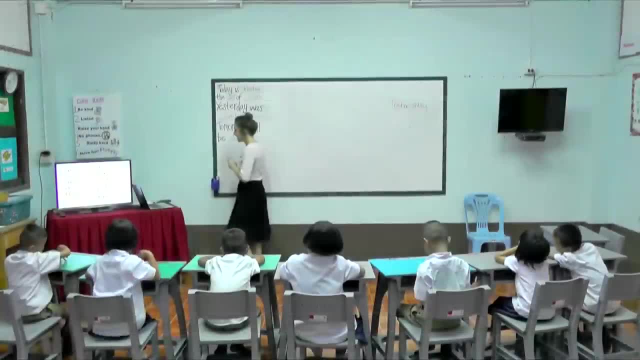 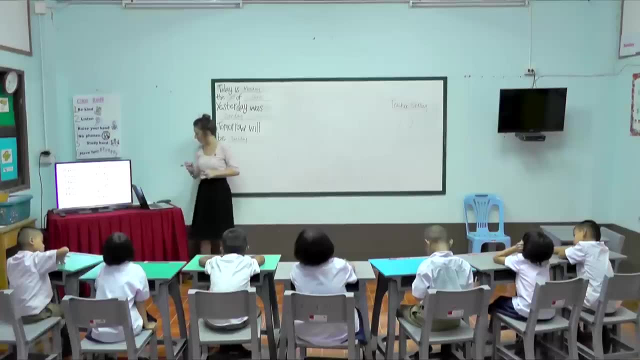 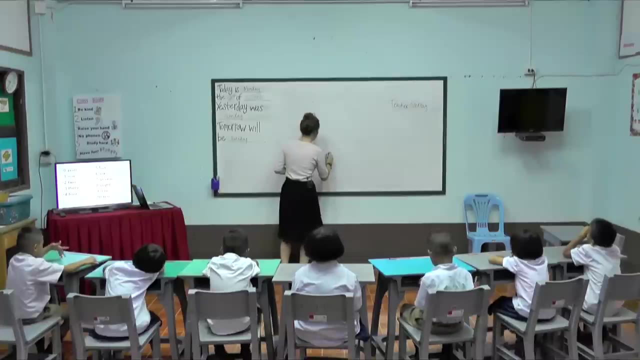 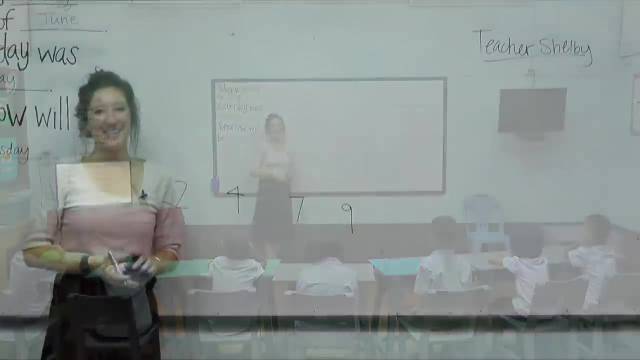 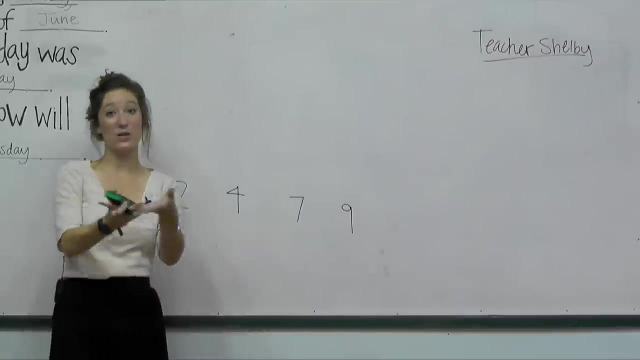 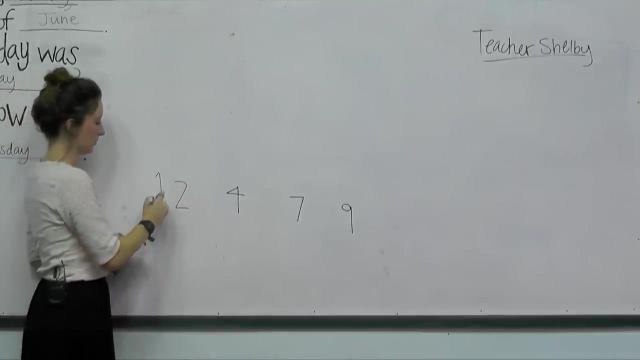 Great job, everybody. Okay, so now I want you all to play fill in the blank with me. Here we go. Okay, great. So for our last activity for today, I'm just going to board some numbers up here and I want you all to help me fill in the blank. Okay, So what number is this? 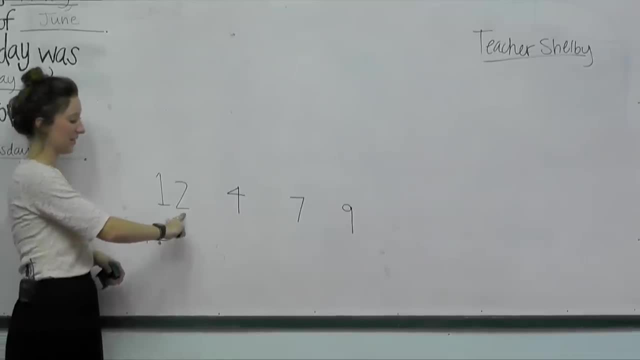 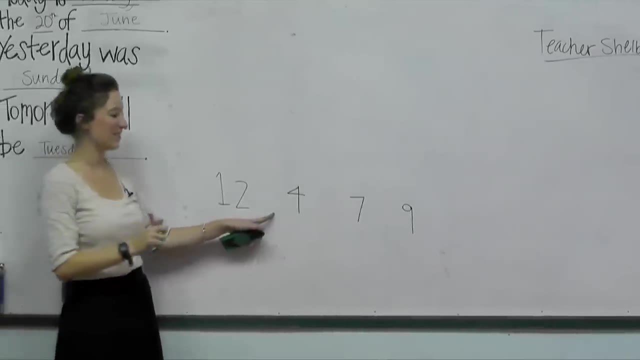 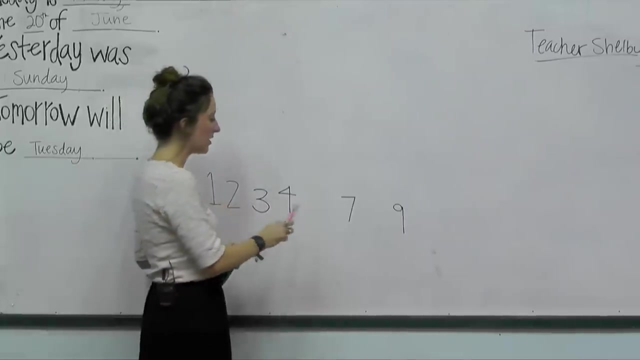 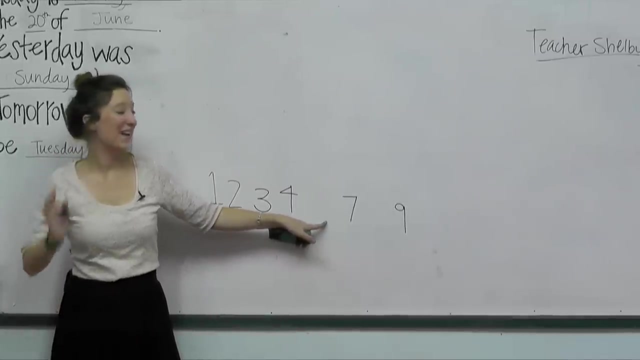 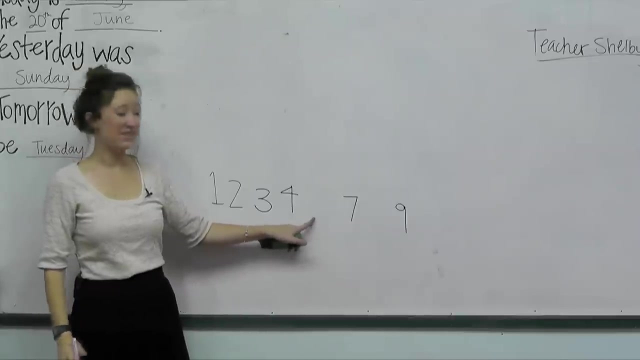 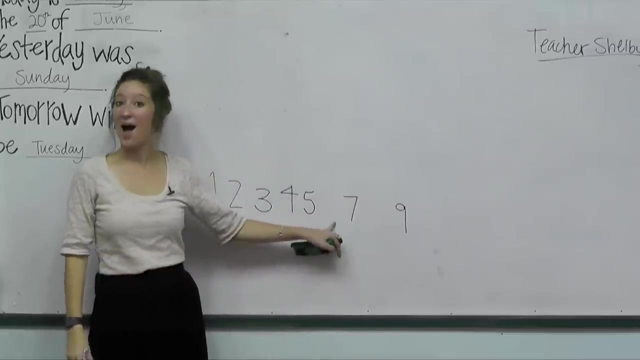 What number? One, One, Two, Three, Three, So three is missing. I'll write it in: this time. We're missing a three. Good, So let's go here. What number Five, Five, Five. We have one, Two, Three, Four, Five, Five is missing. So what's missing here? Six, Six. 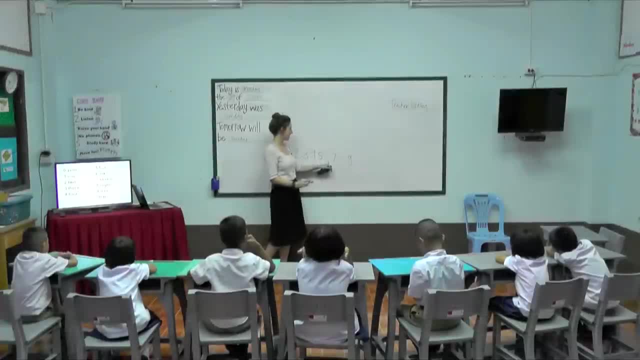 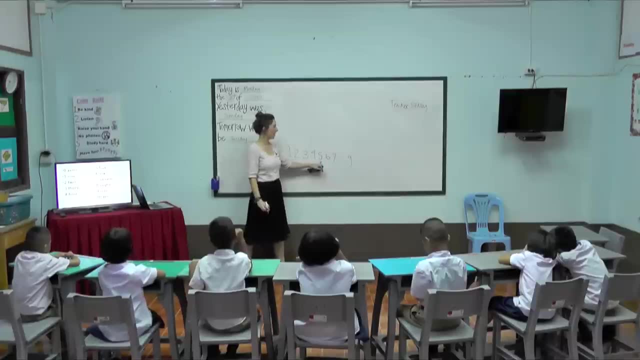 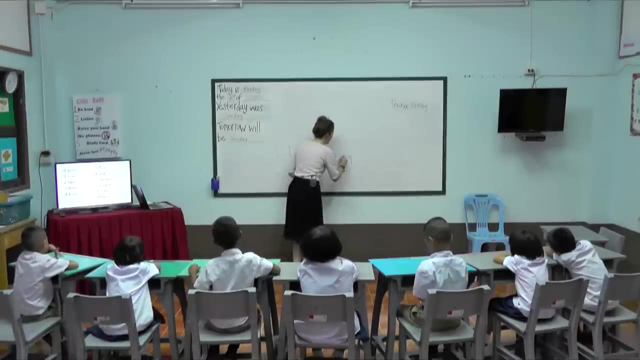 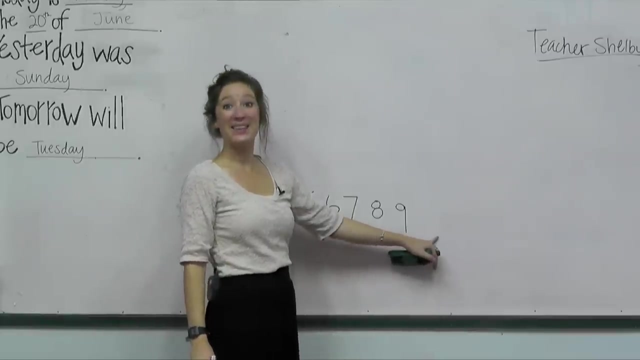 Six, Six, very good. A six is missing here. One, two, three, four, five, six, seven, Eight, Eight, that's right. An eight is missing here. And what's after? an eight, Nine, That's right. our last missing number is a 10.. 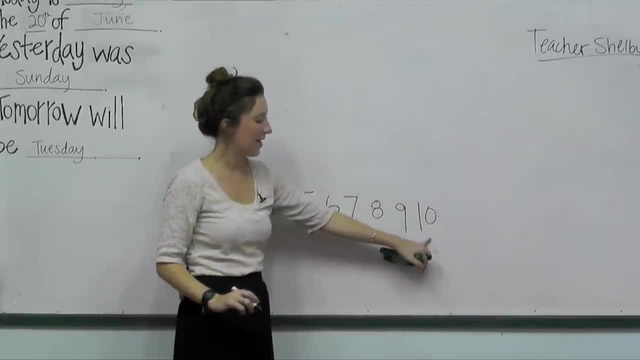 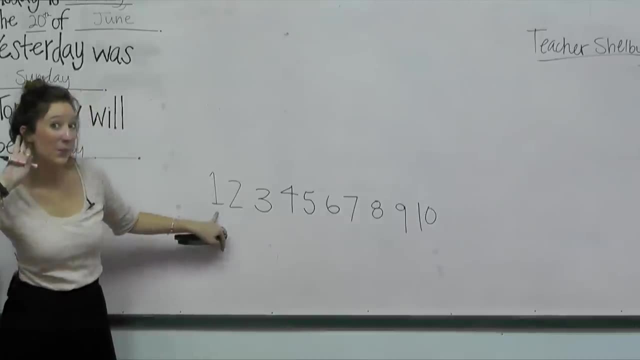 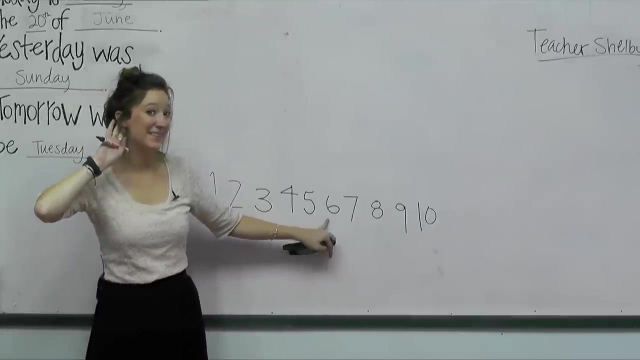 10. One, two, three, four, five, six, seven, eight, nine, 10.. So let me hear you guys say it, without my help: Ready: One, two, three, four, five, six, seven, eight, nine, 10..